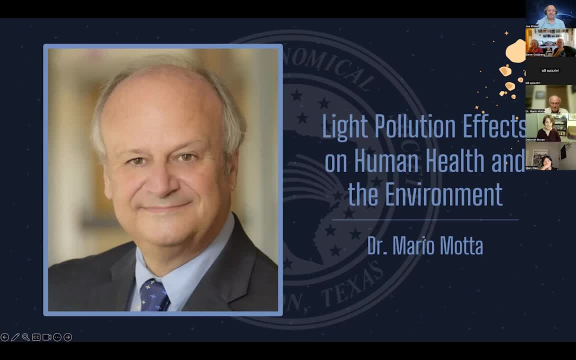 telescopes and observatories throughout the years to do astronomy research, including his entirely homemade 32-inch F6 relay telescope located in Gloucester, Massachusetts. He's been awarded several national awards in astronomy, including the Las Cumbres Award from the Astronomical Society of the Pacific in 2003,, and also the Walter Scott Houston Award from the. 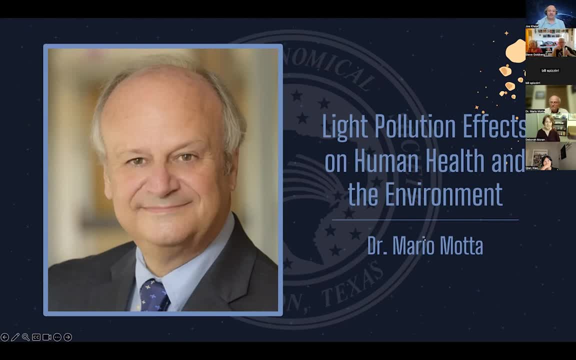 Northeast Section of the Astronomical League And in 2017, the Henry Algar Alcott Award from the American Association of Variable Star Observers. He's also served as president of the ATMs of Boston and has served as a council member of the AAVSO and is a past. 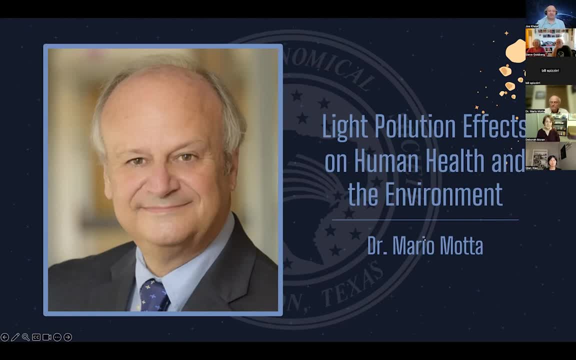 president as well. Finally, several years ago, the International Astronomical Union awarded Dr Mata an asteroid, in part for his work on light pollution, as well as amateur research: asteroid 133537 Mario Mata. So, without further ado, it's my pleasure to introduce Dr Mata. 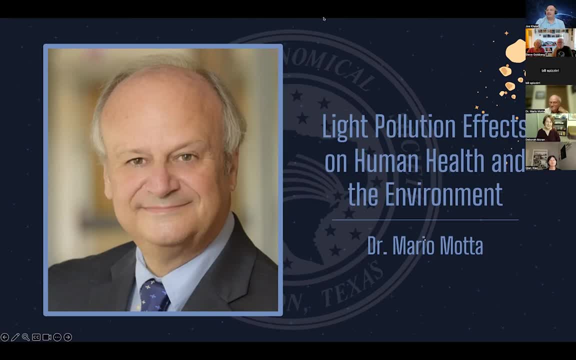 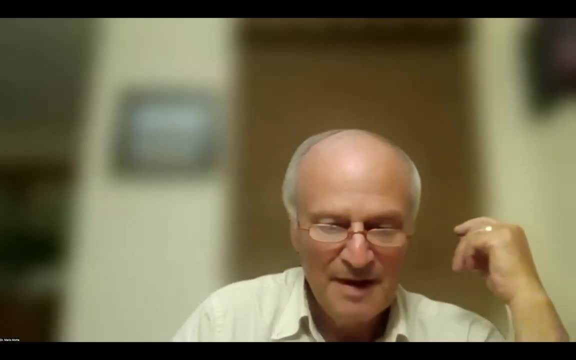 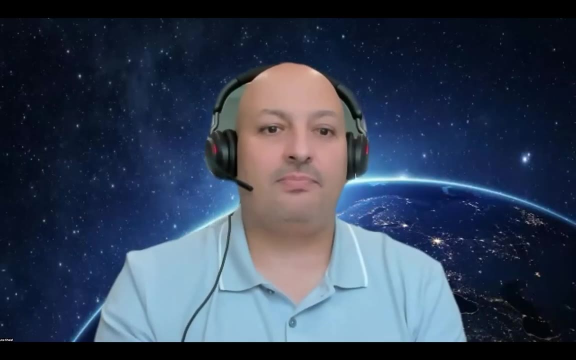 Dr Mata, thank you so much for joining us tonight. I'll stop. I'll stop my share here and I will present the podium to you. All right, That was quite an introduction, Thank you. I will share now, Please, please do. And while you're doing that, I just wanted to remind everybody. 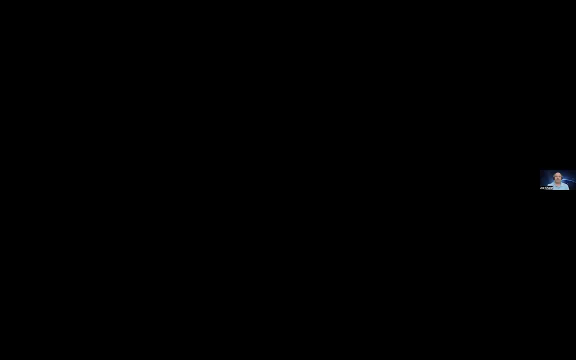 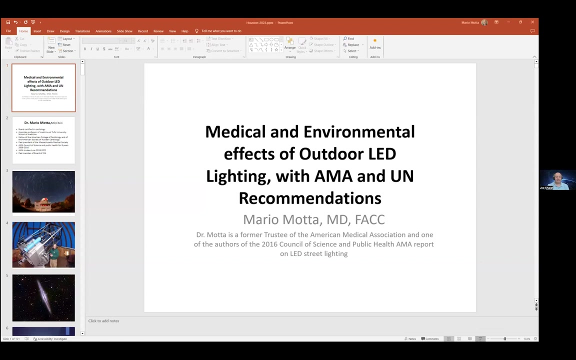 please keep yourselves on mute. We will have Q&A coming in through the chat feature that we have in Zoom. So if you have a question for Dr Mata at the end of the presentation, ask that question through the chat feature. We'll get to those questions in the order that they're. 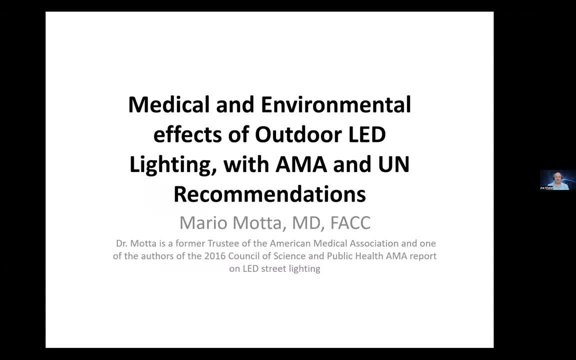 answered, I'll give you all an opportunity to come off of mute and ask the questions there. So thank you. All right, So you can see my screen. We can indeed. Okay, great, So I'll talk about light pollution and its effects on human health, the environment and glare issues. 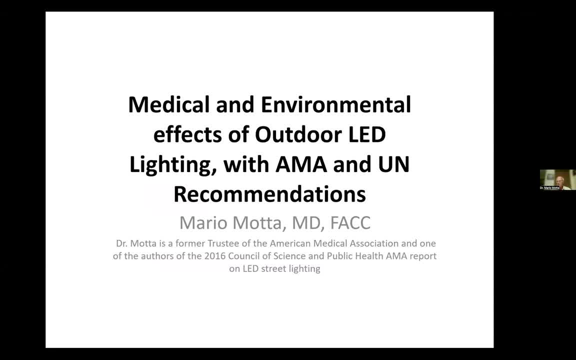 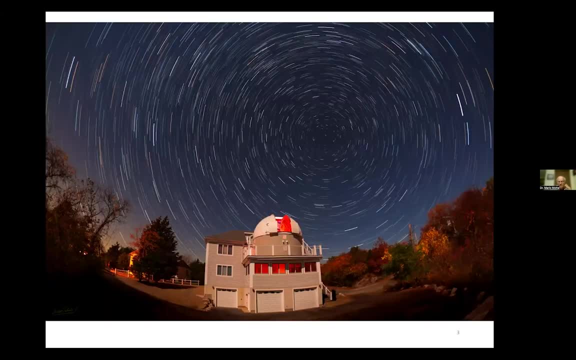 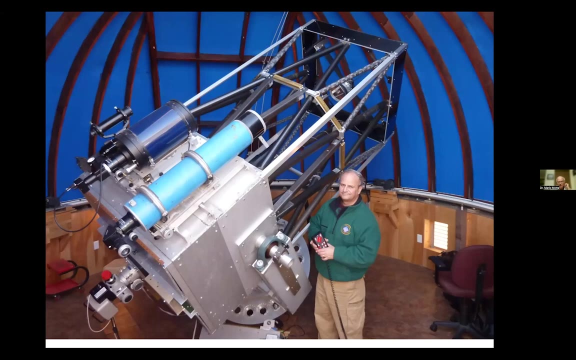 and the AMA's recommendations, as well as the UN recommendations that on a committee I was involved as well, So you already went through this. I won't leave that up. This is my home observatory. It's a 20-foot dome, all handmade. And here's my scope: It's a 32-inch F6.5.. 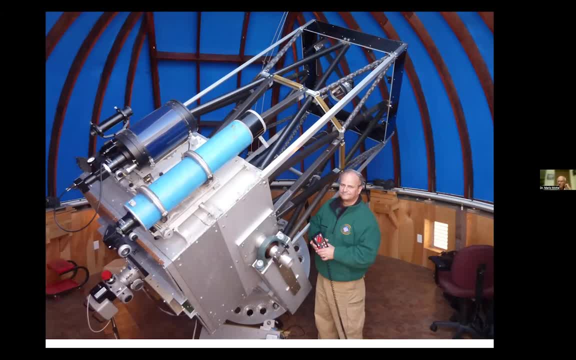 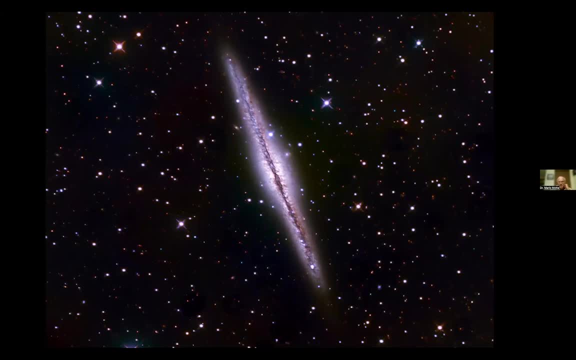 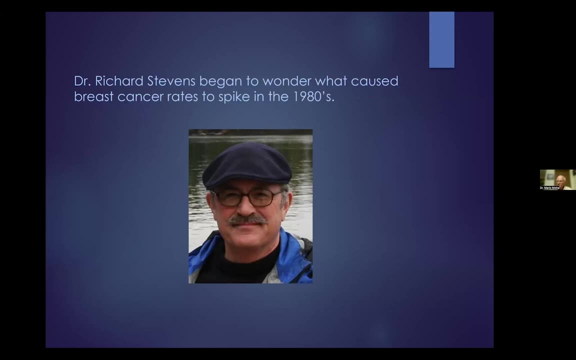 And I use it quite a bit. I was up till 2.30 this morning, in fact. Here's an image of NGC 891 that I've taken. So that's why I'm interested in light pollution. Initially it was because I wanted to protect my 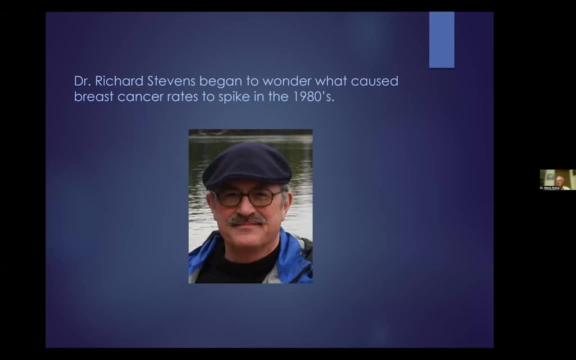 sky for my observatories and my imaging. But I was a researcher early in life And I got interested in the work of this man, Dr Richard Stevens, who was the first person. he was an epidemiologist at the University of Connecticut And he first brought up the issue of whether light pollution 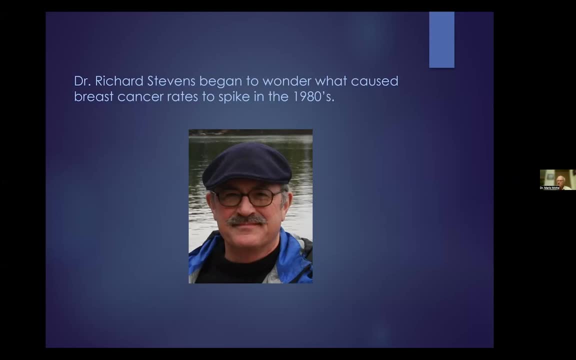 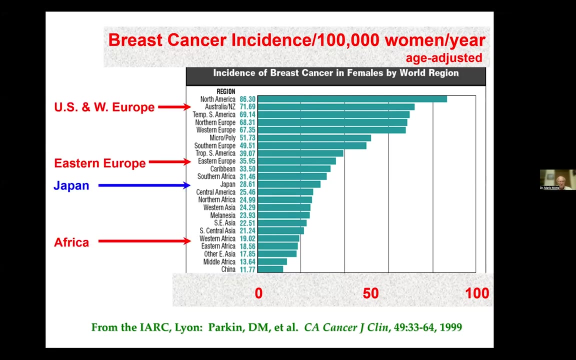 suppressing melatonin could be a reason for the increase in breast cancer in the Western world. And here is the thing that piqued his interest. So, if can you see my arrow pointer right? Okay, So at that time this is early 19,, from 1999, this slide, but it was the same in 1990,. 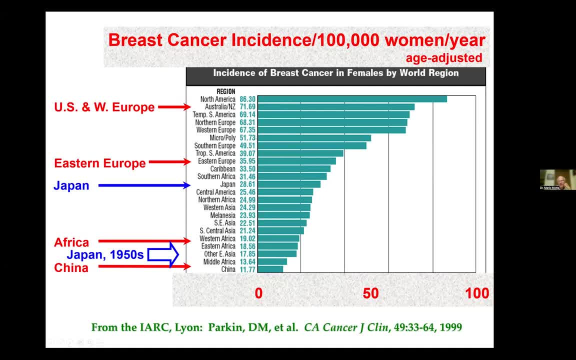 when we first met He noticed that in North America the rate of breast cancer is quite high. In China it was quite low. Immigrants from China to the US rapidly reached the same level of breast cancer as North America And he reasoned it couldn't be air pollution or 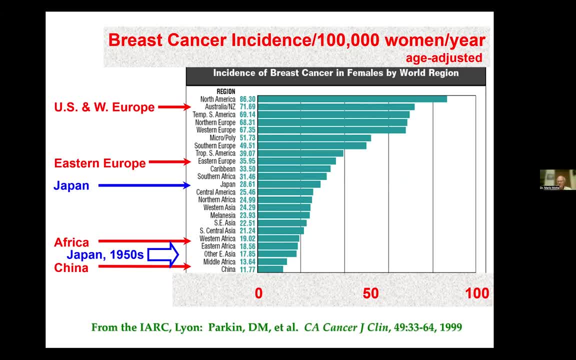 general toxins in the environment, because China at the time was far more polluted than the United States. So he looked for other reasons And and then looking at multiple countries, the one thing that came clear is the greater the amount of light pollution, the greater the amount of breast cancer. 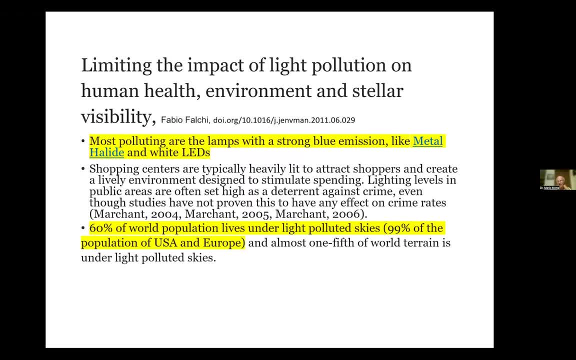 which was a startling conclusion. Now, at the time it was just a hypothesis, But since that time, many, many studies have proven him correct. Till now, I don't think it's in any question at all. So numerous people have worked on this. 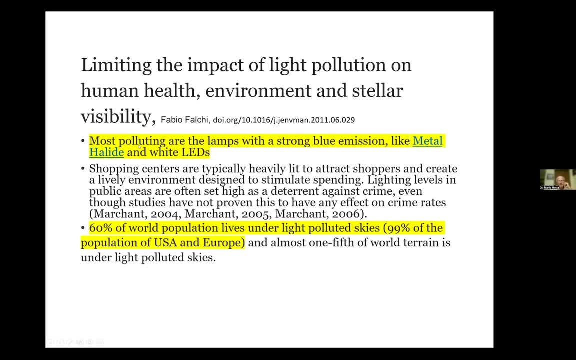 Here's a paper by Fauci, Fabio Fauci, who's showing that lamps with strong blue emission and white LEDs typically cause the most problem, And 60% of the world population currently nowadays lives under light-polluted skies, So this is a worldwide problem, much greater, of course. 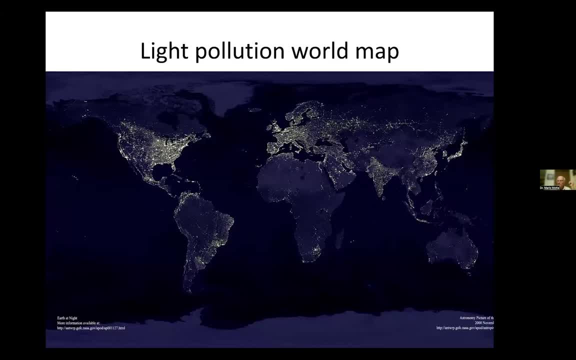 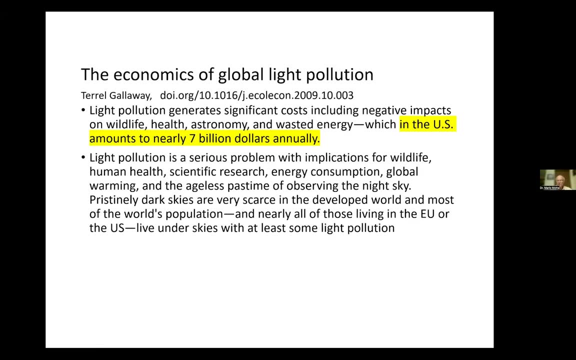 in the Western world. I don't have to tell this group, but this is what light pollution looks like from a satellite. The economics of global light pollution are quite startling. We waste $7 billion annually, and that's from 2009.. That was 10 years ago. It's much greater now. 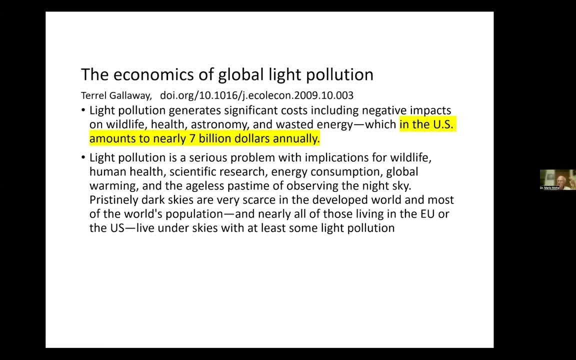 And that's just the light that we let escape, not the amount that we spend on electricity for lights on the ground. The obvious: All this can be captured and we wouldn't have to waste so much if we just directed the light down and not allow it to go up into space, showing up in satellites like the last picture. I thought. 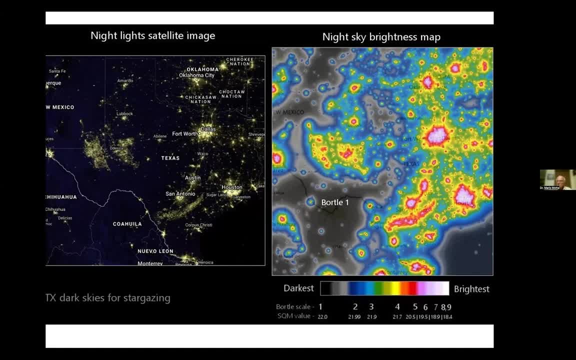 I'd include a satellite photo of Texas, since that's the crowd I'm speaking to. Houston, unfortunately, I hate to say, is one of the most light-polluted areas in the whole universe. Dallas isn't far behind Out here. this is mostly burn-off from methane, But you've got your share of light pollution in. 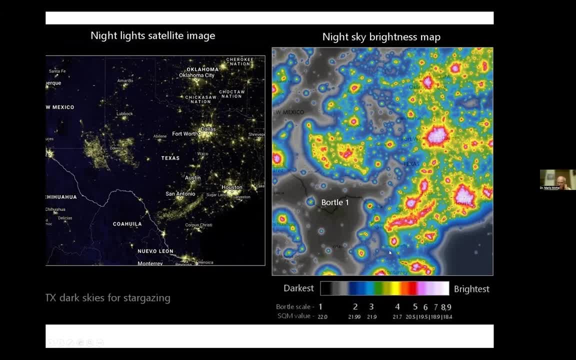 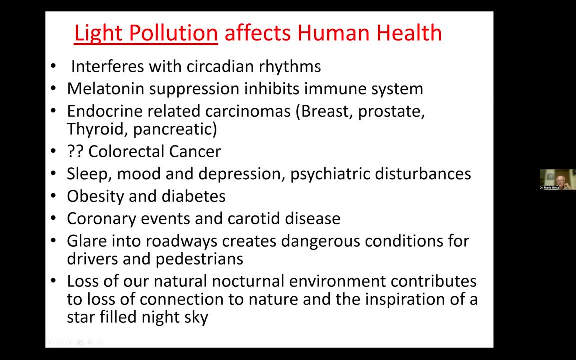 Texas and you have to go out pretty far now to be able to see a good dark sky. So light pollution affects human health. It interferes with circadian rhythms. That's unquestioned now. In fact, the UN declared light pollution a carcinogen as far back as 2009,. 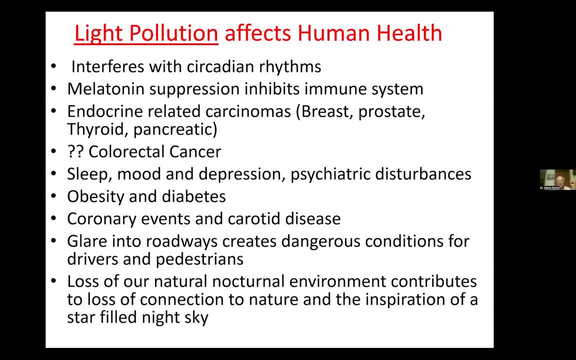 based on studies in the 2000s. Melatonin suppression inhibits the immune system because melatonin is an adjunct to the immune system, So there are many endocrine-related carcinomas because of that. It's been proven in breast, prostate, thyroid and pancreatic cancers. Now colorectal cancer is still. 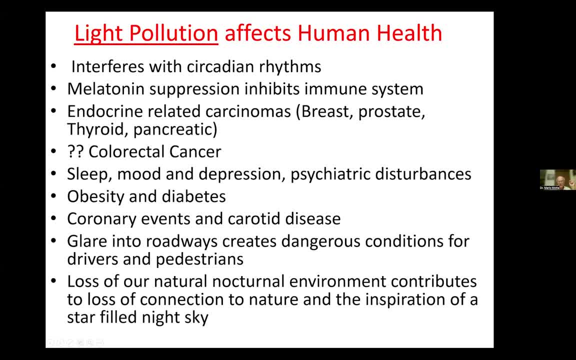 questionable, but there are hints that it may be affecting that as well. So there's because it's not so surprising that it affects sleep, mood and depression. Obesity increases with light pollution and it's consequent diabetes, an increase in coronary events, So there's a wide range of human health effects. Then you have 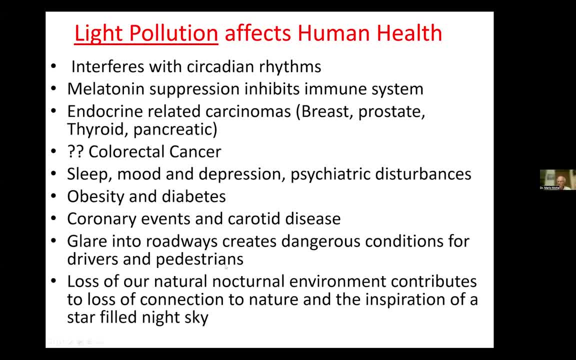 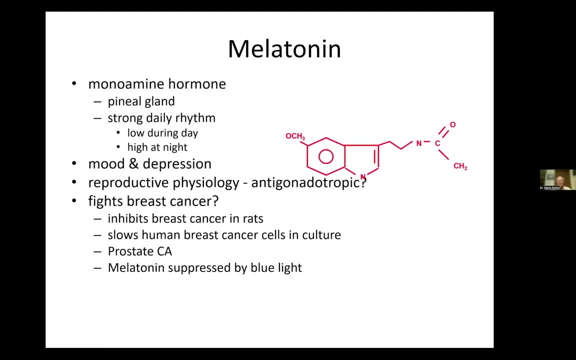 glare into the roadways, that creates dangerous conditions for drivers and pedestrians, And then we have the loss of our natural environment, which contributes to a loss of connection to nature, And then we have environmental damage. So we'll go through those in a bit of detail. 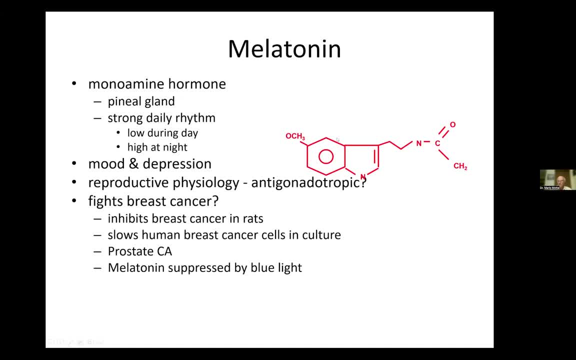 Here's the hormone melatonin. It's a very primitive hormone. It's present even in amoeba, So even amoeba make melatonin, and essentially every animal on Earth makes melatonin. Some use it for biorhythm, like humans. Others use it for other reasons. 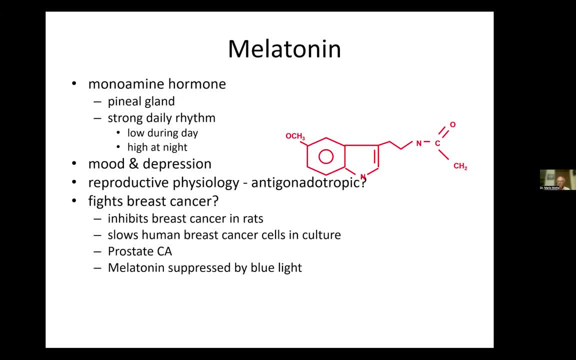 But it's a very primitive hormone that's been around for more than 500 million years in just about every animal. So it's a very primitive hormone that's been around for more than 500 million years in just about every animal. So it's a very primitive hormone that's been around for more than 500 million years in just about every animal. 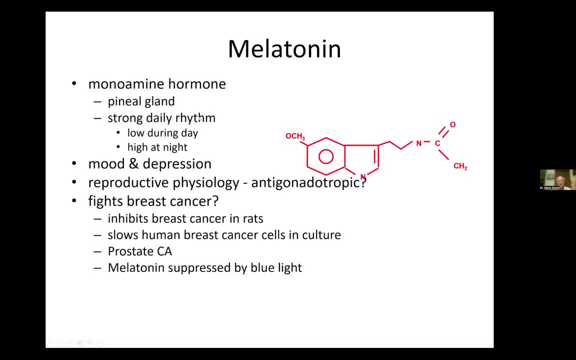 But in humans at least, it induces a strong daily rhythm. It's produced by the pineal gland primarily. Some is produced by the gut. If it's suppressed it changes mood and increases depression, and it helps fight breast cancer. So we'll talk about that in more detail. 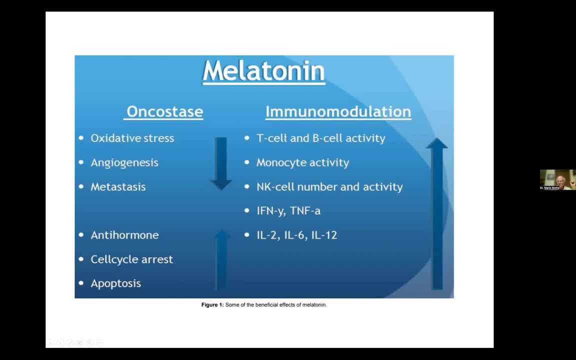 And the main reason why melatonin causes these problems, if it's suppressed, is because it modulates our immune system. So over here on the right it's known as an immunomodulation hormone, And by that I mean it helps T cells, which are killer cells in our body. 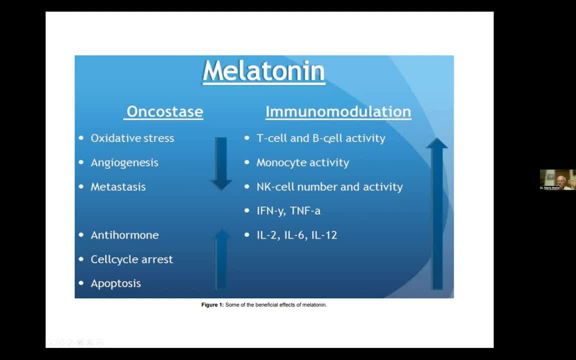 and B cell activity, which are the identifier cells that go out and spot abnormal cells, And then monocytes help and T killer cells help kill that. So if you have melatonin, it's not that light directly causes cancer, No one's saying that. But if you suppress your 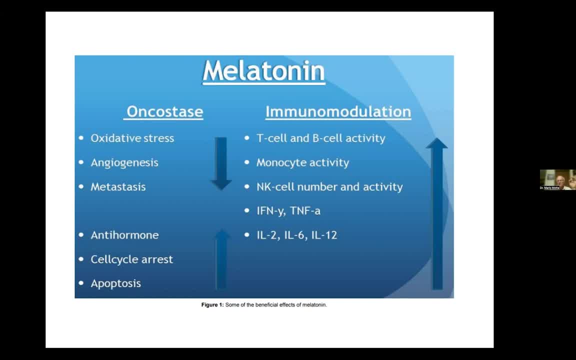 melatonin, then your immune system doesn't work quite as well. All of us produce cancer cells every single day. because we multiply and produce new cells daily, And it's not surprising a few of those may not divide properly and a few of those may become cancerous. 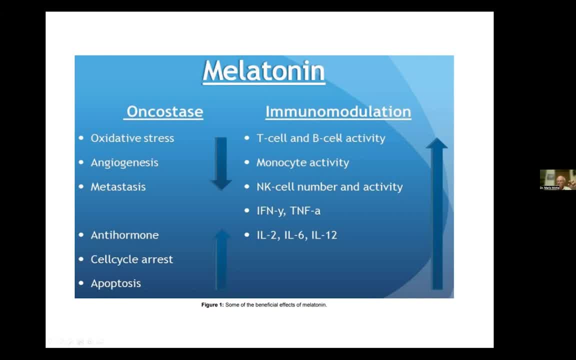 However, if you have a good immune system, you recognize and kill those off. So it's no stretch of the imagination to imagine that if you diminish the immune system in any way, then a few of those abnormal cells are more likely to escape detection. 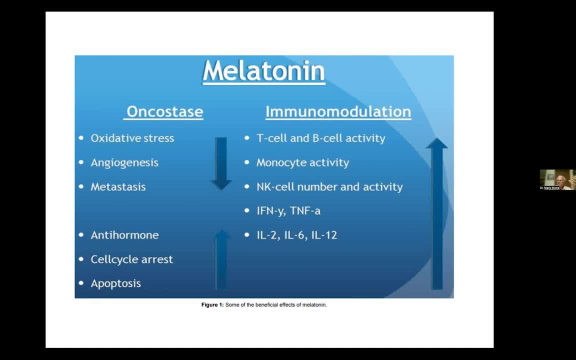 and eventually grow and become a cancer. And that's one of the reasons why older people tend to have more cancers, because their immune system tends to decline with age. So it all happens, But if we think about it, it's actually not that difficult to grasp. 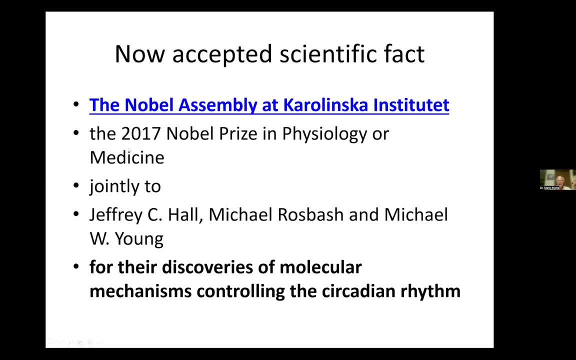 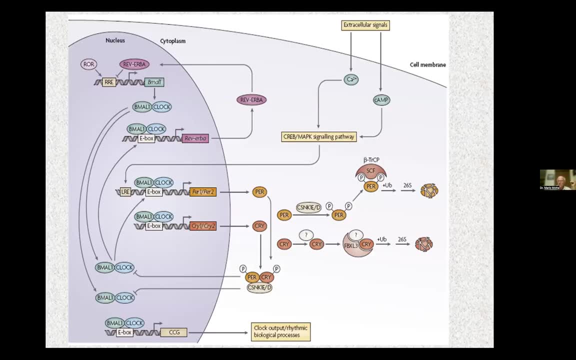 This is no longer in question. In fact, in 2017, the Nobel Prize for Medicine went to Hall Rosbach and Young because of their work in identifying the biochemical pathways of melatonin. This is based on their work. I'm not going to go through this. I just want you to know that. this is well established and is worth studying. So I'm going to go through this. I'll just give you a few minutes, All right, let's go ahead and start the presentation And then I'll just talk to the sort of the most important part of this. So I'll just talk a little bit about the 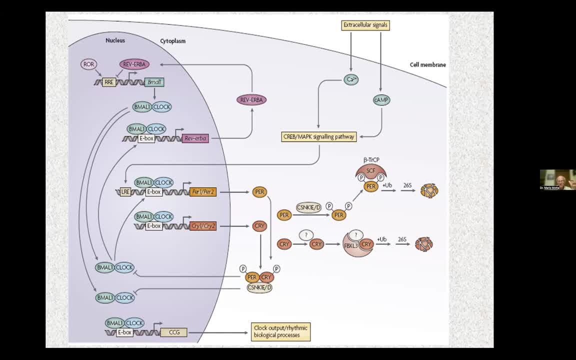 first part of this. So let's talk a little bit about the first part of this. So I'll just talk a little bit about the first part of this. So when we start talking about the first part of well written up and known and again, the Nobel Prize Committee thought it was important enough. 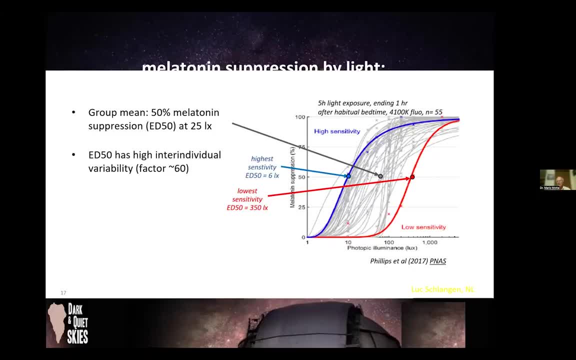 to give a prize for that. So some studies have been difficult to understand because there's a natural variation in sensitivity and that's not surprising. We all have different responses to different stimuli. So there are high sensitivity people to light pollution and there are low. 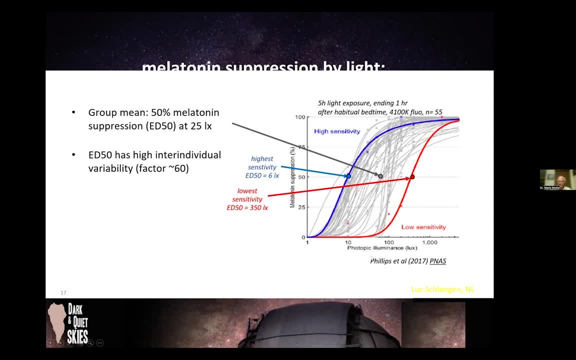 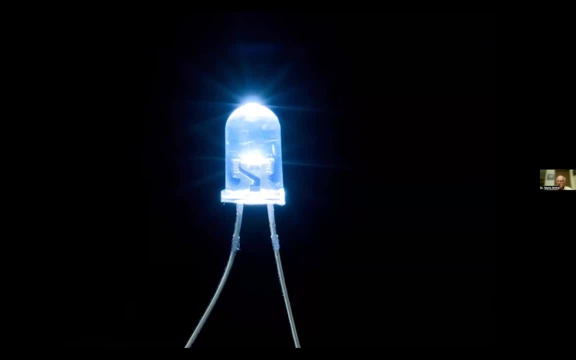 sensitivity Most lie in the middle, and this is from Phillips from 2017.. So what's the issue nowadays? We've always known that light pollution can cause a problem, but nowadays it's more acute. First of all, there's no such thing as a white LED, If anyone in the audience knows how to make. 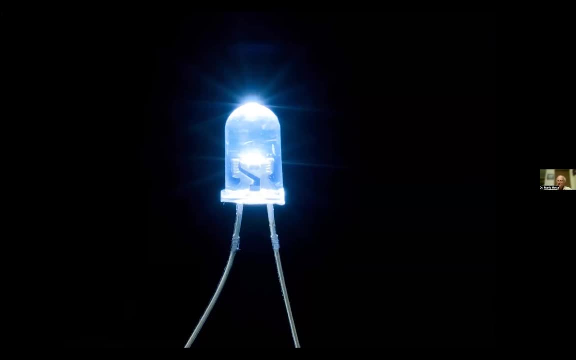 one. I guarantee you a billion dollars the next day. companies will be clamoring for it. The way we make a white LED is: you get a blue LED and you coat it with phosphors. The phosphors then take the high energy from the blue and absorb it, and 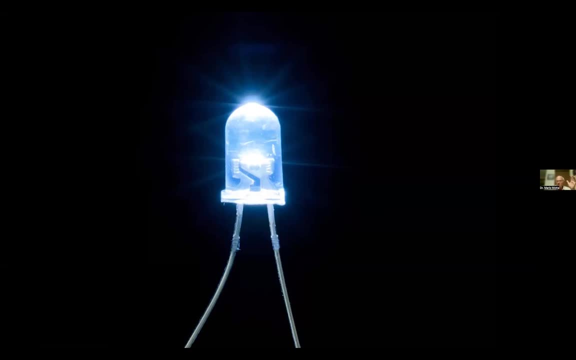 then re-emitted. it lower energy in the yellows, reds and greens, And that's how you get a white LED by covering the entire spectrum. The problem is the phosphors don't completely capture all of the blue And consequently a lot of blue escapes through the phosphors, And that's the problem. 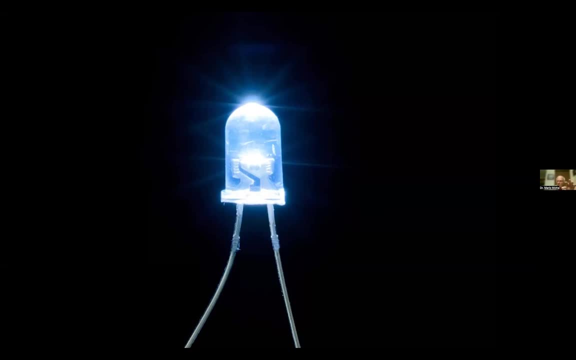 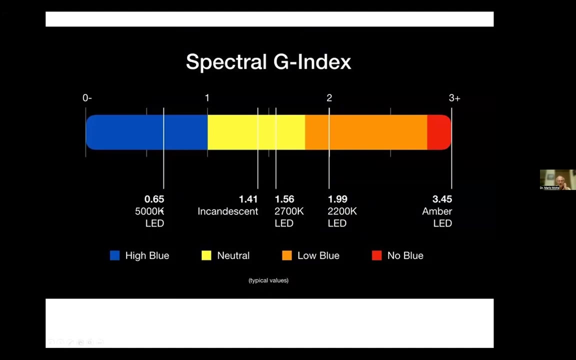 because blue light suppresses melatonin 10 times more than red light. So if you have a 5,000 KLED, a huge amount of that is blue: 65%. If you're in the 2,700 range, it's more like 17%. 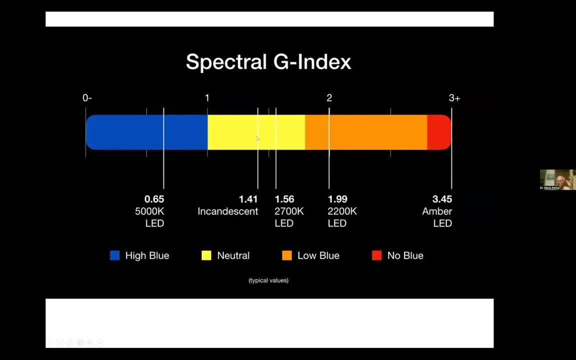 3,000.. Which is a common LED light is generally in the 20, 21% blue. That's still a lot of blue. The people in Quebec and Canada have got the right idea. They produce amber LEDs- zero blue- And that's actually the ideal solution. but no US company is making those. 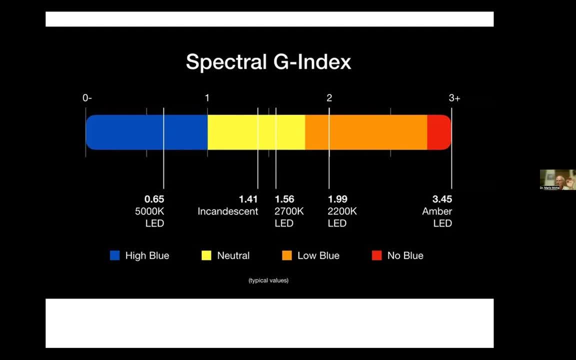 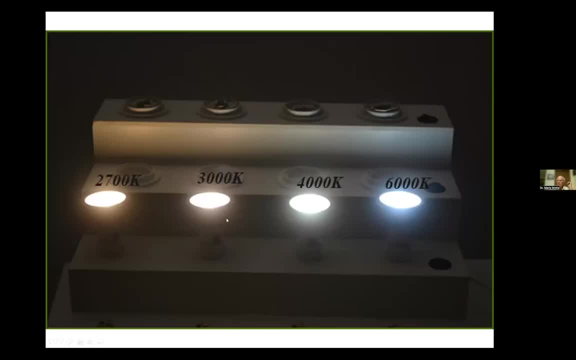 as of yet. I've been in Sherbrooke, Canada, and it's a very pleasing light, Doesn't hurt the eye. We should have got that, But we'll deal with what we have here. So each one of these in isolation will look white to you. if seen on a street, These will 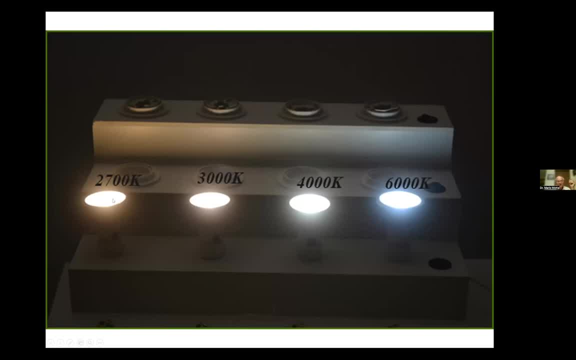 look intensely bright, white and kind of hurt your eye, And this is the best light right now. When the AMA did its recommendation for 3,000 K, we specifically said: in 2016,. 3,000 K are lower And every company seems to forget the or lower. We were anticipating future advances. The advances are here. 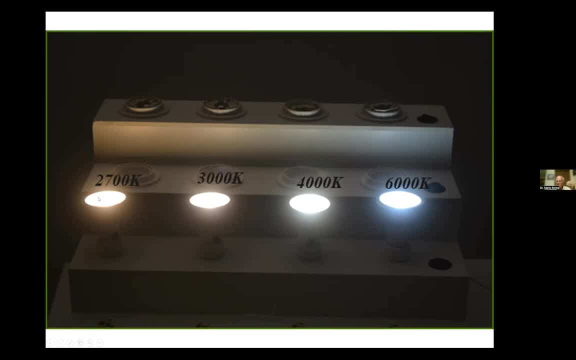 Nowadays, if we were writing this, we'd say 2,700.. In fact, Massachusetts Medical Society has recently adopted 2,700 K as the advised light, And there are lights out there. you now can get for street lights as low as 2,400.. Don't forget the high pressure sodium. we've all been 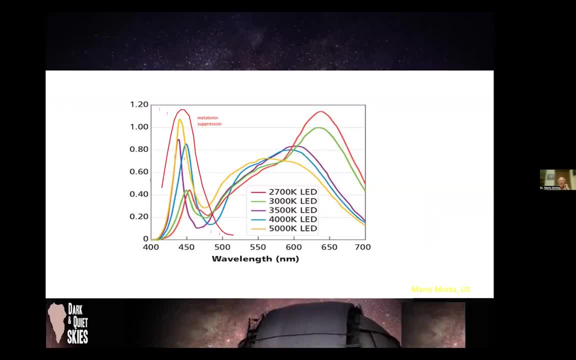 used to. Those are 1,800.. So here's the problem. This is the light. we want this hump, But here is the light. we get A lot of blue, And if you're at 5,000 K or 3,000 K, I'm sorry, 4,000 K, you get a lot of blue light. 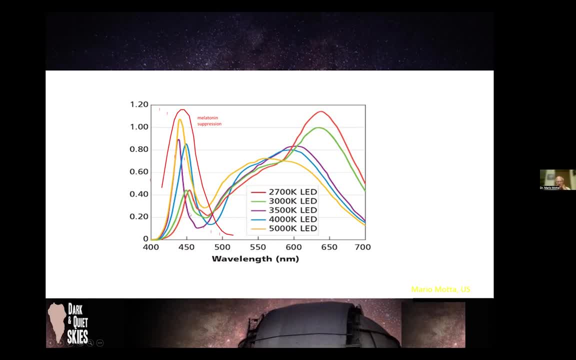 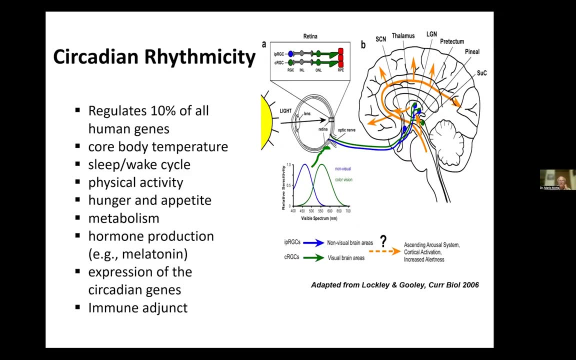 leaking through the phosphorus. Once you get down to 3,000 K or lower, the amount of blue is suppressed, which is why you should go with 3,000 K or lower, And the reason is blue light stimulates the pineal gland to one: wake us up, but two suppress melatonin. 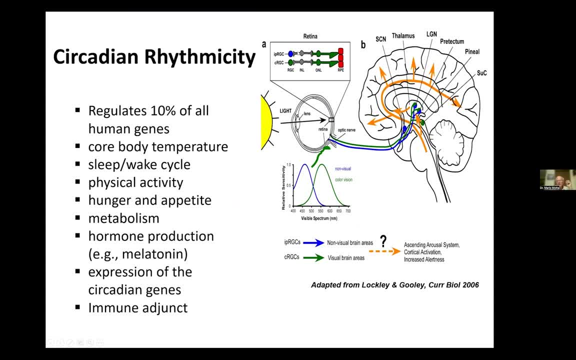 And that's through a new cone in the eye that was not discovered until 2003.. We all know that we have red, blue and green receptors And through that we have our color vision. And then we have a night vision receptor, which is black and white. But we have this other receptor that is peaks at. 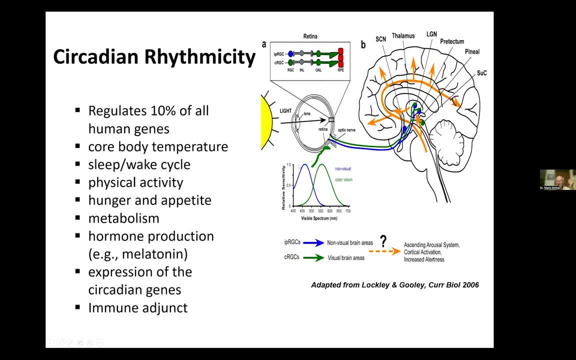 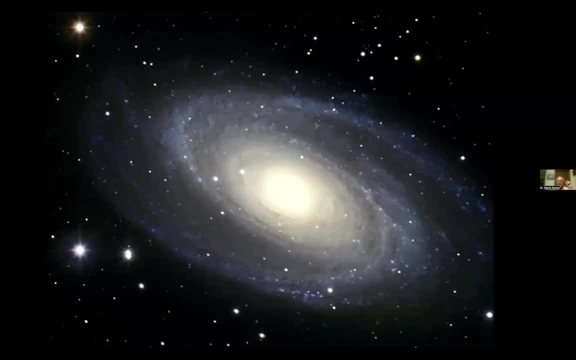 4,500 nanometers, And it only. It's not used in vision. Its only purpose is to depress melatonin production in the pineal gland. This is another image of mine: M81.. I know this is an astronomy club, right, So I have to throw in. 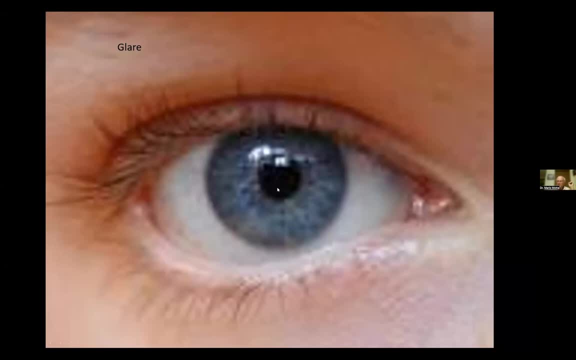 a few astrophotos. So let's talk about glare as a problem. The human pupil, at least when you're young, can dilate up to seven millimeters. When you're older, like me, probably only goes to five or six millimeters, And that's when you're dark, adapted When you're. 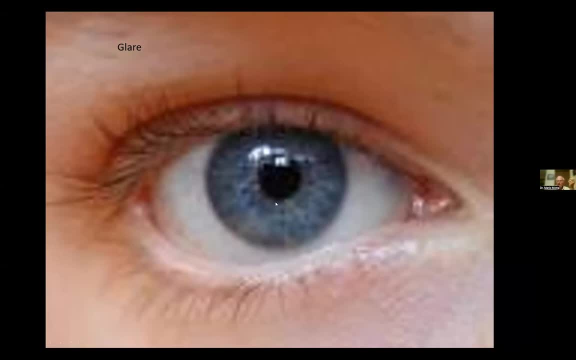 faced with glare and bright intense light, that pupil constrict down to one millimeter And that's important to note. So if you have direct light that's unshielded into your eye, your pupil constricts And then you only can see the light and everything else looks dark. 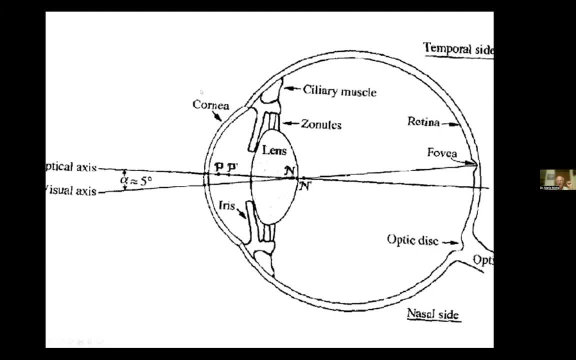 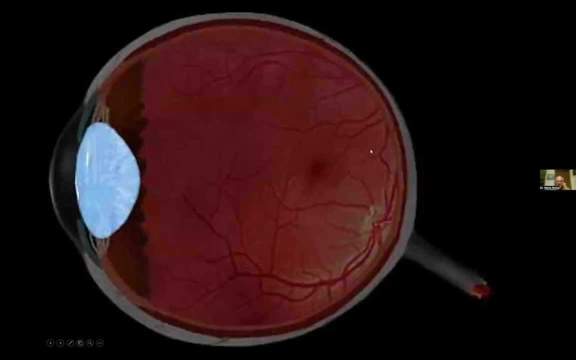 And that's the main concept of a glare problem. So light will come in through the cornea, go through the lens and gets focused, then goes to the back of the eye where, if you don't need to wear glasses, focuses right on the retina. Here's a human eye in a cut. 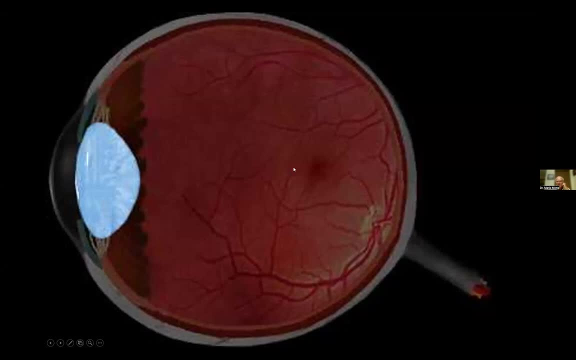 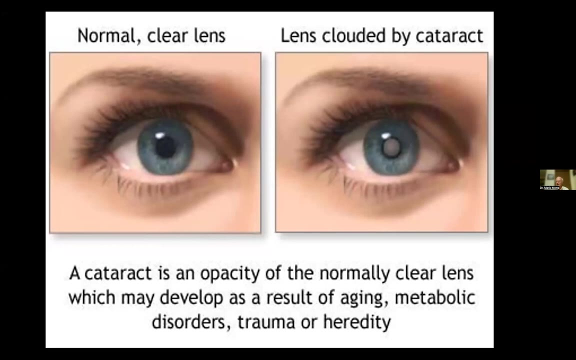 in half And you can see the lens, the cornea and the retina on the back and filled with aqueous humor. So the problem is we have a design flaw. As we get older, we have calcifications that develop in the lens And part of the problem is we have a design flaw. As we get older, we have calcifications that develop in the lens. 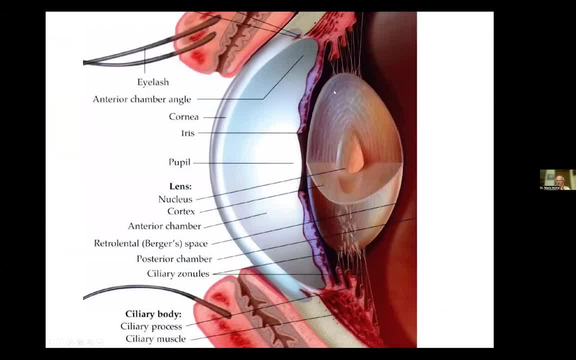 And part of the problem is that, in order to be able to see, there are no blood cells that go into the lens. So what happens is, as you get older, the lens continues to grow. New cells are laid on the surface, and those cells get their nutrients through the aqueous humor. 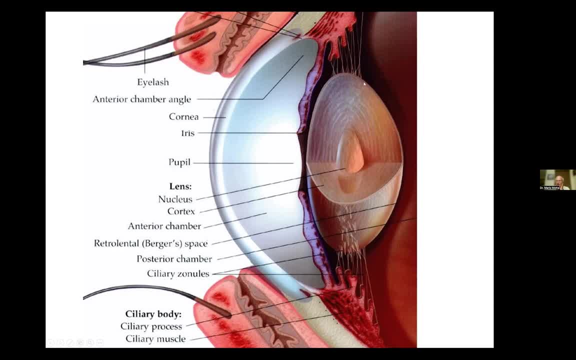 I'm sorry, the vitreous humor in the back- and get their oxygen and sugars that they need in order to stay alive. Once the lens gets thick enough- and that's generally in your 40s and 50s. the central 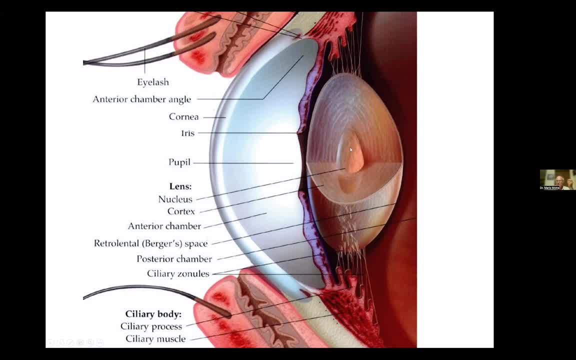 part does not get adequate nutrition or oxygen, Those cells start to die. When a cell dies, it calcifies. And then, when it calcifies, those are micro calcifications. now you have a scatter. when light goes through, that lens off these calcifications And blue light scatters more than red light. Eventually, in your 70s, you get a lot of red light. 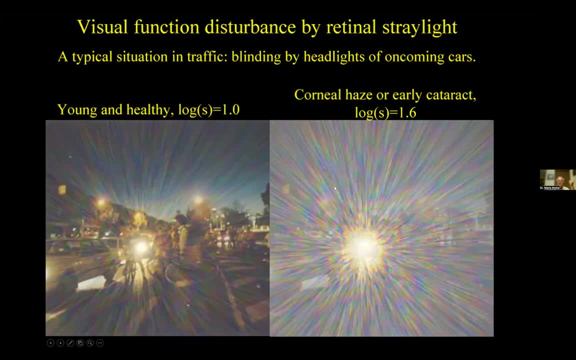 In your 70s and 80, this will coalesce and you have a cataract that you need removed. So if you're young and healthy and you have an intense bright source, you'll get scatter, but you can still see. But this is. 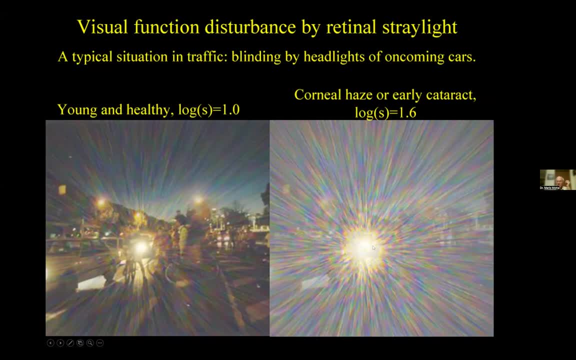 what a 70 year old eye will see. Basically, you have disability glare, which is why it's more dangerous for older people to drive at night. But it's not their fault. I tell people all the time the reason you can't drive at night is not your bad eyes, It's because we have bad engineering. 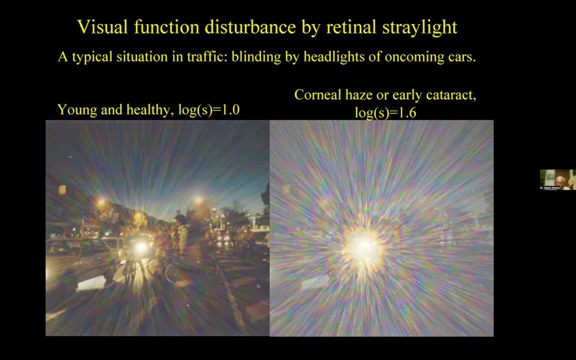 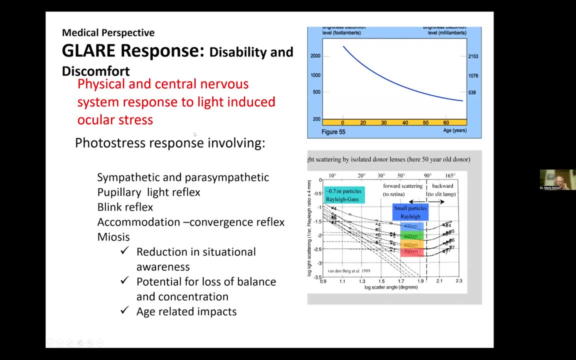 who designed bad lights. it doesn't have to be that way. so here is from: uh uh, the netherlands. uh, why don't i put his name down? i apologize, i didn't put the name down and i'm blocking my mind. who did this study? but when you're um in your 20s, you know it takes uh 1800. 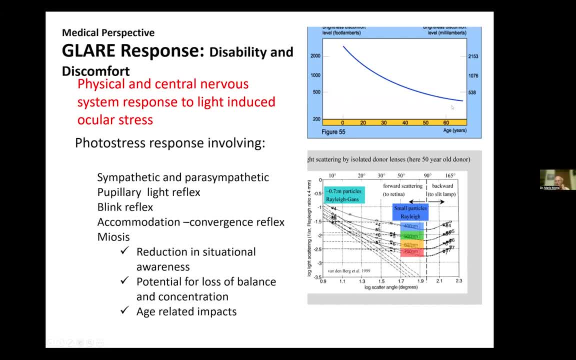 million lamberts to cause disability glare. by the time you're 70, it's a third of that. that's why older people have more trouble, and it's worse than that with blue light. now, this is a log scale, but these are human eyes that were studied in the netherlands and taken from cadavers and just like 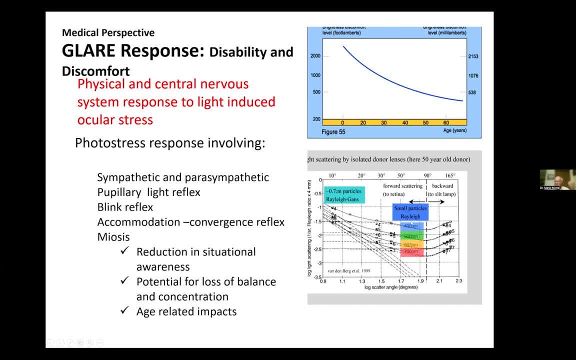 with the sunset you have red light penetrate and blue scatters- same thing in the human eye. so blue scatters more and red scatters least. so if you have a situation where you have a 4000k light, you have intense scatters, 40 percent blue. 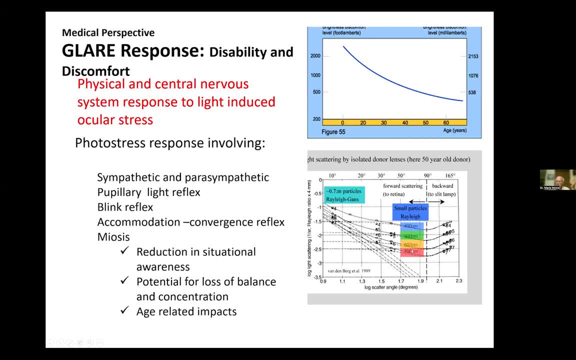 in the human eye, so that's why older people have more trouble, and it's worse than that with blue eye, and basically you're blinded, Whereas the warmer colors don't do that as much, although all light can scatter in the eye, which is why all lights should be shielded properly. 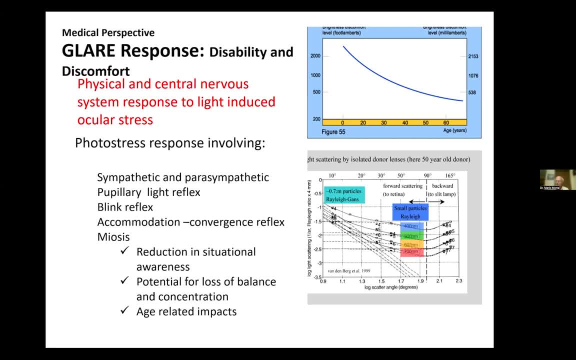 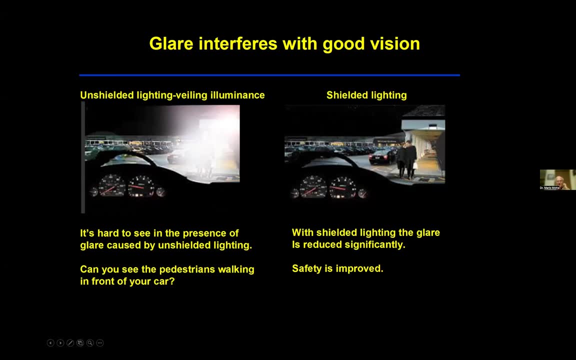 If you want to do a little experiment, take the lampshade off one of your lamps in a house and see if you like it. Most people don't. That's why we have lampshades. Same thing should occur on street lights. So if you have an unshielded light, you're blinded, and if you have it, 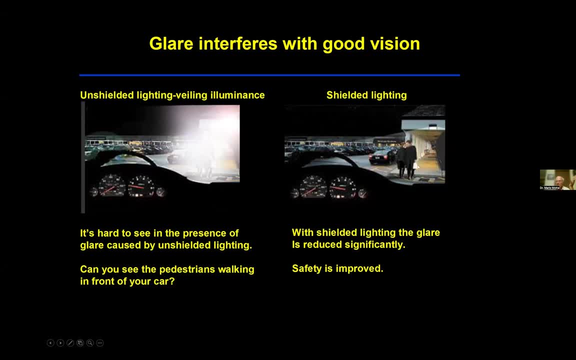 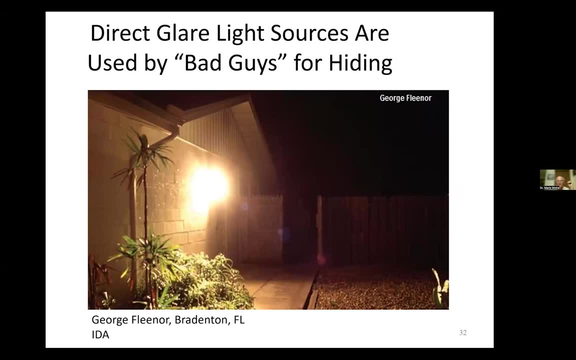 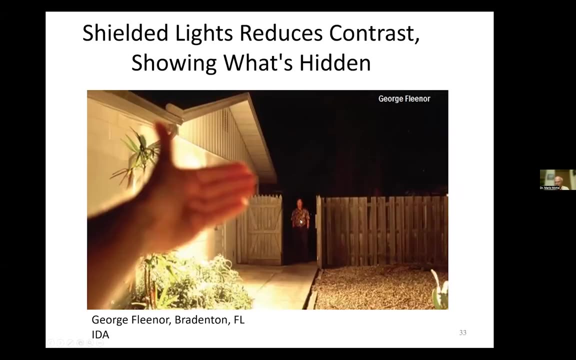 it's basically like having a dirty windshield, whereas shielded lighting is much safer. And here's a great example from Florida: You can't see that there's a person there, but if you shield the light now, you can see. Another example I took from my trip to Quebec. 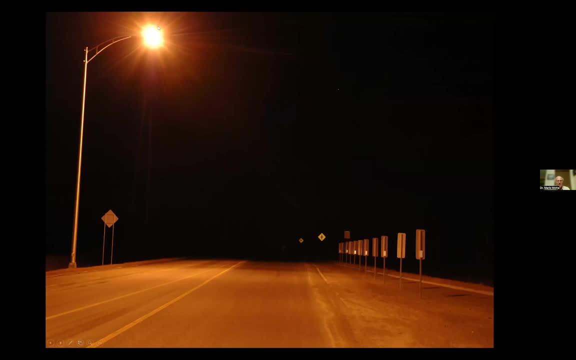 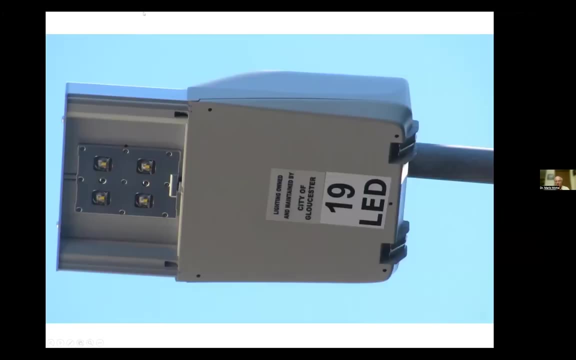 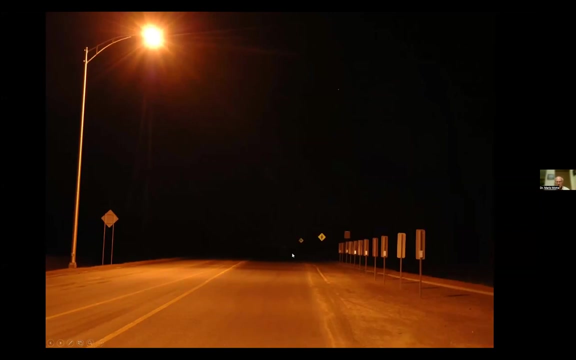 for a talk Kindly given to me. So many intersections- this is the beginning of an intersection in Quebec- have unshielded- oops, sorry, have unshielded lights, And what happens is, if you're driving along, I don't know why that's advancing on its own right. 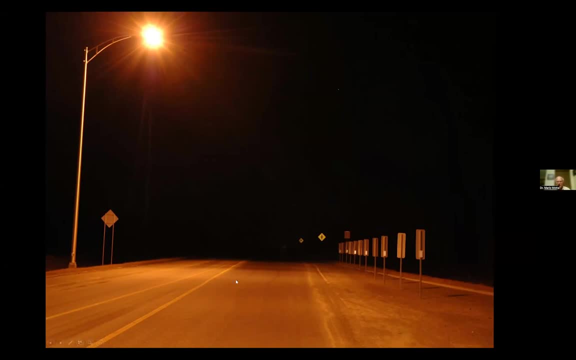 If you're driving along because of this, you're blinded as to anything down the road. So there could be a deer, an auto accident or a person standing in the road. You wouldn't know until you see it. You wouldn't know until you see it. You wouldn't know until you see it. 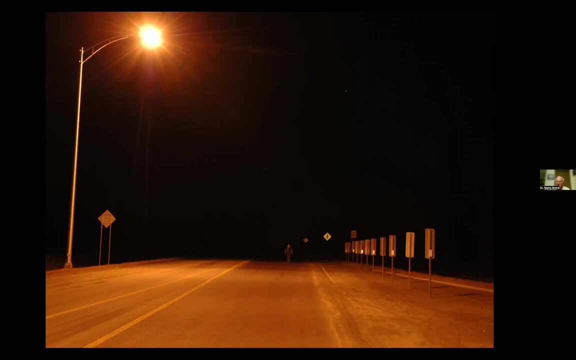 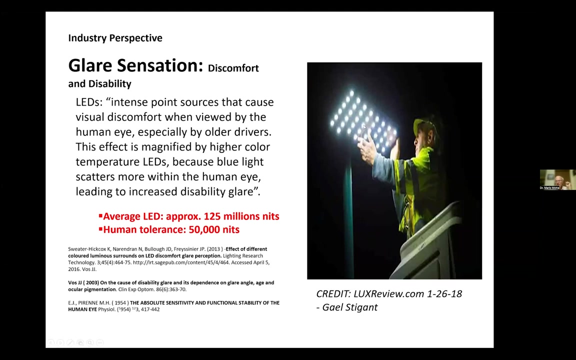 You hit them And again, that's not your eyes. It's bad engineering. They should be shielded and you'd be able to see down the road much better. We shouldn't allow that in public roadways. It's worse with LED lights because they're intense pinpoint lights And in fact in France they've. 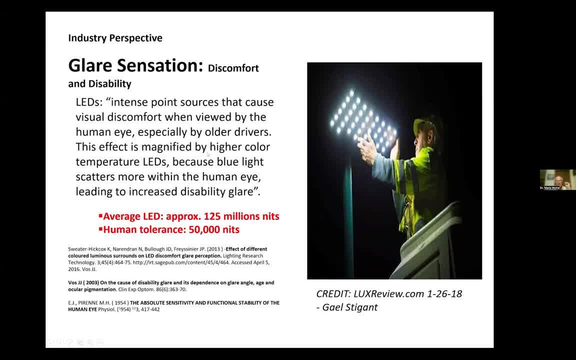 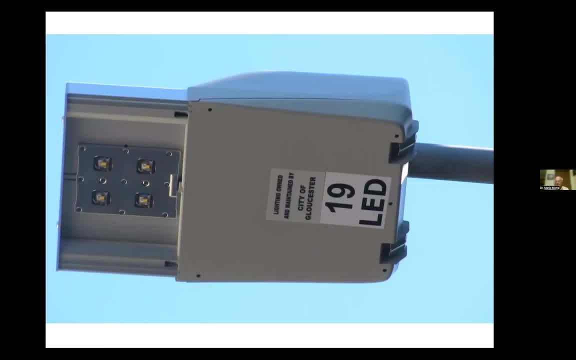 basically mandated that these be shielded. I wish the US would do that. And when they're blue it causes intense disability glare. In my hometown of Gloucester I was in a town council 14 years ago. We were one of the first adopters And notice: this is 19-watt LED. We were replacing 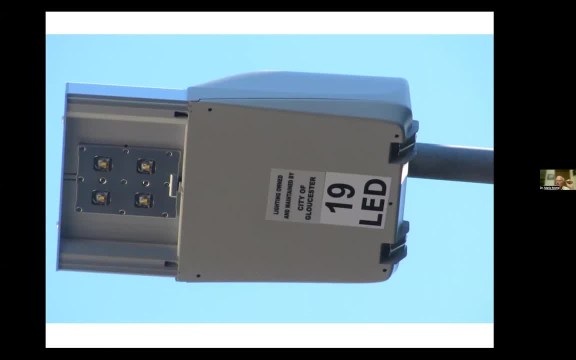 60-watt high-pressure sodium. Everyone's got to remember, when you talk to your city councilors, that there's a four-to-one ratio. So a 60-watt high-pressure sodium is the to get the same lumens. you want a 15-watt LED because of the four-to-one ratio. Unfortunately, far too many. 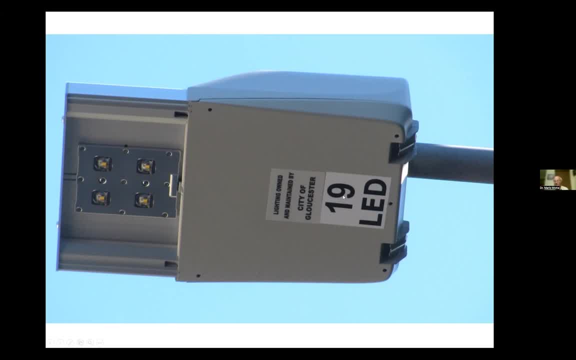 city councils think well, and lighting companies are complicit in this. If you replace it a 60-watt, well, we'll give you a 50-watt. Now you have four times as much light as you started with. It doesn't matter what the color correlated temperature is, whether it's 3000K or 2700K. 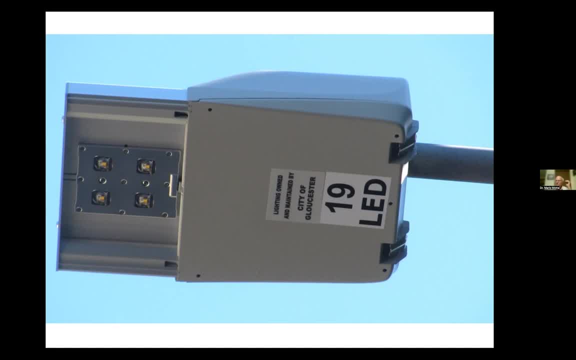 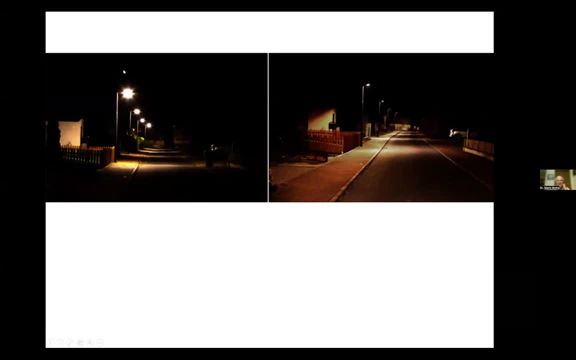 If it's way over lit, it's way over lit. You got to demand that you have proper lighting and not over lighting. So here on the left is a street that was lit up on shielded lights And then, when switched, to LEDs. 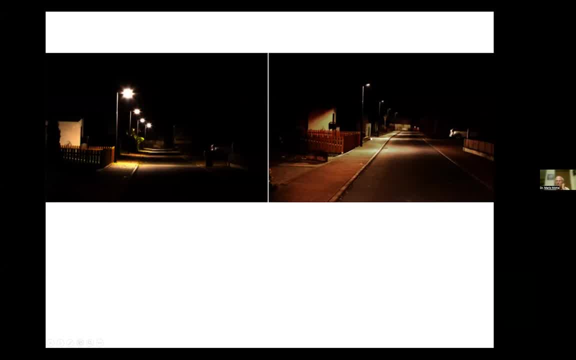 proper lighting. with shielding you can see much better on the right than you can on the left, And that's with the same exposure. on the camera, Which would you rather drive down or walk? I picked this one In Gloucester, one way to convince. 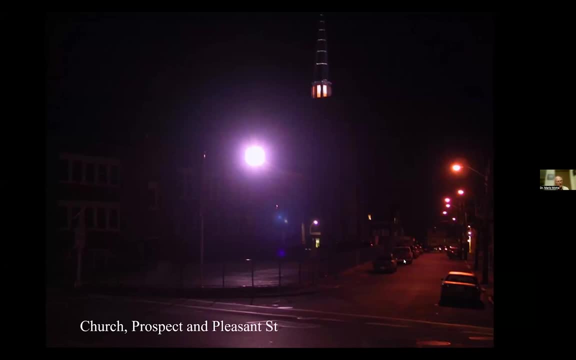 city councilors and police departments. I actually asked for a list of intersections with the most accidents. It was: here's the winner: in Gloucester, This is a church, St Anne's Church, near the center of town, And here's a school by the church, And they had this quote. 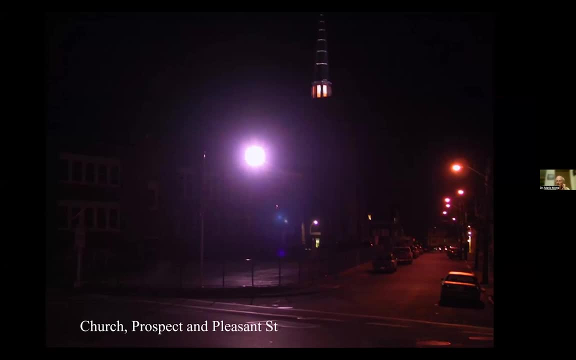 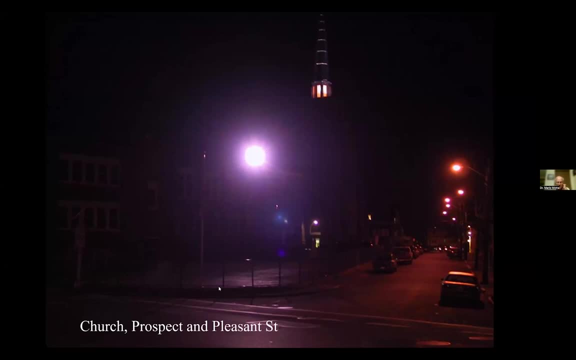 Because of the glare. There is one light pole here that's supposed to be lighting up the street. It never turns on because the light sensor thinks it's daylight all the time. So you have no proper lighting And the glare basically drives, causes glare and causes accidents. So it's no surprise. 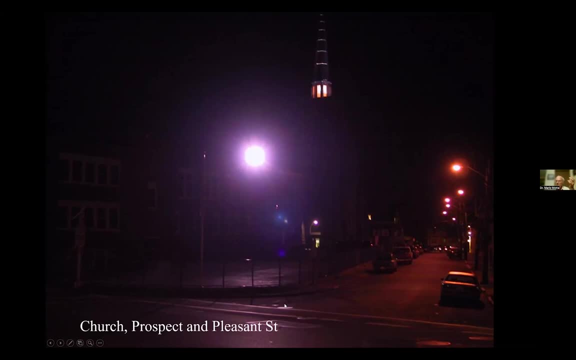 that over a five year span there were 19 accidents in this intersection. It took this to convince a city council. this is why you're getting so many accidents here. We convinced the school to take that down and put up a shielded light. Accident rate went way down. 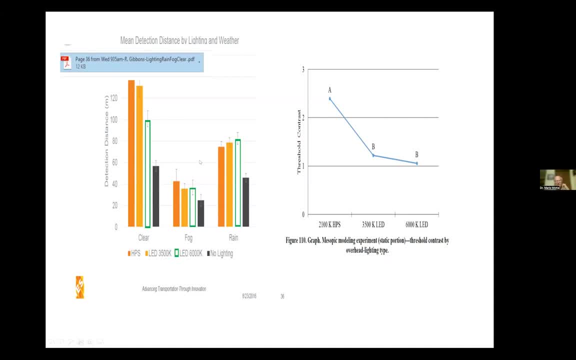 IAS Ron Gibbons from Virginia Tech did a study some years back where he showed his high pressure sodium and 3,500 K LED and 6,000 K LED. Notice you could see better down the road with the 3,000 K LED than you can with the 6,000. That's because 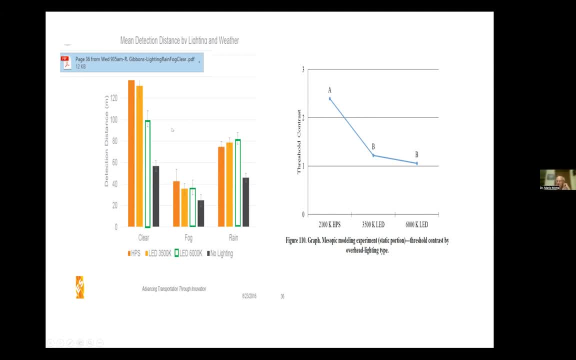 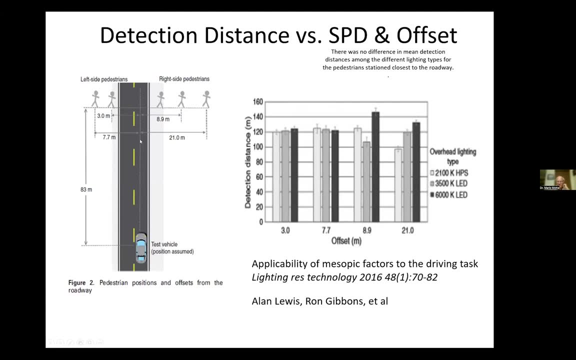 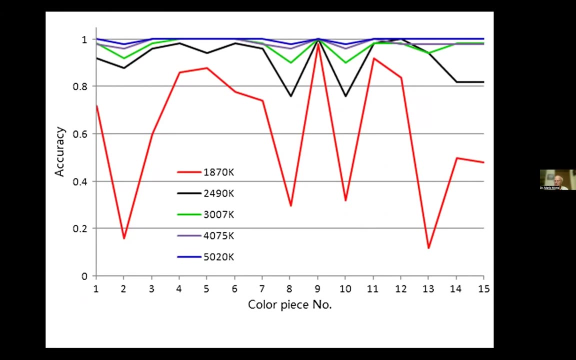 of all the glare that comes from these high intensity lights. Here's another latest study that showed basically the same thing. So you'll hear a lot from some lighting companies. Well, we need the 5,000 K so you can see color better, And that's complete balderdash. The red is 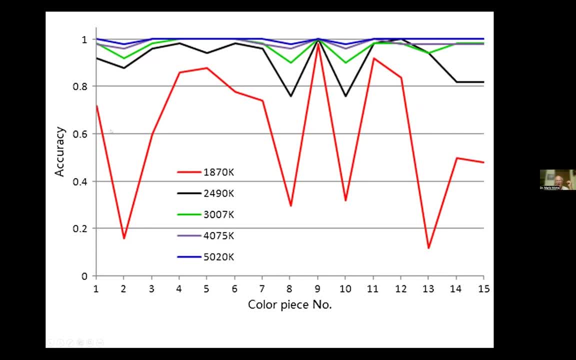 1,800,, which is your high pressure sodium, And yeah, there's some color rendition problems with that, But up here you have 5,000, 4,000, and 3,000 K lighting. There's essentially no statistical. difference in the color rendition with any of those. You don't need 5,000 K to see color at night. I'm not even sure you need color at all. Again, we lived with 1,800 K for 30 years without. any problem. IAS Ron Gibbons from Virginia Tech did a study some years back where he showed that the 5,000 K LED and 6,000 K LED can be used to see color better. And that's complete balderdash. 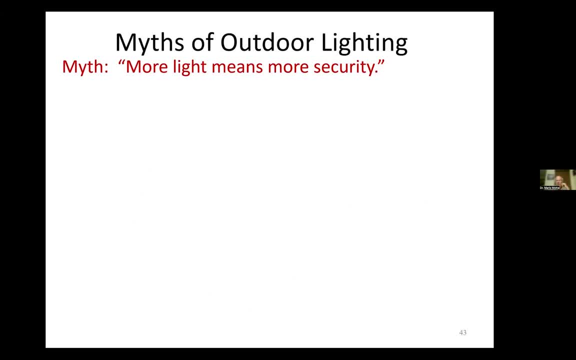 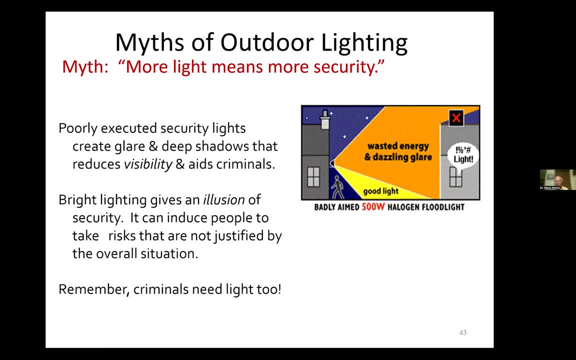 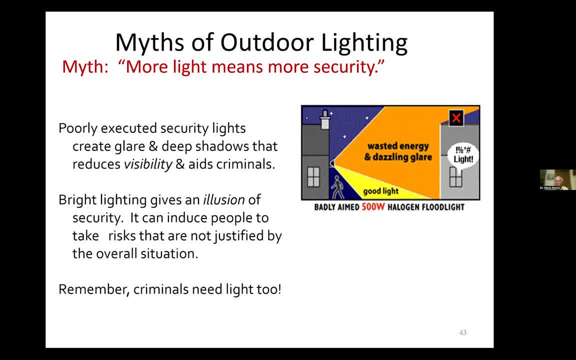 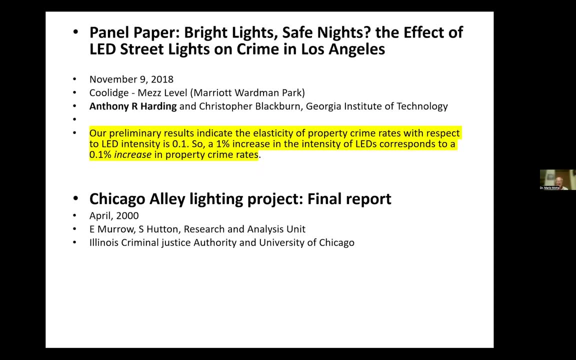 school systems. they get vandalized. A simple way to do it is to turn off the lights and put motion sensors, because teenagers are like moths, They go where the lights are. You turn off the lights, they don't congregate there and you don't have the vandalism And you have multiple studies that. 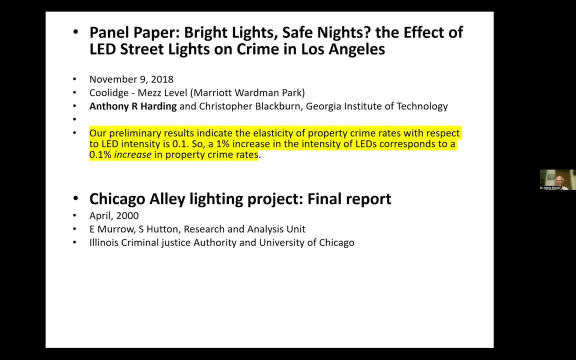 have shown that there's no difference between lots of lights and low light to prevent crime. Are studies out there that purport to show the opposite? Whenever you see a study, look who funded it and who did study. almost off Any study that I've seen that shows. 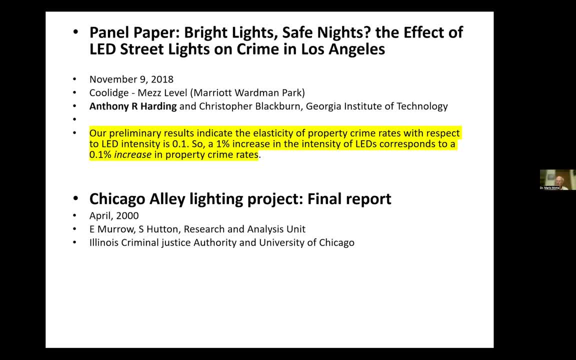 oh, you need more. lights are always funded by a lighting company to sell their product. I've yet to find exceptions to that rule, So you gotta find studies that are independent. So you're. So here's a study 2018,. and they showed that crime rates with respect to LED intensity is 0.1.. 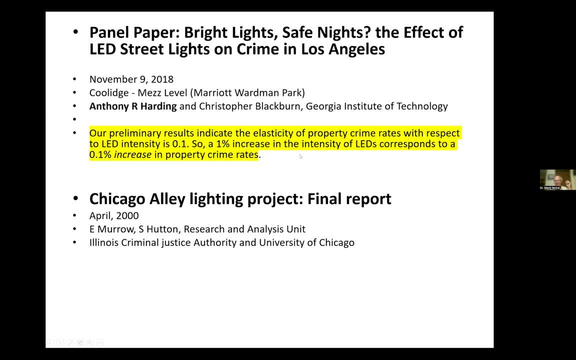 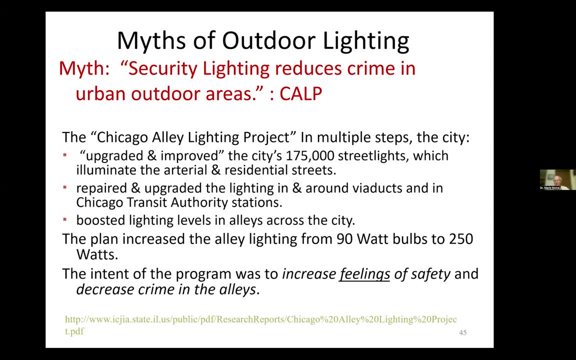 So a 1% increase in the intensity of LEDs corresponds to an increase in property crime rates, not a decrease. Then there's the famous Chicago Alley Lighting Project. OK, so Chicago got a grant to light up all their alleyways because there was crime in the alleyways, supposedly. 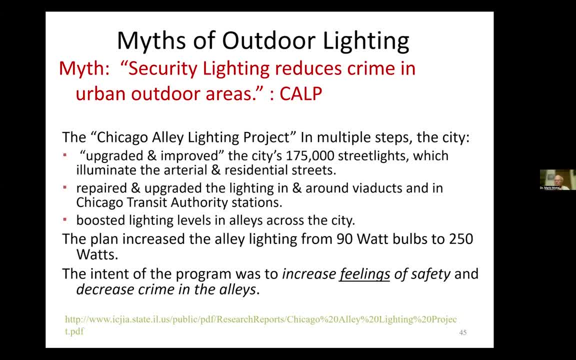 And they ran out of money about two thirds of the way through. So they had this two thirds alleyways lit up, one third not lit up. So University of Chicago and this group here decided that would be a perfect study to prove how well this program worked. 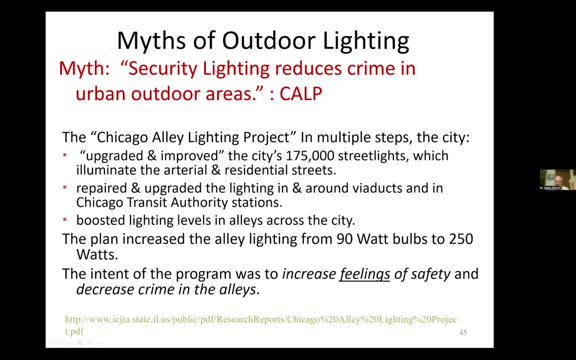 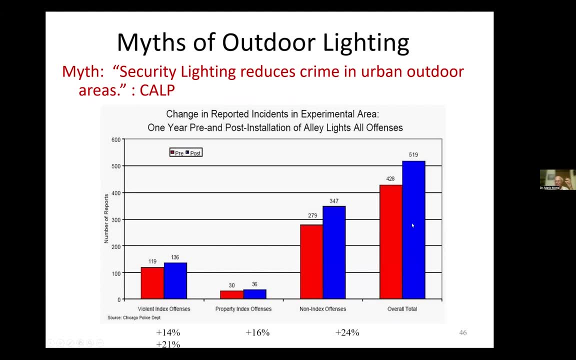 So, unfortunately for them, after they changed all the alleyways- 250 watts, by the way, high, huge lighting- they had a feeling of safety. But the actual result: every place they lit up better had the crime rate increase And the places that were left dark actually decreased. 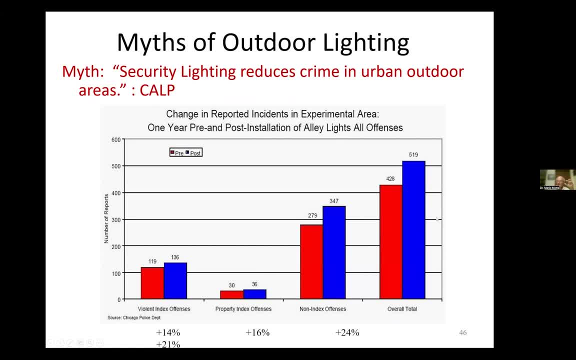 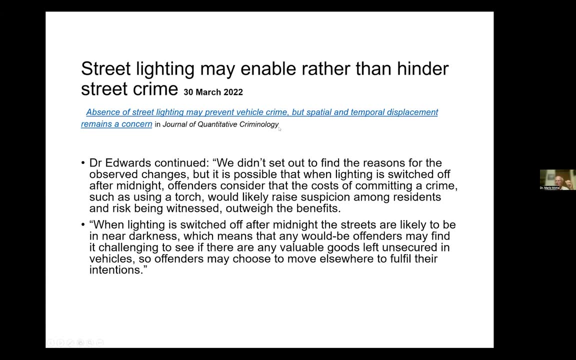 It's because the criminals went to where they could see better. That's a landmark study. by the way, They went in with a bias, thinking the opposite, and proved that they were wrong. Street lighting may enable rather than hinder crime And, in general, quantitative criminology. this is a legit study. 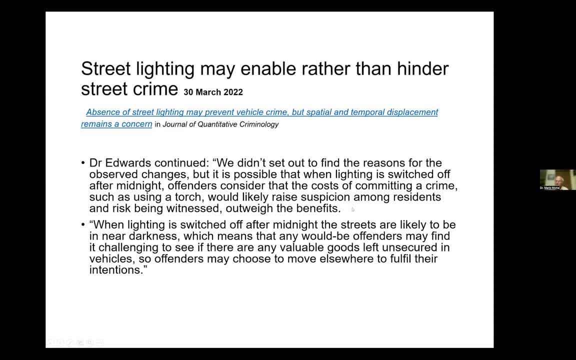 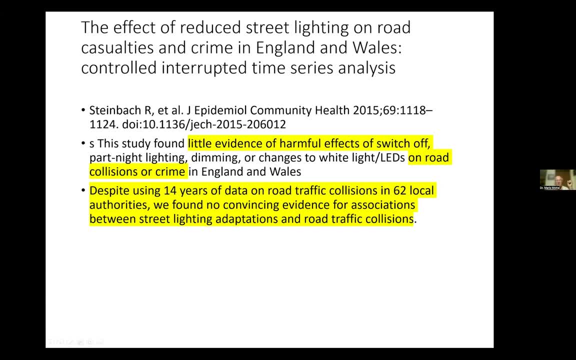 And it shows that there is no evidence that increased lighting causes increased crime. Decreased lighting causes increased crime. So reduced lighting, So reduced lighting in England and Wales show the evidence of harmful effects of switching off on roadway collisions of crime in England and Wales. 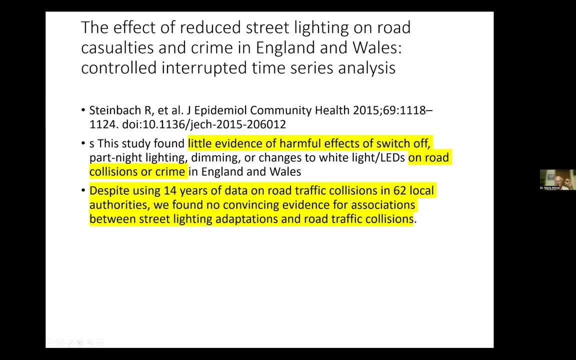 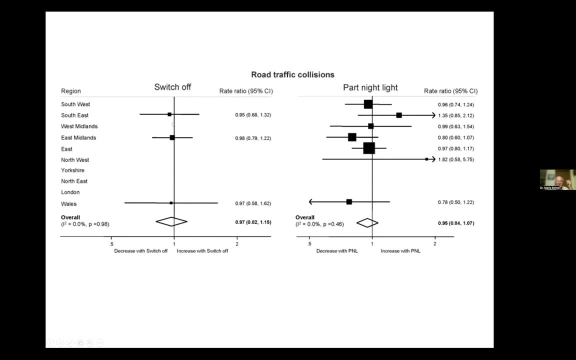 Despite 14 years of data on road traffic collisions, they found no convincing evidence for association between street lighting and road traffic collisions- none whatsoever, In fact. here's some of their conclusions. If anything, when they switched the lights off, there was a slight movement to less traffic. 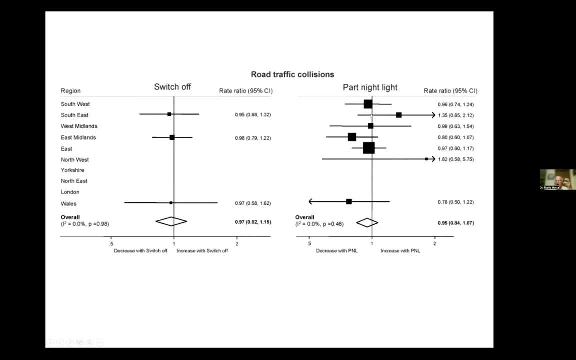 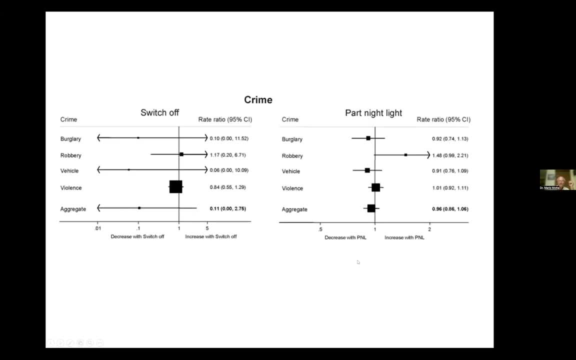 And part-time lighting, meaning they turned it off after midnight. There was one town that increased, but most of them decreased Crime, basically not significant either way. And part-time lighting- again not significant either way. So lighting does not change crime rates or accident rates. 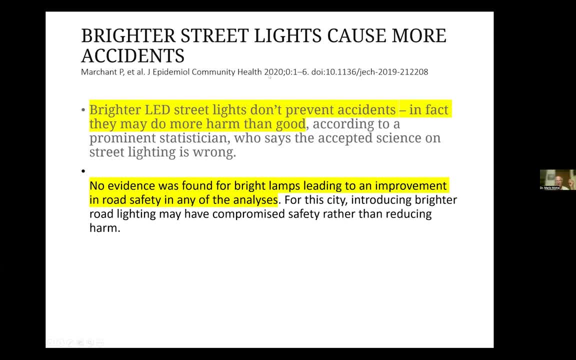 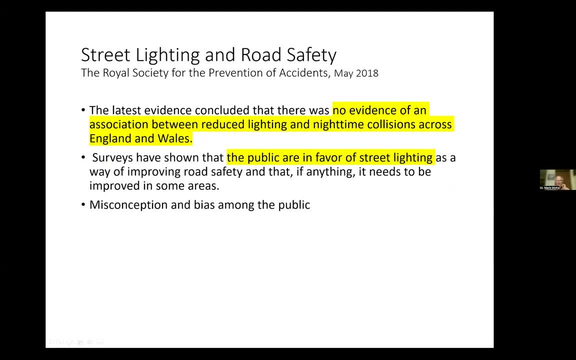 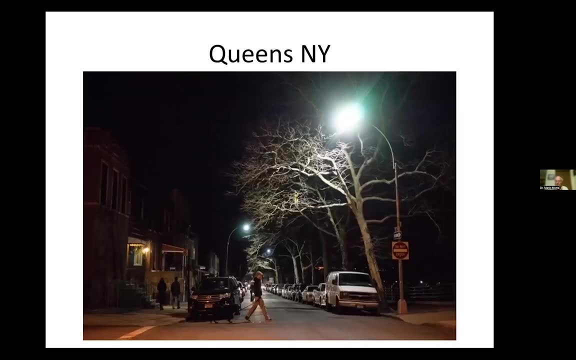 In fact, brighter streetlights cause more accidents. Another study here from 2020.. Street lighting, road safety, Royal Society, prevention of accidents. No evidence for association of reduced lighting and collisions. Now the same thing is. there are other reasons to not use the 4,000K lights. 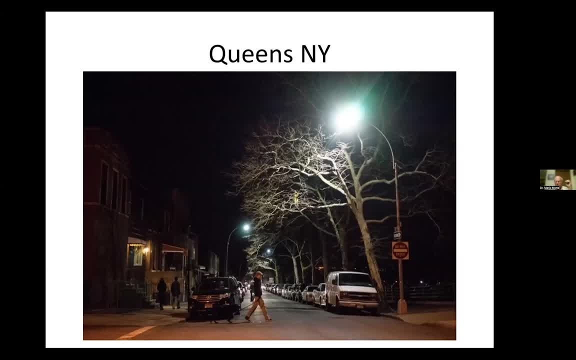 Queens, New York, early in around 2012,. Queens decided they were going to put up 4,000K lighting. They're awful. Just look at these. Until you live next to 4,000K lights, you don't realize how bad they are. 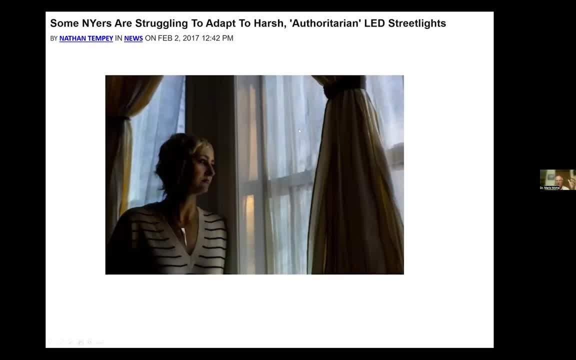 So people, People complained endlessly. This is what someone's bedroom looked like, And you just can't keep this light out. It only takes a little bit of light to suppress your melatonin. So eventually they stopped the project and switched to 3,000K. 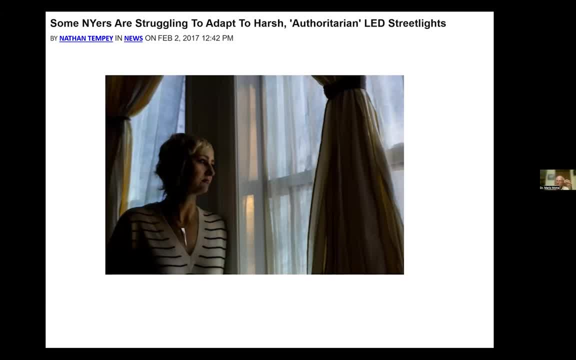 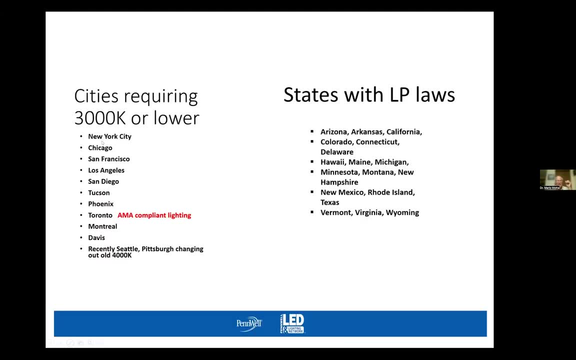 Now again. New York City is one of the most light polluted areas in the universe. Even there they don't like the 4,000K lights. Since then, many cities now require 3,000K or lower. Some cities that were early adopters, like Seattle and Pittsburgh, that put up 4,000K. 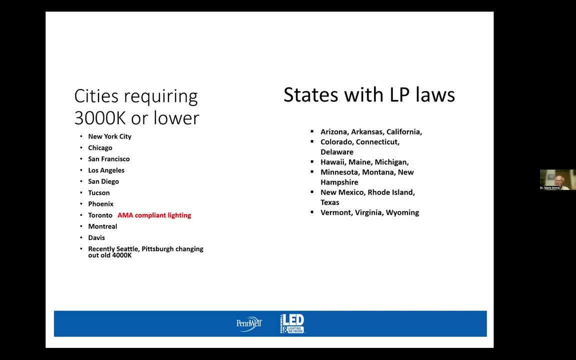 lights in the last two years, voted to take them all down, And the reason is the townspeople hate them. So what I tell people all the time is: don't be foolish, Don't put up lights that others hate and want to take down. 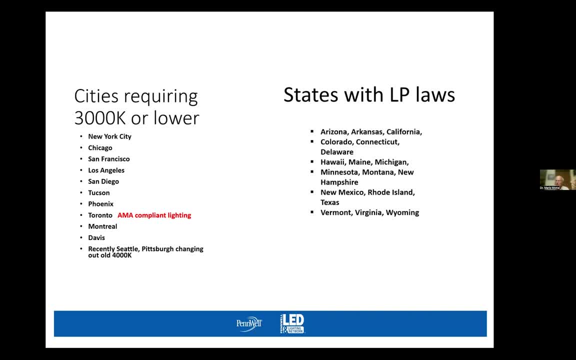 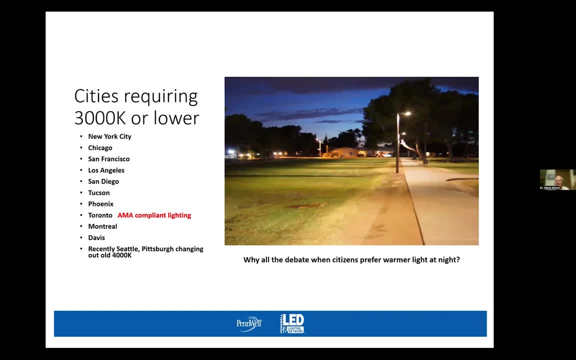 They'll cost you double. That's the only way to get rid of them. Take them down. They last forever. So this is what 3,000K lights looks like. It's very pleasant, It doesn't hurt the eyes, Especially if it's shielded. 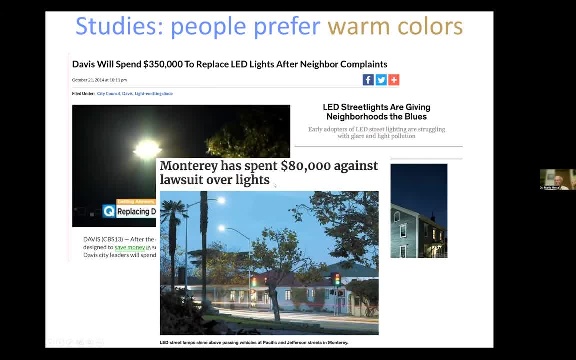 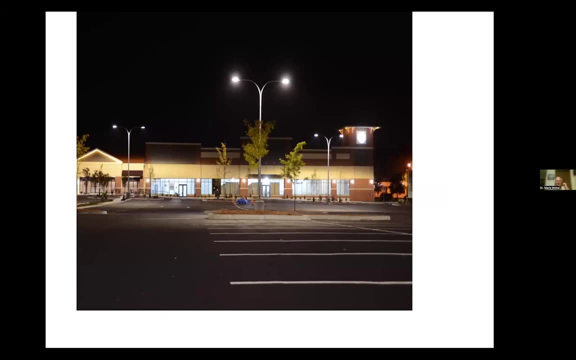 And some cities act. Monterey actually sued their own city when they went against their recommendation over lights. Davis actually raised their tax rate to get rid of the 4,000K lights. When's the last time you heard that That's how much 4,000K lights are hated? 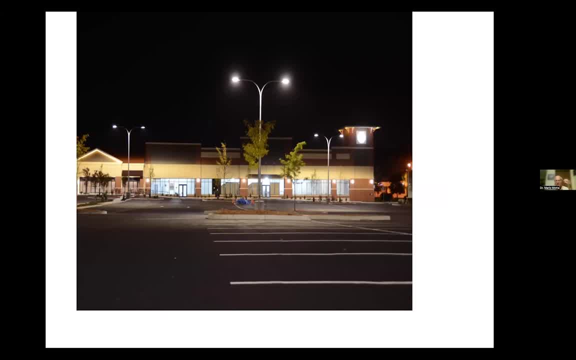 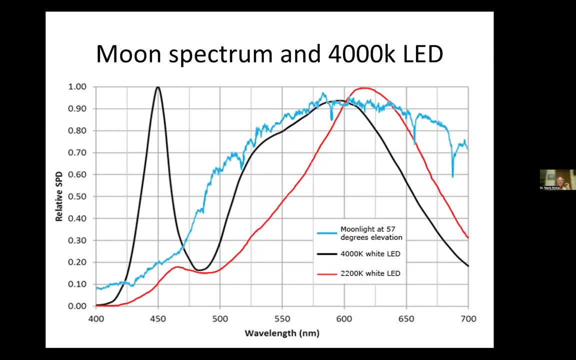 Here's a shopping center not too far from me. They have 3,000K lights. I'm sorry, this is 2,700.. You can see the color's perfectly fine And it's pleasant light. And now here's another thing. I hear engineers misquote a lot. 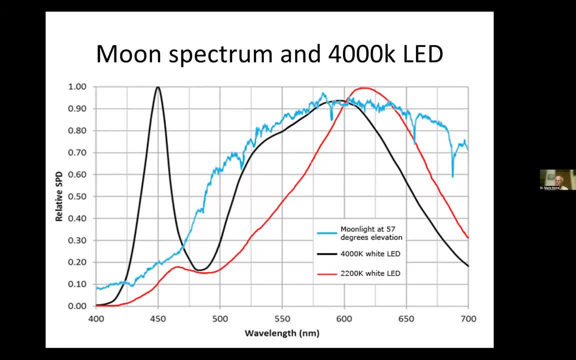 They'll say, wow, 4,000K is the color of the moon. So what are you complaining about? And I've actually heard that when I've spoken to engineering groups, And that's why I include this slide, because you may hear this all the time. 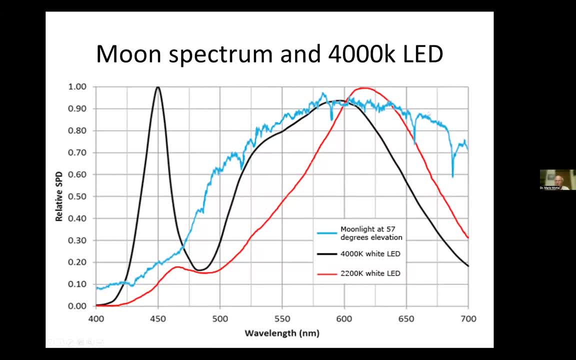 So this blue line is a spectrum of the moon. The red line is 2,200.. The black line is 4,000.. Notice this spike here. That's the blue that penetrates. That's not found in moonlight And that's why I include that on my slide, so I don't have an engineer saying but the moon. 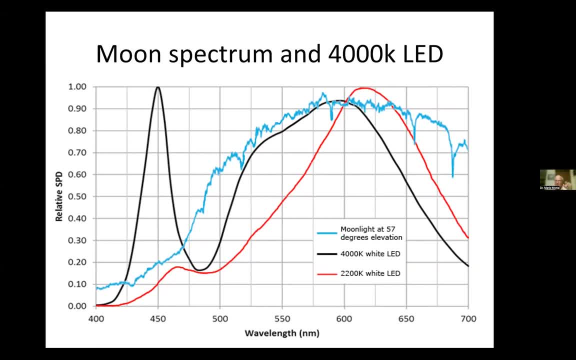 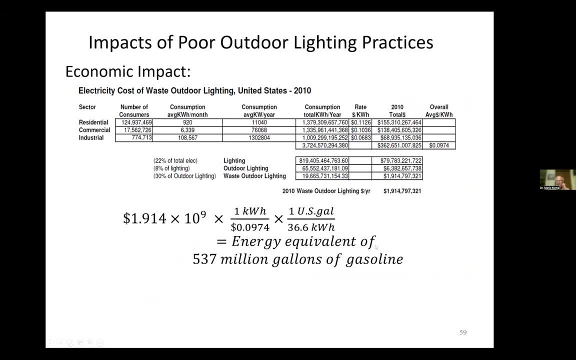 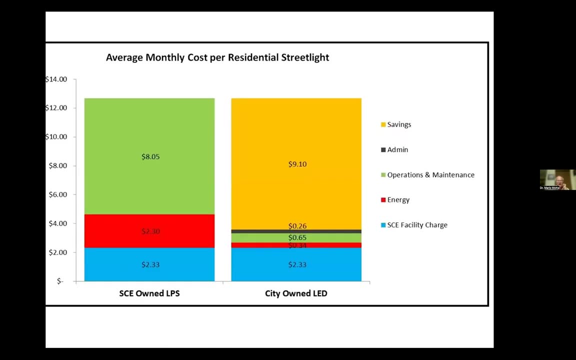 And I say yes. what about the moon? Here's what proves you're wrong immediately. So there's an economic impact. We waste lots of energy by lighting up things we don't need to and by lighting up the sky- Typical science. 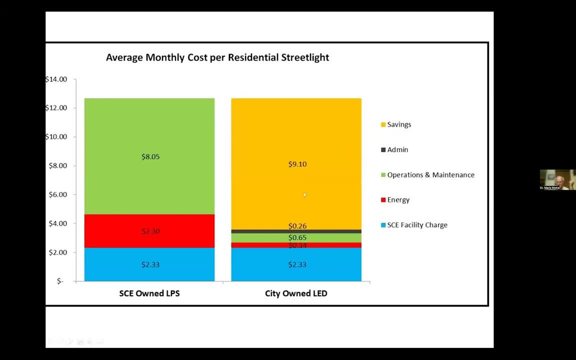 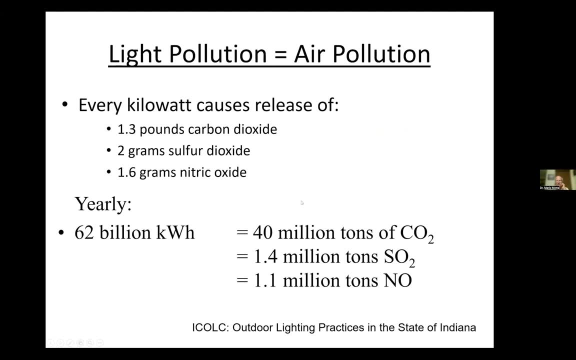 The city-owned LED light. this is how much it costs to maintain and run. Light pollution equals air pollution. I know in Texas you're still using a lot of fossil fuel. Well, this is how much you're contributing to global warming when you do. 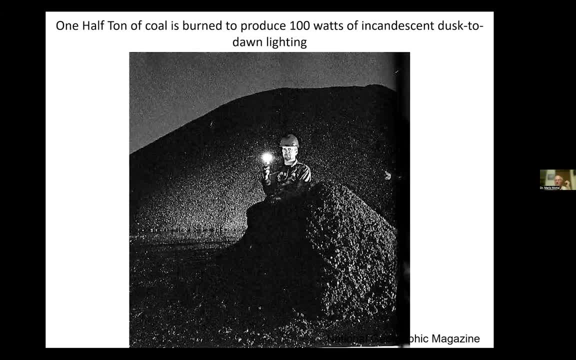 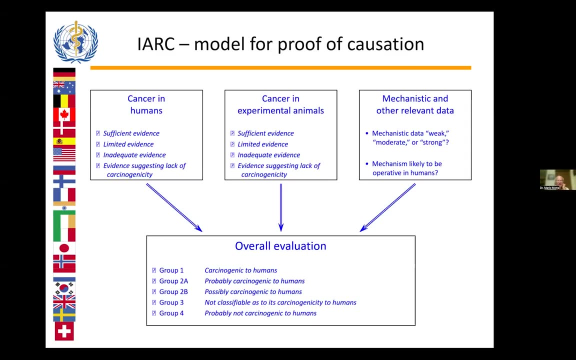 So to put it another way, 100-watt incandescent light all night long, for one year is a half ton of coal. Let that sink in. OK, here's my view of the Trifid. All right, so the IARC back in 2009,- claimed, stated that melatonin suppression is a probable 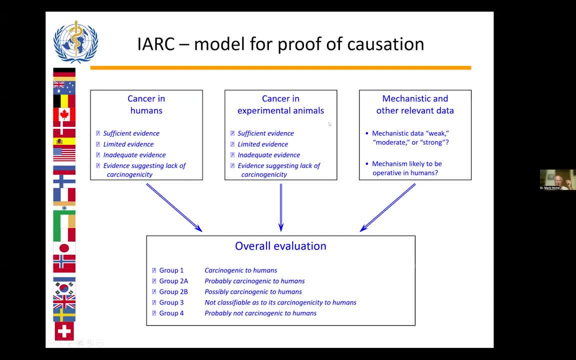 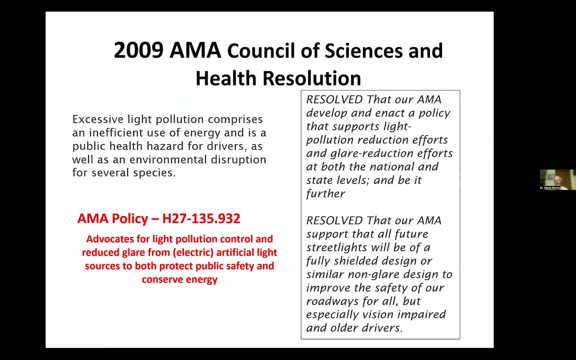 carcinogen to humans. Mind you, here's what it takes to declare that. And cigarette smoke is in the same category, group 2A. OK, So because of that in 2009,, I was able to get some resolutions passed through the AMA. 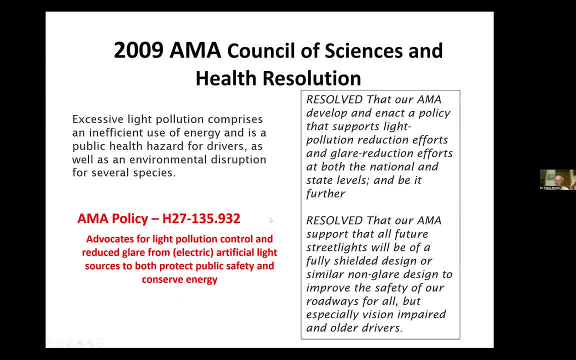 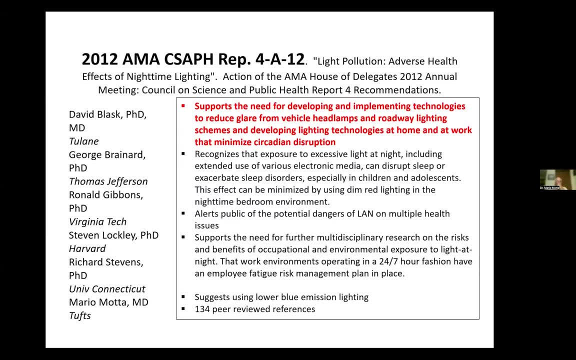 First was simple: shielded lights. That's kind of a no-brainer. No light should be unshielded. That's been AMA policy since 2009.. That's what we recommend 2012,. when I was on the Council of Science and Public Health, light pollution was becoming. 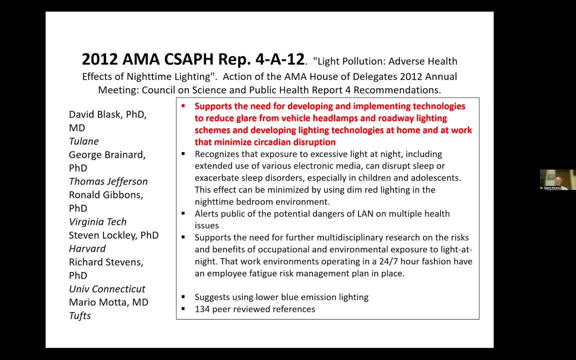 a real problem and we're starting to switch to LEDs. And I've been reading all these reports about light pollution. I invaded some of the. I've been talking to some of the country's best researchers- Gibbons, Brainard, Lockley. 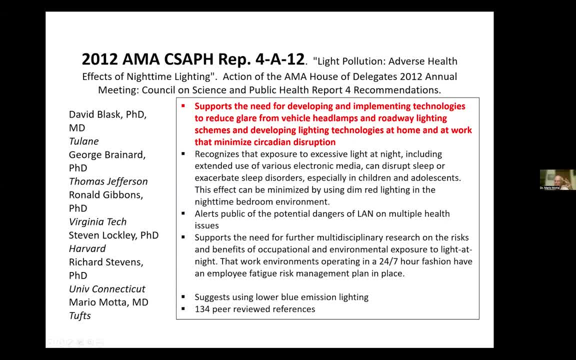 Stephens and myself. We- And I'll admit that I was mostly a editor here- These were the real researchers, But we produced this paper. It has 134 peer-reviewed references, So every word in it is proven by a peer-reviewed paper. 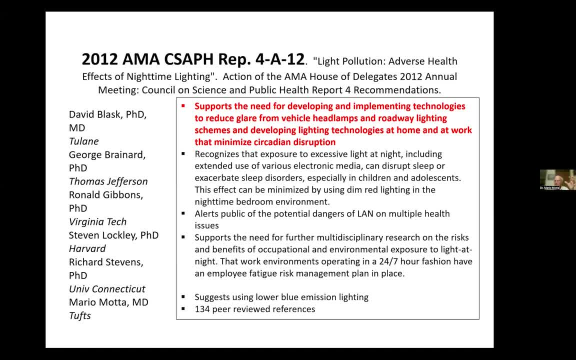 You can't get anything through the AMA, because I tried- unless it's peer-reviewed, And even then we had to go through several universities to check us for accuracy. So this is probably one of the most studied papers in history and it passed unanimously. 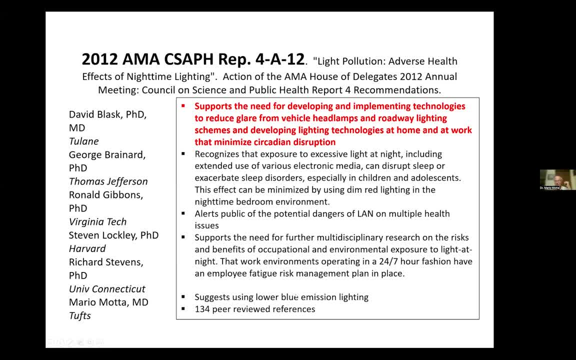 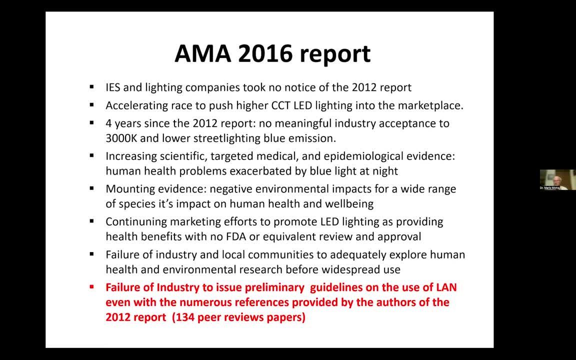 through the AMA And basically it suggested that we cut blue emission. Very simple thing, But that was ignored. The IAS, which recommends lighting for the country, basically ignored that and lighting companies like CES, Like Siemens, were basically buying up tons and tons of 4,000K lights from China shipping. 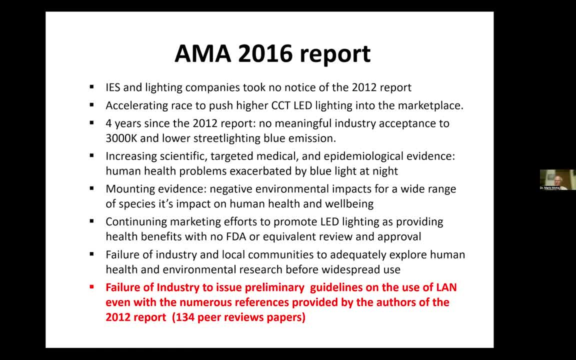 them over here and wanting to kill the market by going to city councils and saying: we'll give you these lights, you'll save energy and you'll have better lighting. Just give us the contract. So by 2016, it was clear that cities weren't getting a message. 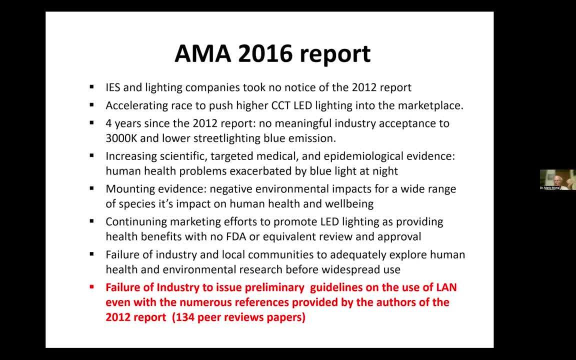 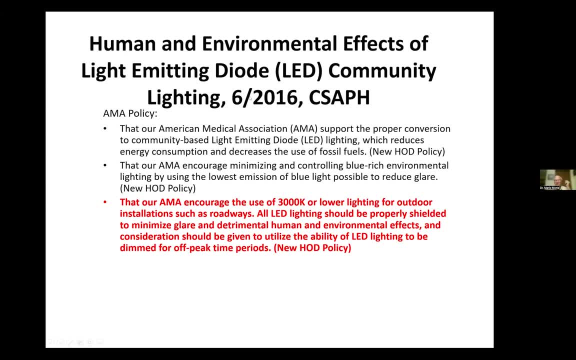 And, And Companies, Companies were doing the wrong thing, So came up with a paper in 2016, specifically designed about LED lighting, And basically it's a 36-page paper and it has, I think, 40 references. 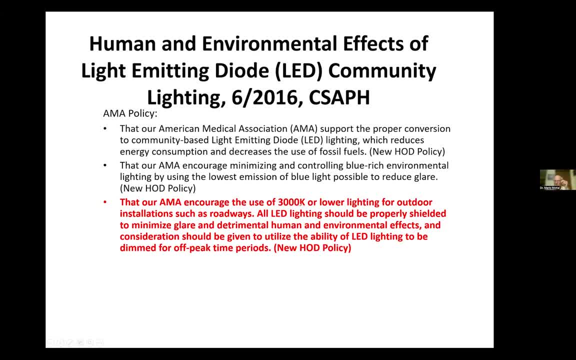 But we encouraged 3,000K or lower. The only reason it's 3,000K is 2016.. That was the best we had back then, But we didn't want cities to use 4,000K And 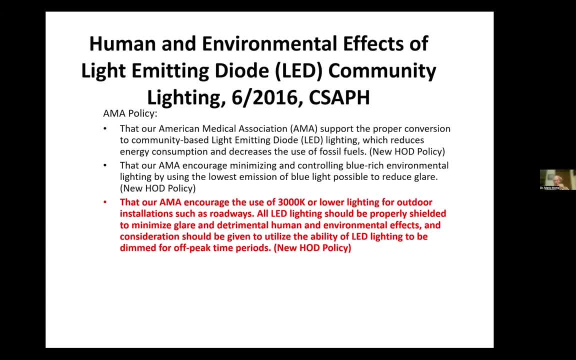 And, And And. in Chicago, a city council, because the AMA is based there, took note of that, did their own study for three months. They were about to sign one of those contracts with Siemens, a $1 billion contract to switch. 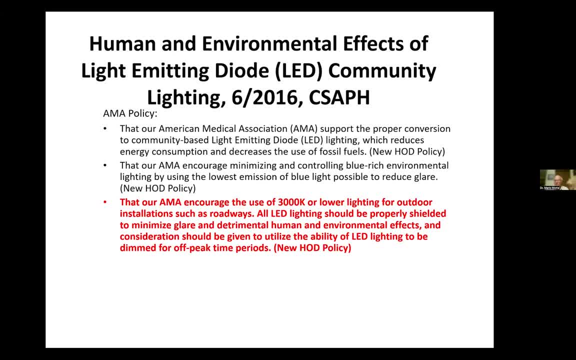 out every light in Chicago To LEDs. This came out. someone gave it to the city council, it wasn't me. they read it and said: well, maybe we should look into this. They did their own study, agreed with the AMA report. 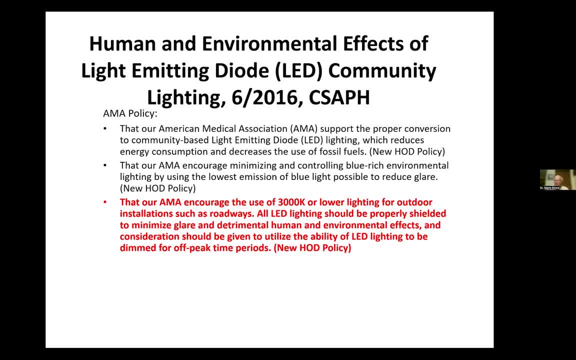 cancel the contract with Siemens, which they didn't sign yet, and ask for new contracts for only $3,000K, which Siemens didn't have To this day. if you mention my name to Siemens, you will get a very nasty rebuke with my name because they feel that I cost them a billion. 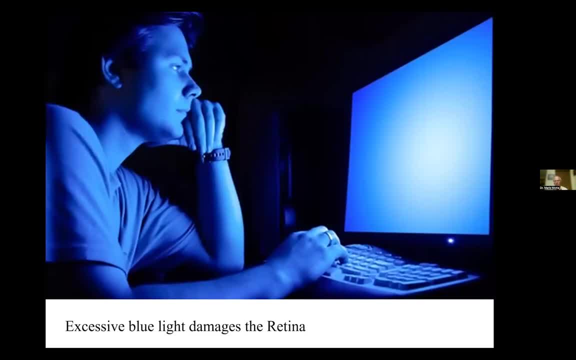 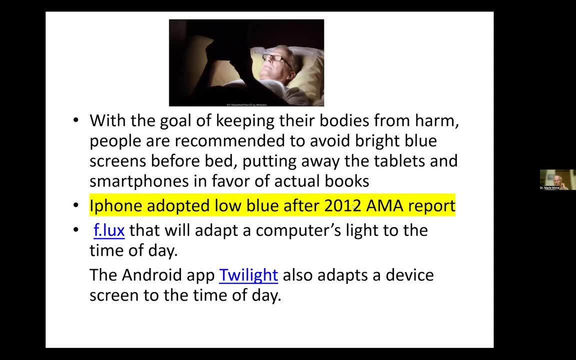 dollar contract. So let's talk about blue light. Blue light suppresses melatonin the most- Um, shortly after the uh 2012 report, by the way. that's when iPhone started dimming the night lighting, And then most uh phones now and computers now do that, And that's all because of 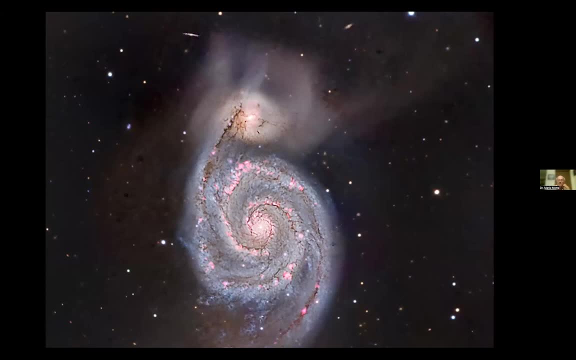 that report, I'm happy to say: uh, how am I doing? 840.. Okay, I got till nine, right, Take as long as you'd like, Dr Brother. Okay. So here's a picture. one of my favorite galaxies: M51. 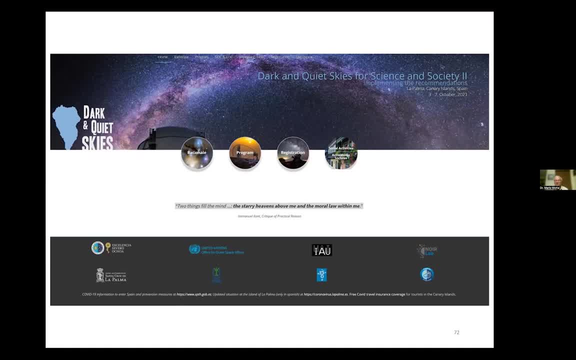 So then I was invited to be part of the UN Dark and quiet skies, which was supposed to occur in La Palma. Unfortunately, uh uh, COVID came around, And then the following year we were going to have a follow-up meeting in La Palma. 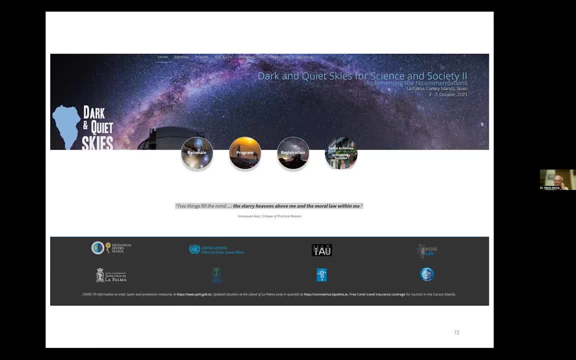 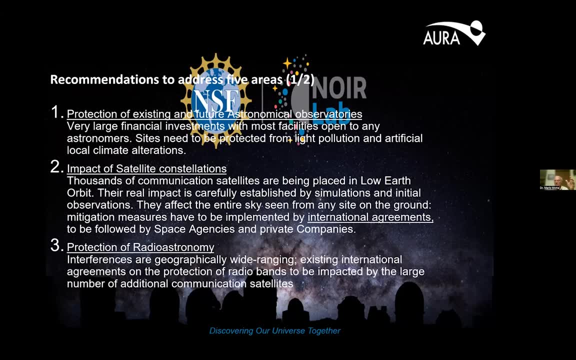 The uh uh the volcano erupted, So I feel like I was cheated, but we still got our work done. So here is the recommendations from uh, the UN advisory committee, which is in front of the UN now and hopefully will lead to a uh uh international treaty. 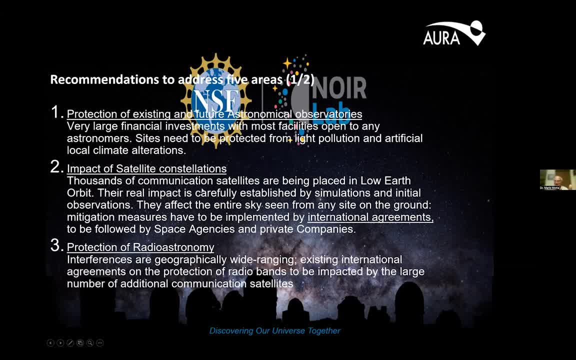 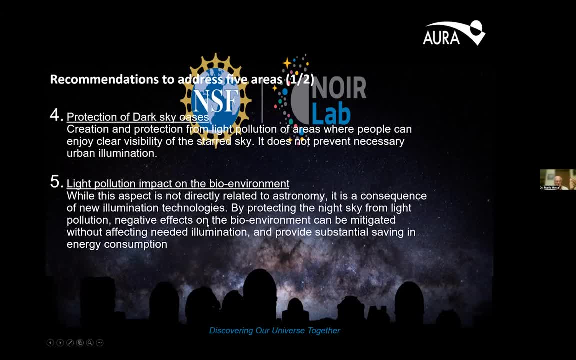 So it was primarily for astronomical observatories, satellite constellations- damn Elon Musk, uh- and protection of radio astronomy. But there was a section on light pollution in the bio environment And that's the part I was involved with And we basically 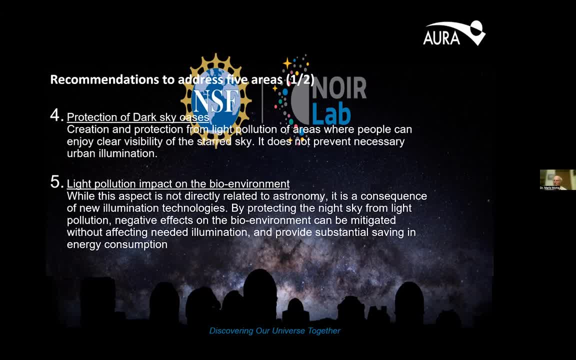 everything I say is part of the UN's recommendation. uh in front of the UN now. Hopefully that'll be an international treaty. The uh Europeans are getting way ahead of us. by the way, There are countries in Europe that now ban 4,000 K. 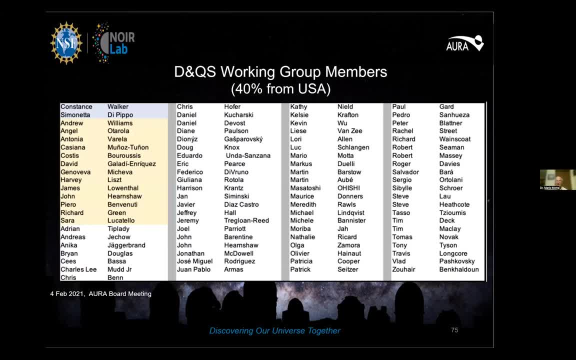 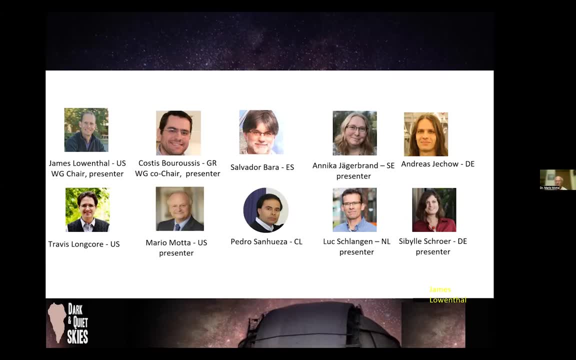 And demand shielding, like the Czech Republic. Uh, here's all the people in the UN that were, I mean in the uh around the world, that were involved with this effort. You know, this is the group that was involved with lighting. So circadian clock and clock control genes. 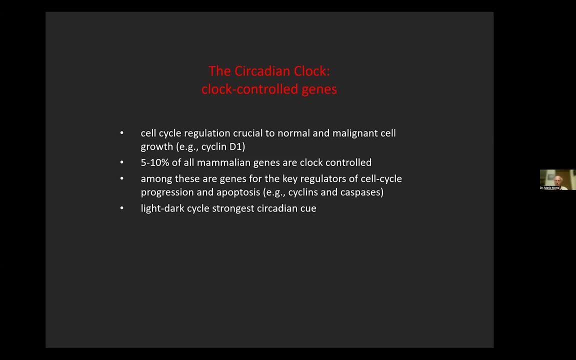 10% of our genes. a clock control- uh, control our biorhythm Okay. So it's not surprising that if you screw up a bio clock you're going to have some problems, If one out of every 10 gene is. 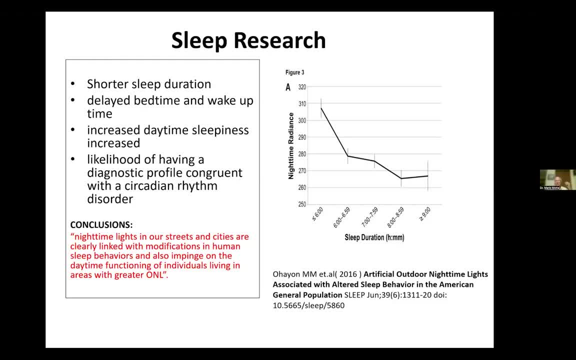 controlled by the bio clock. So the most obvious is sleep. Uh, if you have light leaking through your windows, you tend to get less sleep, And that leads to- uh turns out- obesity, uh, increase in diabetes, uh, psychiatric. 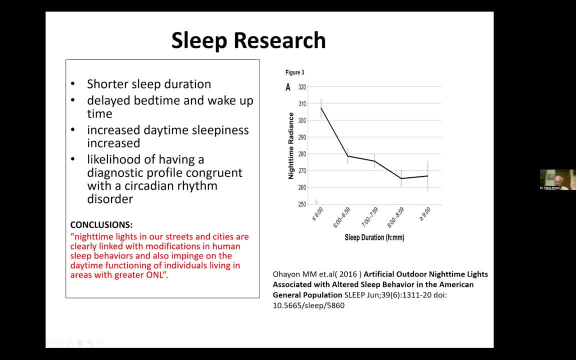 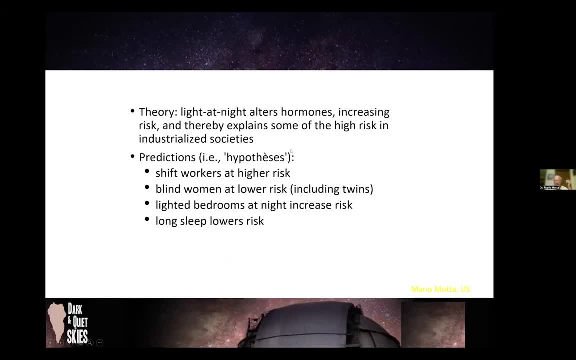 issues, bipolar disease. all that's been shown already. So then there's a theory that light at night, all those hormones and increased to high risk in industrial societies. Initially it was hypothesis, Now it's pretty well proven. So there's a theory that light at night, all those. 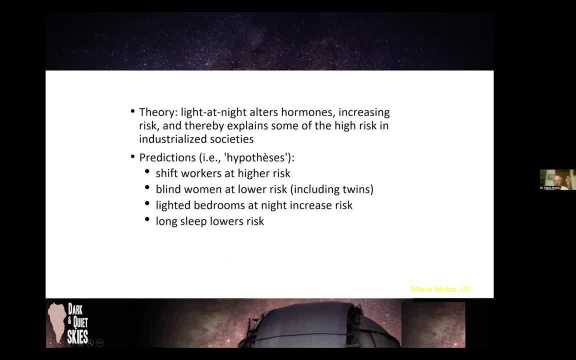 hormones and increased to high risk in industrial societies. And so the uh shift work is the hypothesis. Initially in 1990, it was shift workers should be at higher risk, That's been proven. Blind women should be at lower risk, including twins, That's been proven. I'll show. 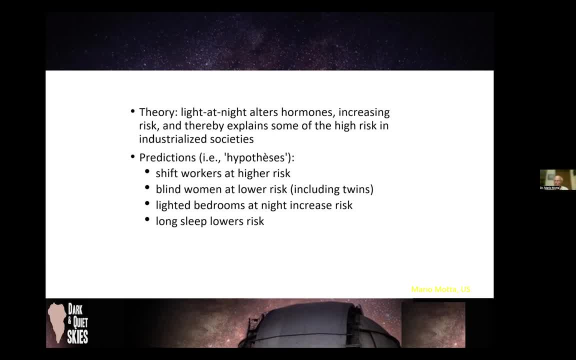 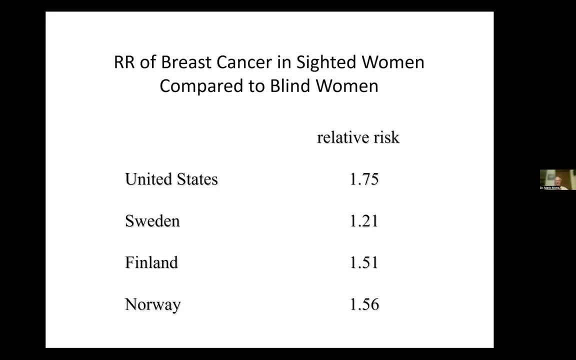 you one study: lighted bedrooms at night- increased risk, including if the light goes through the shades from a street lights. long sleep blows risk. that's been proven. So here is breast cancer. incited women compared to blind women. believe it or not, they scoured the world. This is a 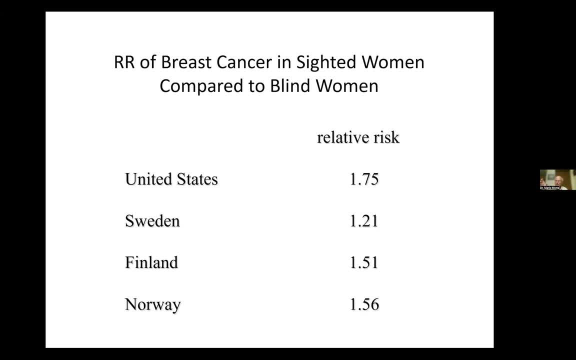 I have some evidence that there's a. there's a study that's been done by uh. the study is found twins- One woman is can see and the other one is blind- and in uh United States, uh, the one who can see has 1.7 times the risk of getting breast cancer. Then her twin sister, who does not. 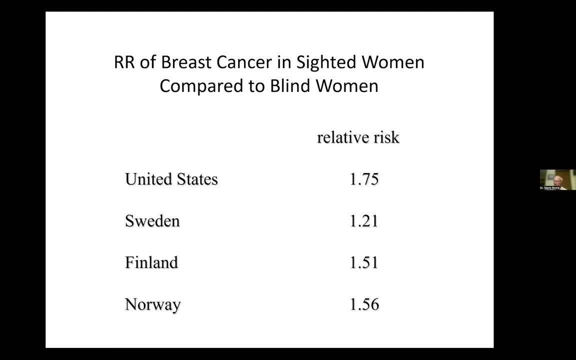 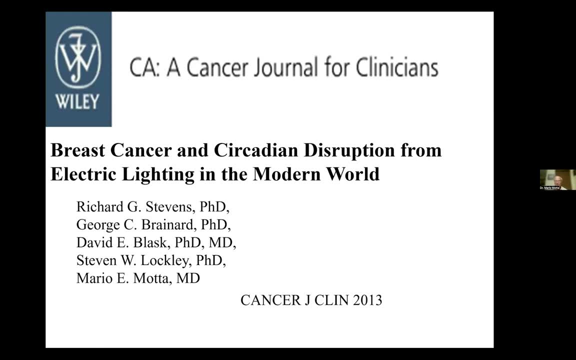 see, and that's consistent in Norway, Finland and Sweden. It was a Swedish originated study, So that's kind of proven now And then multiple studies have also shown that since then, Early on, my group of researchers put in a paper for Cancer Journal. It was one of the first papers in 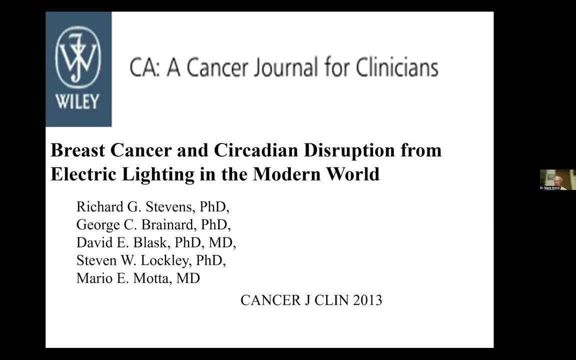 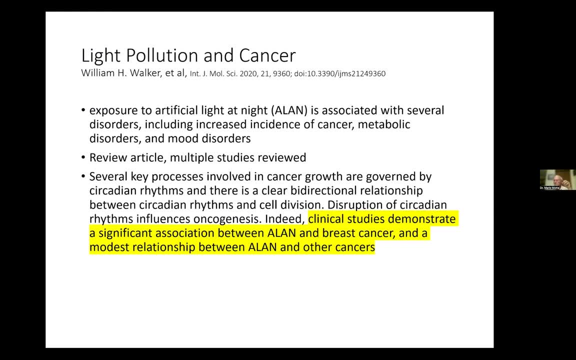 light pollution in the journal Cancer- And I'm not an oncologist, I'm a cardiologist- But since then many, many studies have been done. I'm going to list some of the studies, not because this is a medical talk, but I want to demonstrate that this is not hearsay. 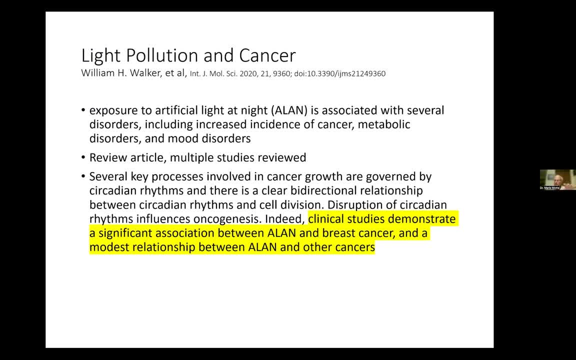 It's not pie in the sky. This is proven research now and it shouldn't be questioned, And I'll give you some studies to show that. So light pollution in cancer: Clinical studies demonstrate a significant association between artificial light at night and breast cancer and a moderate 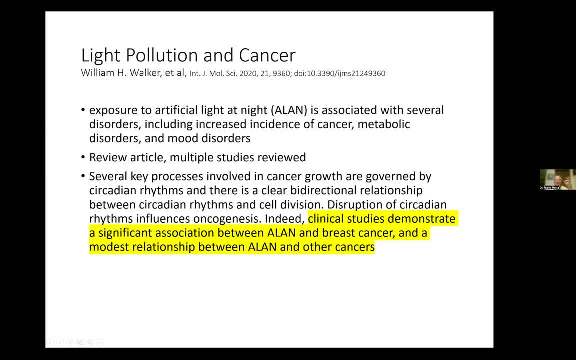 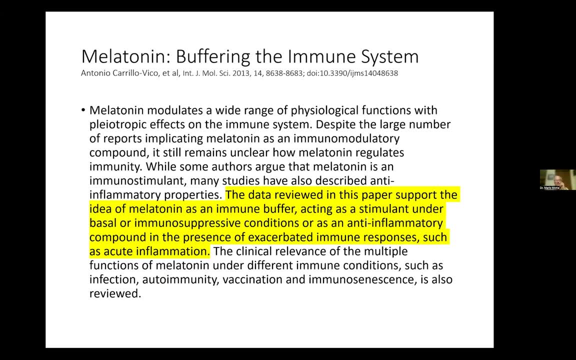 relationship in other cancers as well. This is in 2020, and this is multiple cancers that have been looked at. Then there's melatonin: how it buffers the immune system. This paper supports the idea that melatonin has an immune buffer. 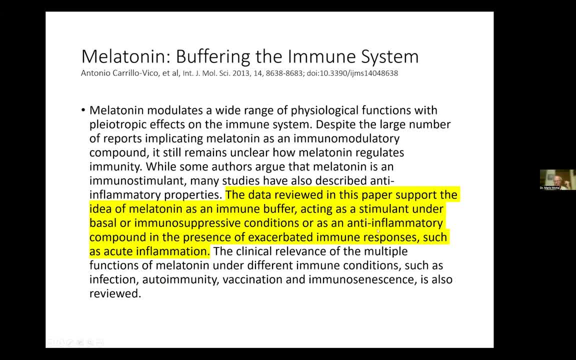 It acts as a stimulant for conditions of anti-inflammatory and immune responses, such as acute inflammation, And so melatonin is important. If you suppress it, you're going to have bad medical effects. This is again 2013.. Melatonin, immune function and age- It's more. 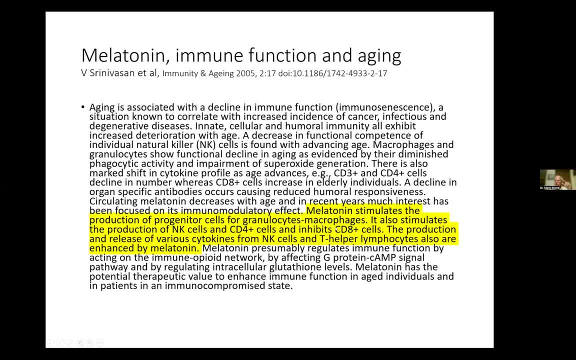 important as you age because your immune system is already on the decline and melatonin stimulates the production of granulocytes and macrophages. So if your melatonin is suppressed you're going to have a problem and higher rates of cancers and difficulties. Melatonin on the immune system in 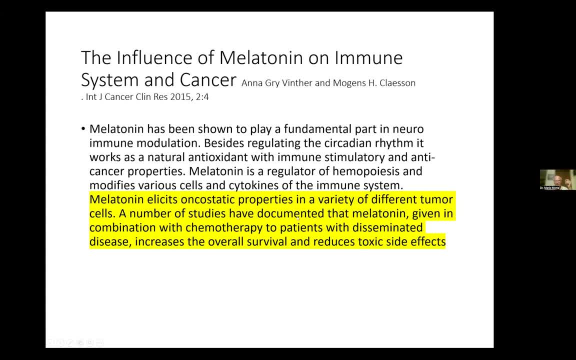 cancer: Journal of Cancer and Clinical Research 2015.. Melatonin elicits oncostatic properties in a variety of different tumor cells. A number of studies have documented that melatonin given in combination with chemotherapy to patients with disseminated disease increases the overall survival and reduces toxic side effects. So if 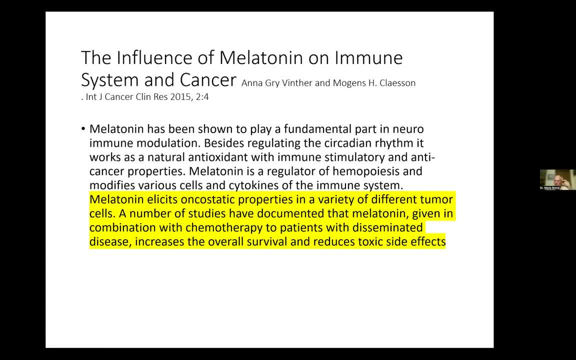 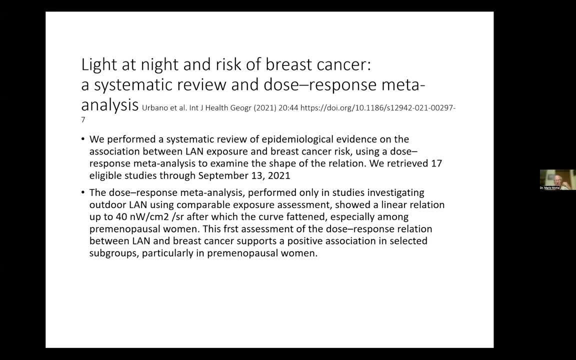 you have a cancer, it's important to make sure your melatonin stays healthy. It improves the tumor-fighting toxins that are given So light at night. and breast cancer is a systematic review, meta-analysis and, basically, demonstration. I think they reviewed 17 studies through 2021. All of them showed that there is a linear 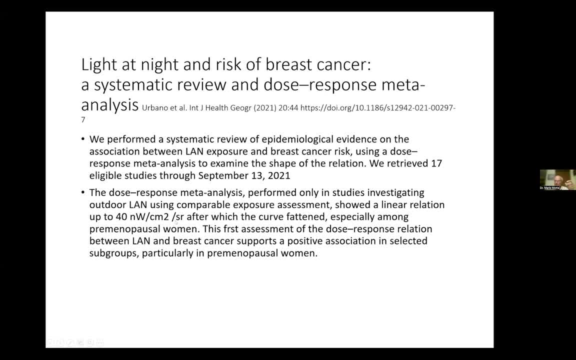 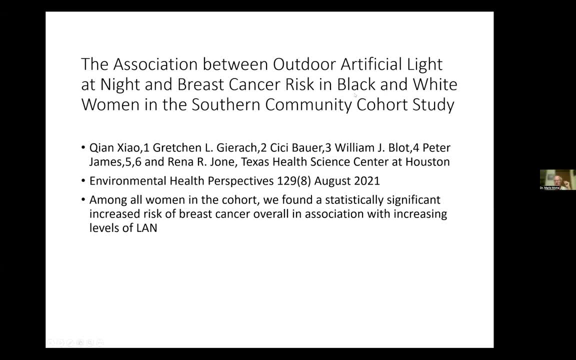 relationship between excess light at night and cancers, Outdoor light, night and breast cancer in Black and white women. in Southern Community Code study it's even more important in Black women, it turns out. So here's one of my favorite studies, mainly because it was spread out in. 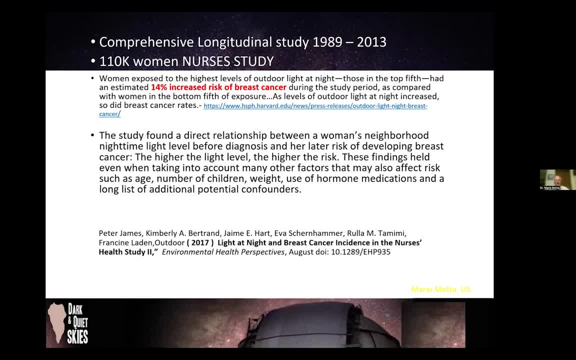 the United States and I was here at Harvard and I had some mild input into it. This was followed: 110,000 women from 1989 to 2013.. And these women were divided up into five quintiles based on their zip code. The lowest quintile was in a more rural area, The highest quintile was in Central City and 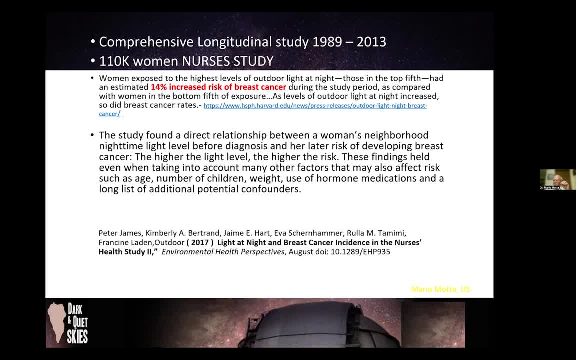 everything in between. And then they correlated that with satellite photos showing in that zip code how much light pollution there is And it turns out the difference between the lowest light polluted area and the highest. there was a 14% increase in breast cancer, And that's a lot of women, so this is a pretty good. 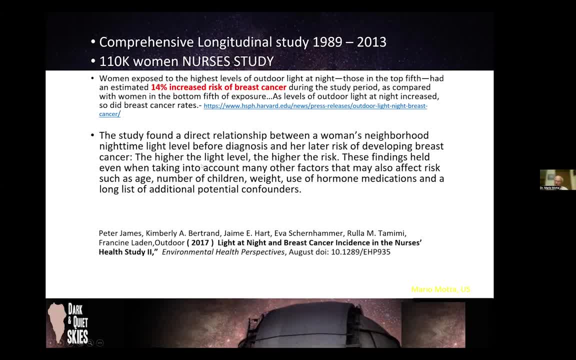 and well-documented study, And they took into account every other factor that they could. by the way, Now don't get me wrong- 40% of breast cancers are by the BRAC gene, and there are other factors as well, But a 14% increase for the rest is quite significant. Now, if you think this is just one, 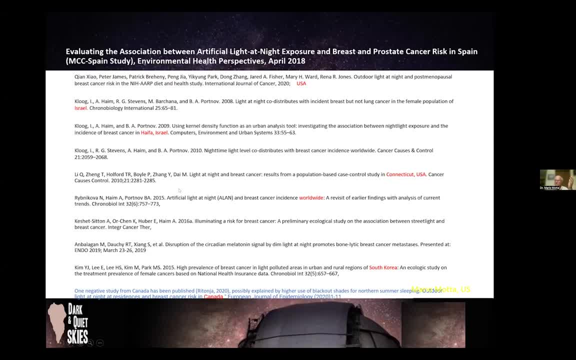 study here. there are 20 other studies that have reproduced that study. Best one is from Spain. There's one from International Journal of Cancer. Let's see, this was well, let me see. uh, there's one from Spain, there's one from Israel, one that tried to do a worldwide study. 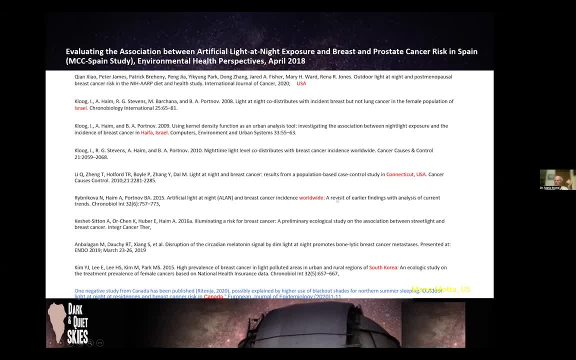 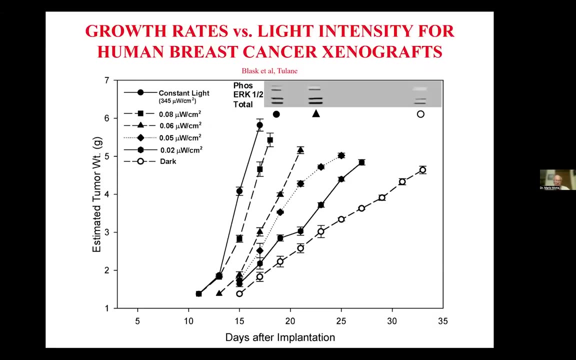 South Korea, one specifically to Connecticut. So 20 studies have reproduced that study. When you have 20 studies that all show the exact same thing, you can't dispute it anymore. One of my favorite studies goes back to 2003 by Dr Blask at Tulane. He's a great. 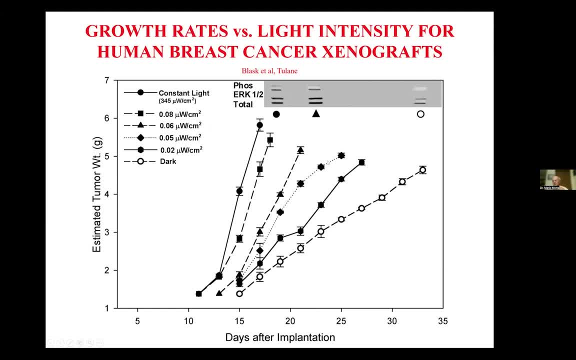 researcher and he's a basic researcher. He took 120 nude mice. nude mice, take their bred mice that allow transplants. So what he did is he transplanted, uh, human breast cancer under the skin of these rats and then subjected them to a normal. 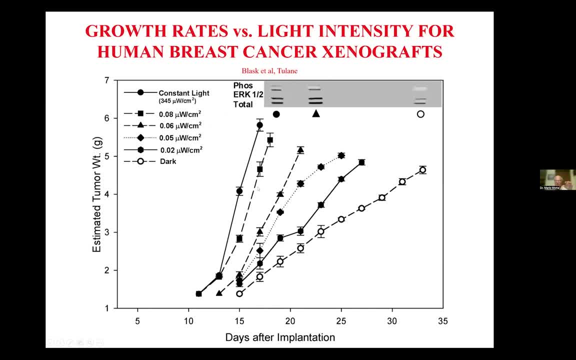 daylight cycle or increasing amounts of light until there was light on all night long. if that's right, It was eight days of care at the Western constrains channel for doctors with research. So they recorded that síclox in the crossUSR and his teeth combined And he took a 127-new mice- nude mice, take their bred mice coming from tons, unlike other situations. So what he? 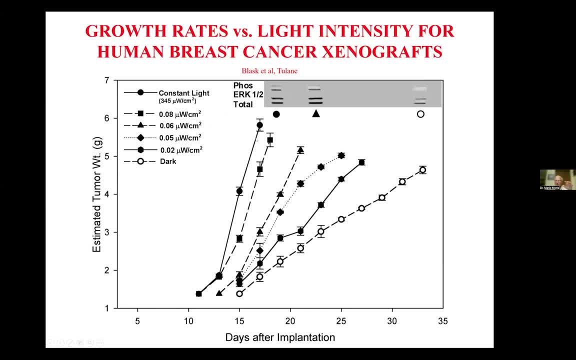 did is he transplanted human breast cancer under the skin of these rats and then subjected them to a normal daylight cycle or increasing amounts of light until there were light on all night long, or these paths. there was light on all night long at full intensity. and lo and behold, what did he found? 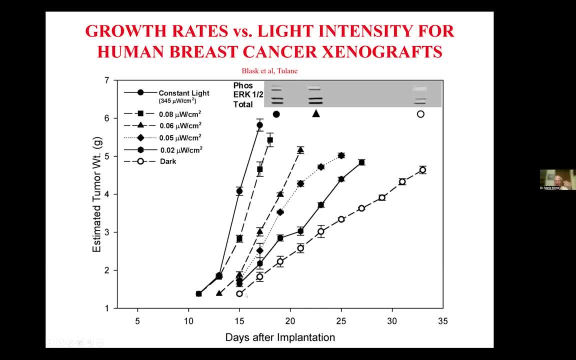 at 30 days. uh, the ones that had a normal daylight night had this steady rate of cancer growth that was implanted a little bit of light. this is minimal, uh: 0.02 watts per square centimeter. that's the amount of light that goes through your shades at night if you live in a city. 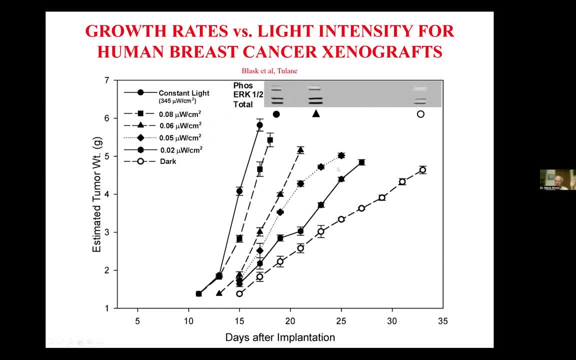 they had this rate of breast cancer growth a little bit more light, higher rates until finally, if you kept the lights on all night long, uh, the poor little rats, the- uh, the tumors basically exploded out of their chest. so you can't do this experiment on humans, you have to do it on rats. 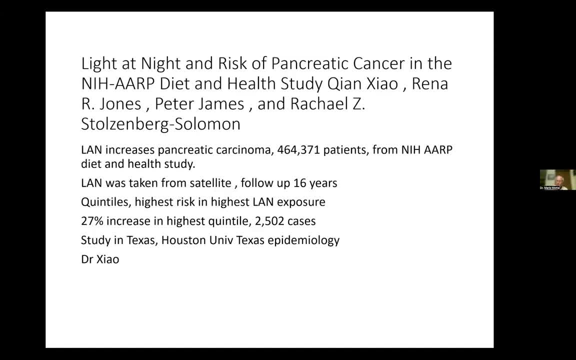 but I think this is pretty indicative of what can happen. so there are other cancers. I know Dr Zhao is in the audience. I picked her studies to highlight. uh but uh. right there in Texas you have a great researcher who's highlighted increase in pancreatic cancer. um and uh. and the NIH diet and health study. okay and also is correlated with light at. 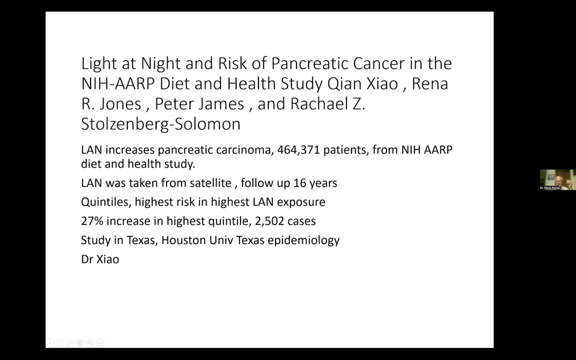 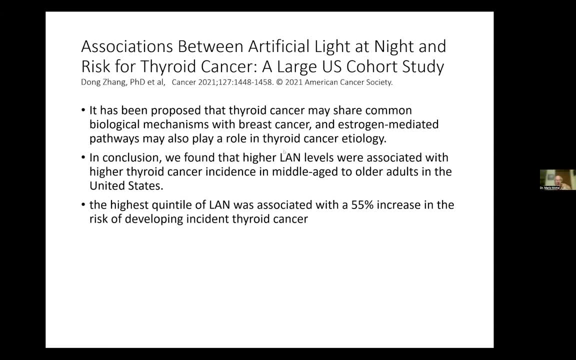 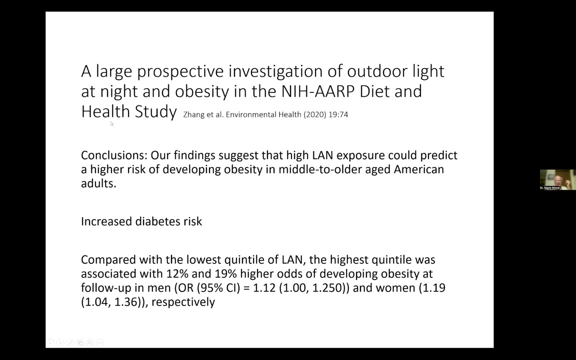 night from satellites followed for 16 years. they also divided up into quintiles, so a 27 percent increase. that's pretty significant. artificial light and thyroid cancer also- Dr Zhao was in this, I believe. anyways. uh, it showed thyroid cancer increases as well. outdoor light at night and obesity: uh, in the NIH diet and health study: increase obesity increases. 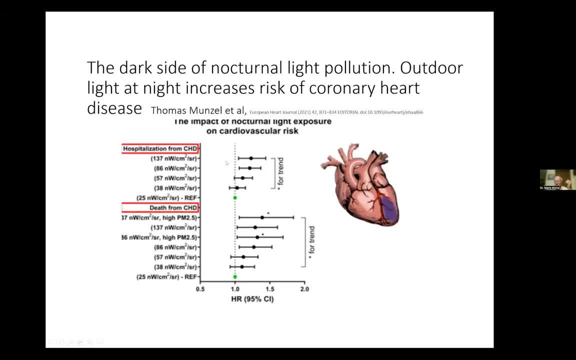 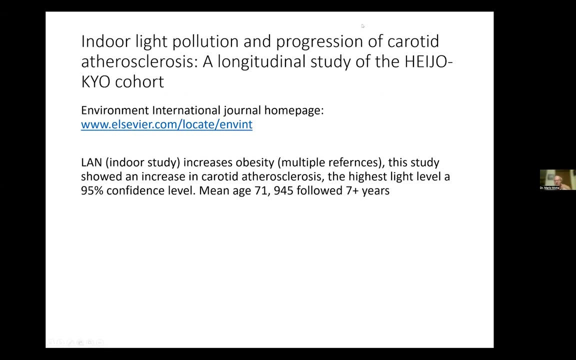 and whenever you have an increase in obesity, you have an increase in coronary disease and diabetes. okay, I'm a cardiologist, so this study I've looked at. it's from the Europeans 2021 European heart study. uh, indoor light pollution. I haven't seen one for outdoors yet. 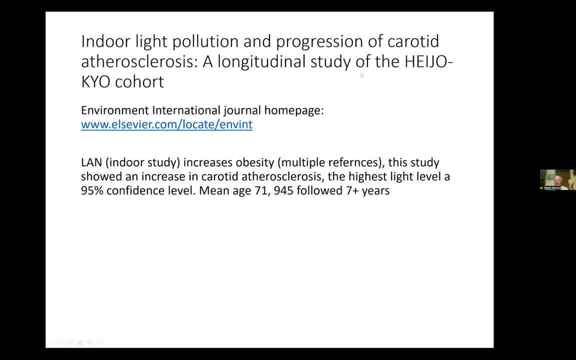 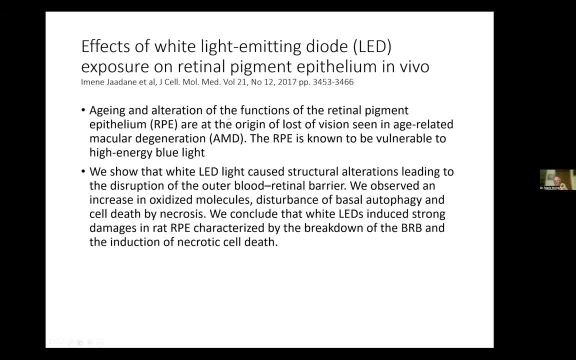 for carotid atherosclerosis. but if you keep that in mind, you're going to have a lot of, you're going to have a higher rate of atherosclerosis and strokes later in life. white light emitting on retinal pigment. so let's talk about something totally different. 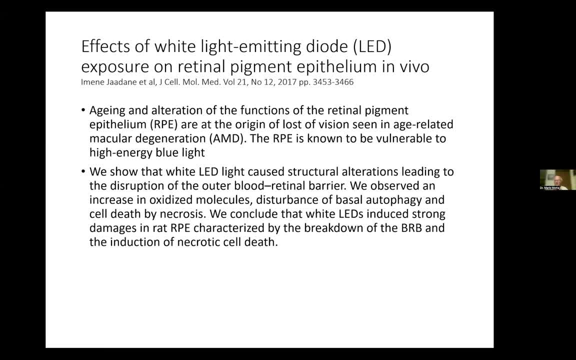 um. high intensity light and blue light damages the retina and if you're exposed to that on a regular basis, uh, you can. you have retinal damage. multiple studies have shown that, and it increases the amount of age-related macular degeneration. so that's another reason to cut down the blue. 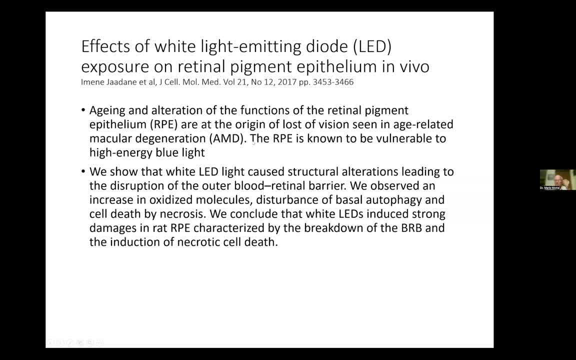 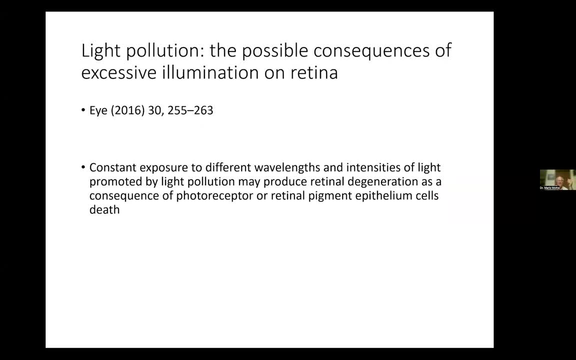 because blue increases the rate of macular degeneration and the rate of retinal damage much more than red possible. there's another study showing the same thing: different wavelengths, but blue is the worst. this is ngc6781. it's a very nice planetary nebula. 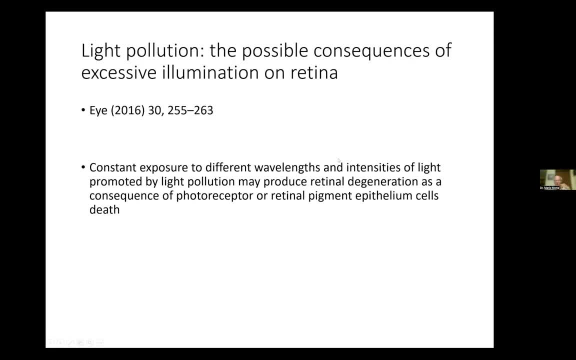 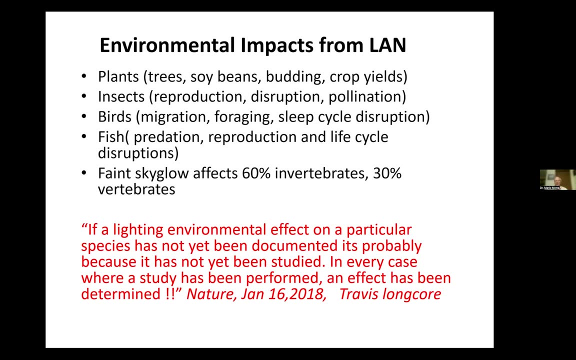 so constant exposure to different wavelengths of light. this is in the journal eye again. excess light, excess blue, and you end up with worse retinal damage later in life. I must have gone the wrong way. sorry, environmental impacts of land. I won't spend much time on this. 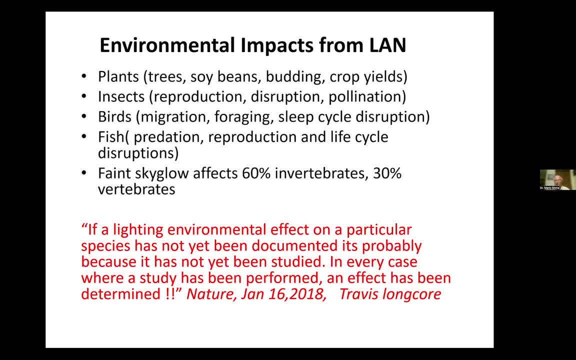 I was getting short anyways, but I just thought I'd point out that humans are one species on earth. every species on earth is affected. one of the best researchers is from California Travis Lancourt University of California, Southern California, and he's documented multiple studies that have shown many different species get affected. in fact, in nature 2018, I love this. 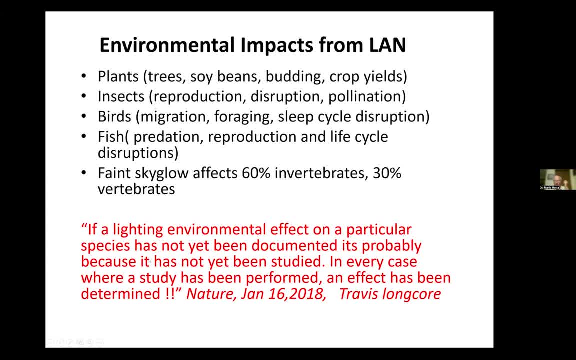 quote. I use it a lot. if a lighting environment effect on a particular species has not been documented, it's probably because it has not yet been studied. in every case where a study has been performed has been determined. I can't think of a stronger statement. basically, he's saying that if you don't, 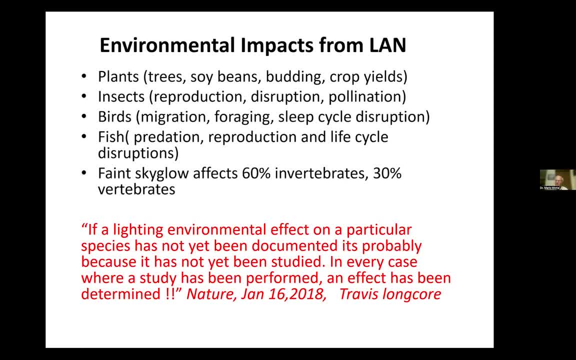 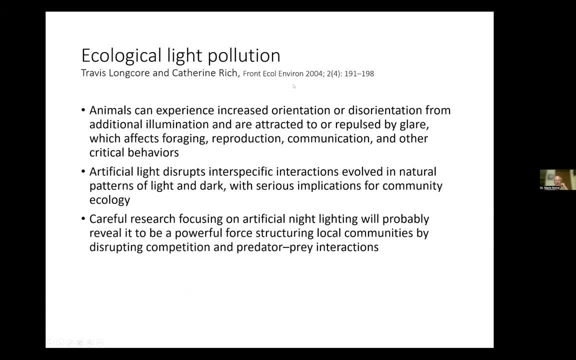 know the species has been affected by lights because no one studied it yet. every time he studies it there is an effect. so light pollution can affect animals, different species, insects, and artificial lighting effects our general environment. so there are many species that have been affected by lights and artificial lighting. 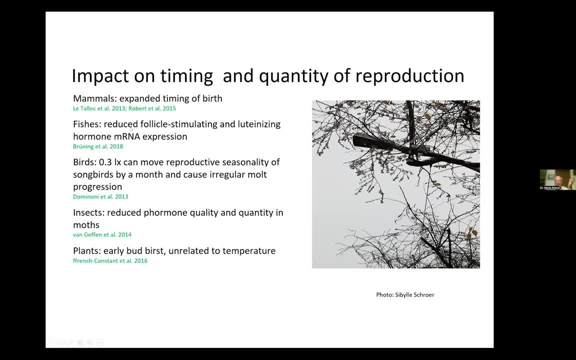 studies mammals. it changes the timing of birth. fishes reduces follicle stimulating and luteinizing hormone. birds: 0.3 Lux, which isn't a lot, can move the reproductive seasonality of songbirds by a month. interfere with their mating insects reduce pheromone that should be pheromone quality. 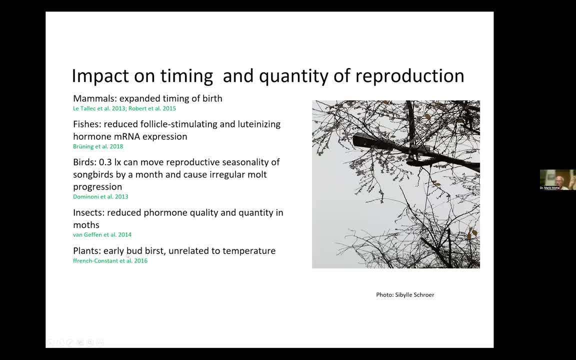 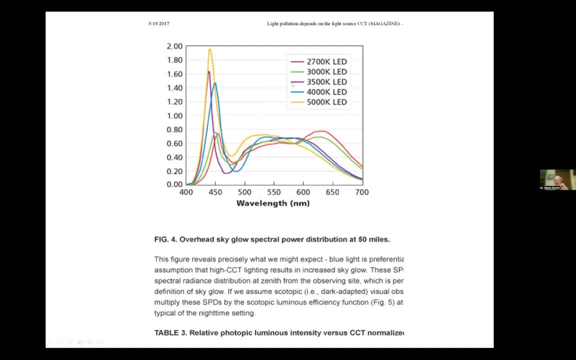 and quantity. in mods plants early bud bursts unrelated to temperature and then they die. so here's the problem with the high blue LEDs. this is from 50 miles away. the 4000k, 3500k and 5000k spread horizontally much more than. 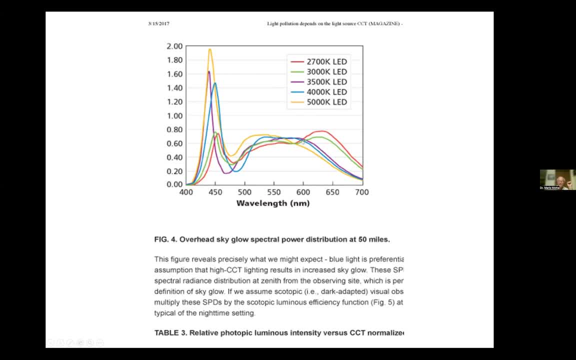 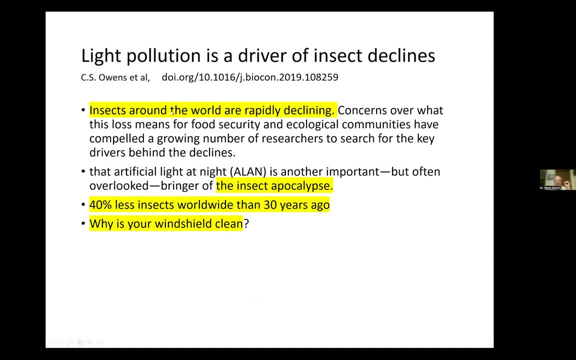 the the warmer wavelengths. light pollution is a driver of insect declines, so this is by Owens. insects around the world are rapidly declining, and we're in fact. many entomologists are calling it an insect apocalypse. right now, there are 40 percent less insects worldwide than they were 30 years ago. let that sink in we're. we're essentially 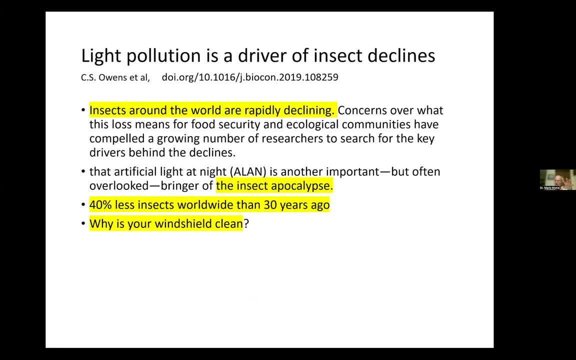 creating an extinction event. now, some of that's due to insecticides, no question. a lot of it's due to lights, because many of the good insects we don't want to kill are also being killed. in fact, there was a lecture I attended a few years ago and I love the title. 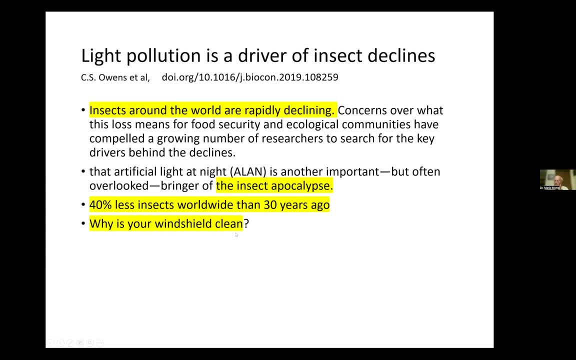 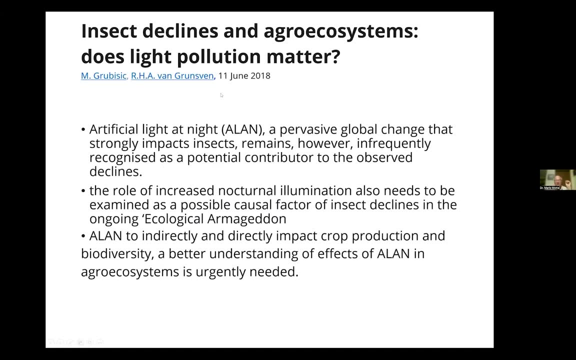 why is your windshield clean? I remember as a teenager driving and insects were always splatting on my windshield. hardly ever happens anymore. we've already killed them all off. is the reason why the windshields are staying clean. insect declines, this light pollution matter as you kill. 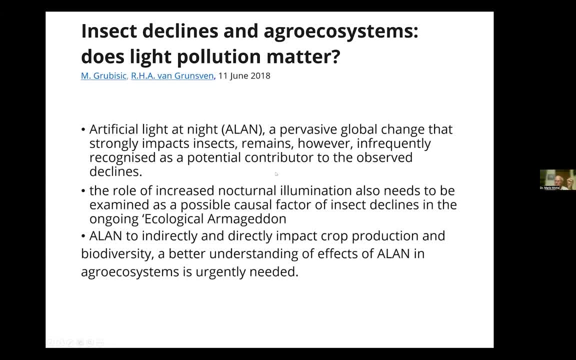 off the insects. it causes a decrease in pollination and decreases agriculture as well. because of that, to understand why so many uh communities need to now bus a truck in bees in order to pollinate their plants, because we're killing off all the local insects. this is an extreme example that this is. 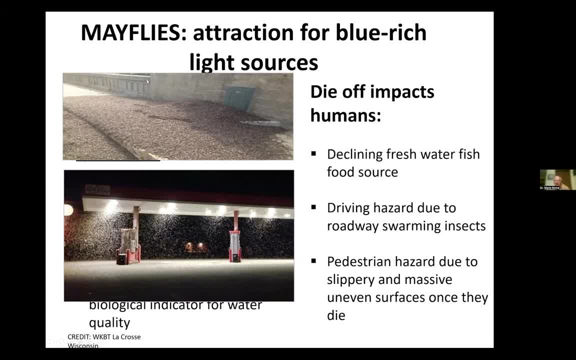 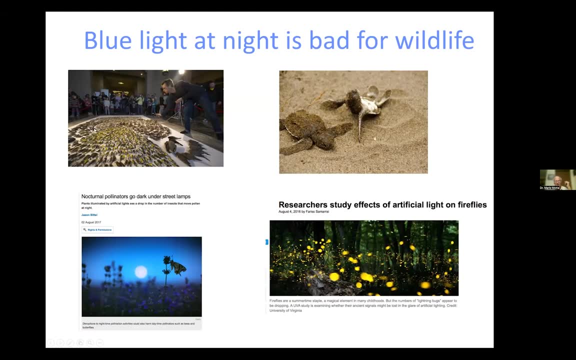 over the Susquehanna River mayflies. they should be going along the river mating. instead they attracted the light and just dying in place. okay, all these are fish food that are no longer food for the fish, which are now starving. we're killing off insects- I mean birds- at an alarming rate because of light pollution. 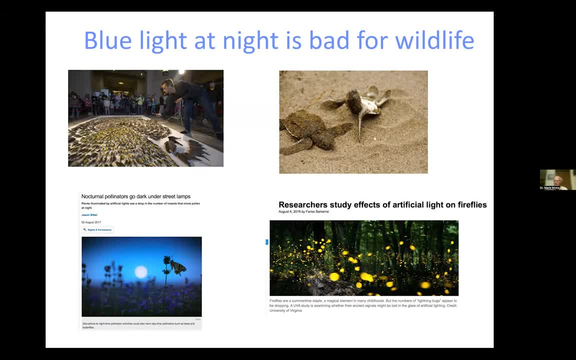 turtles in Florida. I don't know if you remember 25 years ago everyone thought the turtles were dying off because of local uh toxins and pollution. well, took a researcher from Atlantic University in Florida and he realized: no, it's the lights everyone in Florida loves to, for some reason. 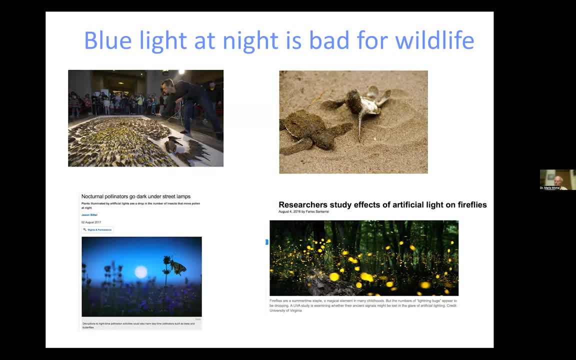 put on their lights and shine up the beach and the waves come in. and even when they're in bed, turtles hatch at night and go by the Moonlight to go out to sea if they have bright lights. instead of going out to see, they go out to the street and they don't make it to the sea and 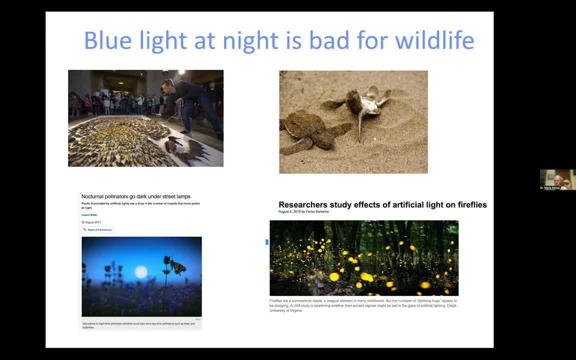 die. so they did pass a law in Florida, one of the few environmental laws actually passed. but now you can't shine your lights on on the light all night long and the turtle population, Behold, is coming back um. the uh, the uh. fireflies used to be. 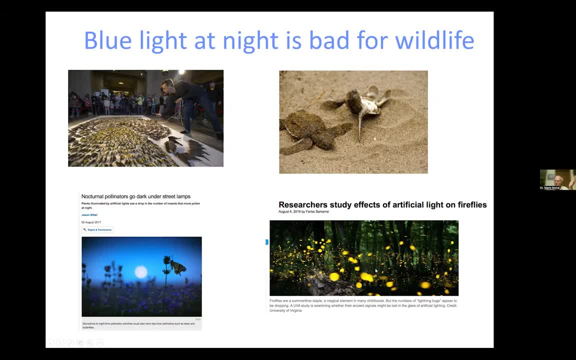 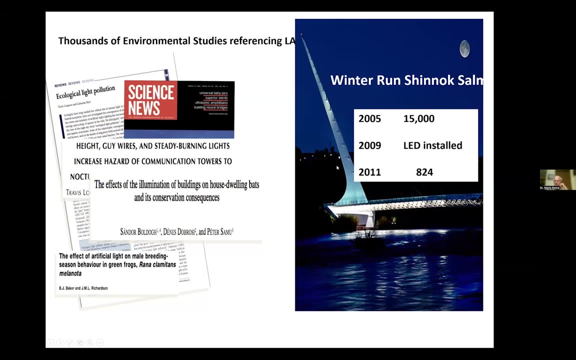 very common. They're getting rare, except in rural areas. If the female and male fly can't see each other because of light pollution, they don't mate. You have no baby fireflies. Here's one of my favorite examples. This is in Northern California. There is a bridge that goes across a river. This 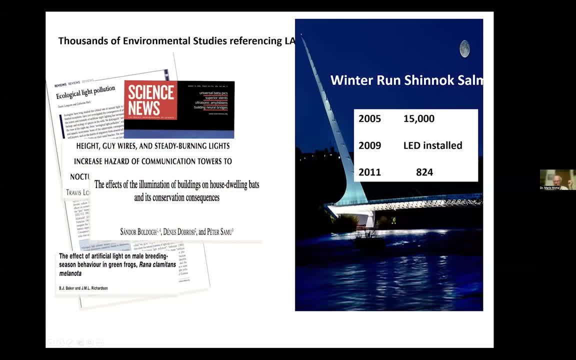 is near the Oregon border And some bright souls- here's the pond- decided it would be great to light up underneath the bridge. It's way from 10 miles away. You can see it- even though it has nothing to do with safety and crossing the bridge. So they put up these lights: 4,000 K lighting up the. 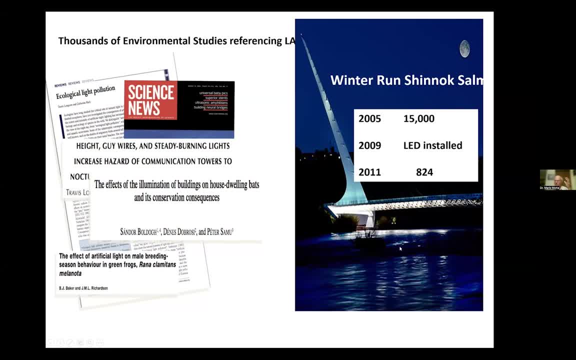 water Salmon used to run up here. It turns out salmon don't like the bright light and they stop right here and basically don't run upstream And it took them five years to figure it out until when the LEDs got a few years. basically the salmon run. they basically got them wiped out. 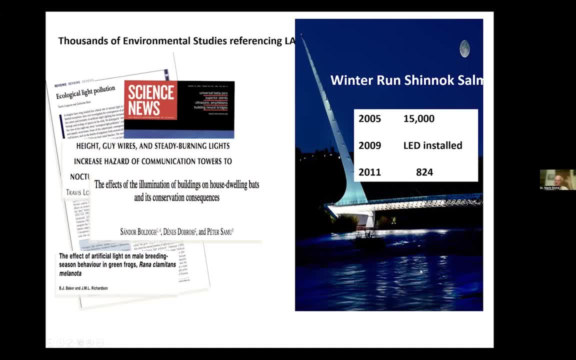 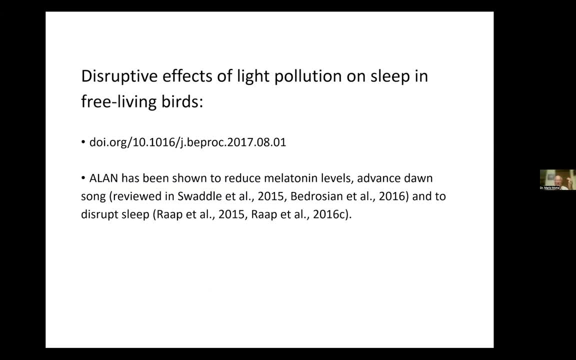 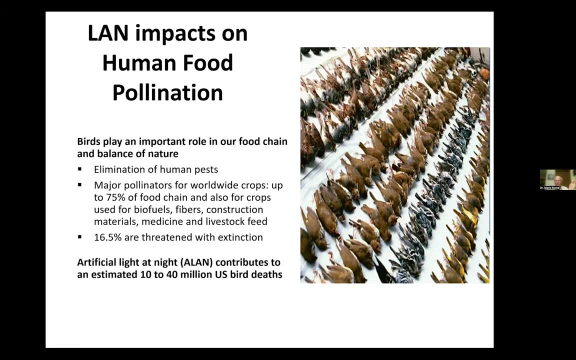 They finally turned them off for two months while they're running and the salmon population is coming back. So every species is affected, even the ones you wouldn't think about. Reduced melatonin in songbirds affects them as well. Human food pollination is being affected. We need pollinators. 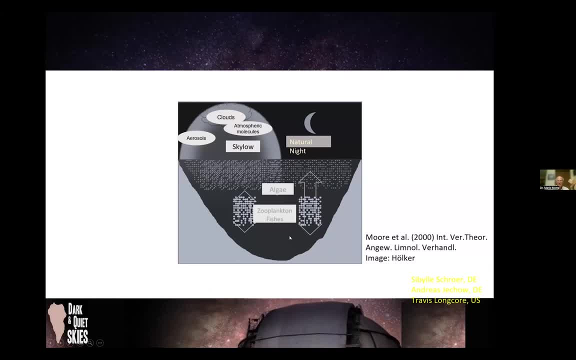 for 75% of our food. And then here's one that you wouldn't expect. We've all heard about algae blooms in Florida Now, most of the algae blooms because of runoff from agriculture, No question about that. But here's something that's not well known: Algae get eaten by zooplankton. The zooplankton will not come. up when there's light, So they stay in the depths below 300 feet. But there's a migration. every single night Zooplankton come up and eat algae. But along the shore, when you have light pollution, the zooplankton either go somewhere else. 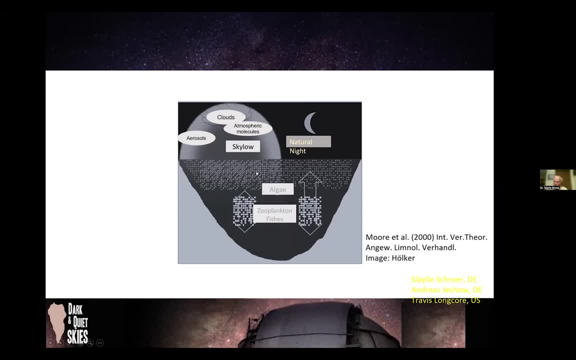 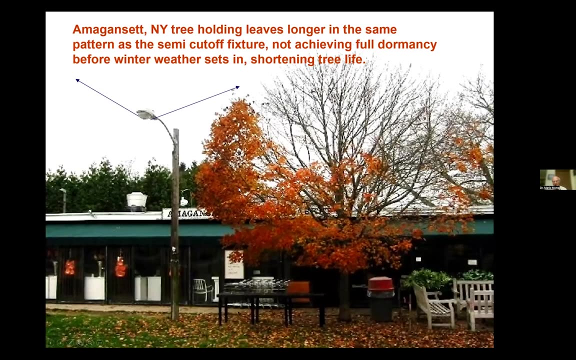 don't come up and eat the algae, which, again, not the root cause of the algae bloom but contributes to it. Again, things that you wouldn't think about cause environmental damage. Trees are affected. Here's a tree that's lit up pot waste So it thinks it's summer fall. here. 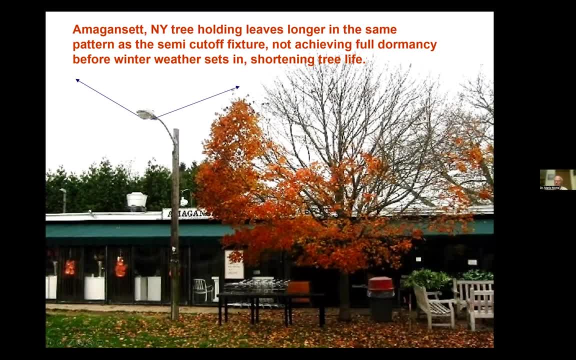 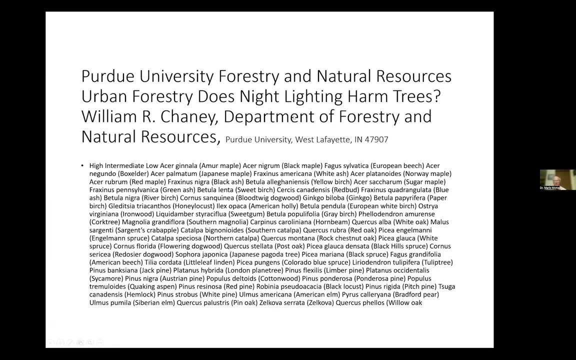 Here it thinks it's winter And when the tree is stressed this way, trees die 50% faster. And here's a study from From Purdue University: Does light at night harm trees? I won't. basically, instead of putting in: 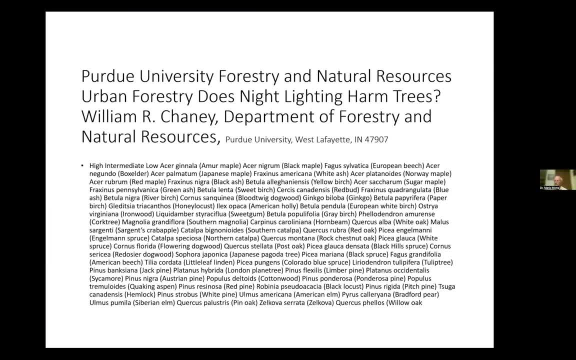 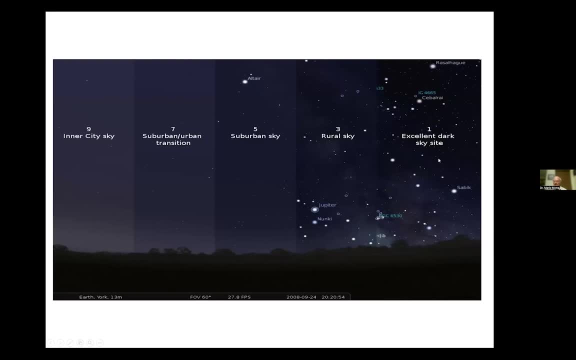 the conclusion I put in the name. Sorry about that, But basically the conclusion is: excess lighting harms trees and they die about 50% to one-third faster if they're exposed to lights at night. And finally, just the aesthetics: Who would rather live here rather than here, which most of us 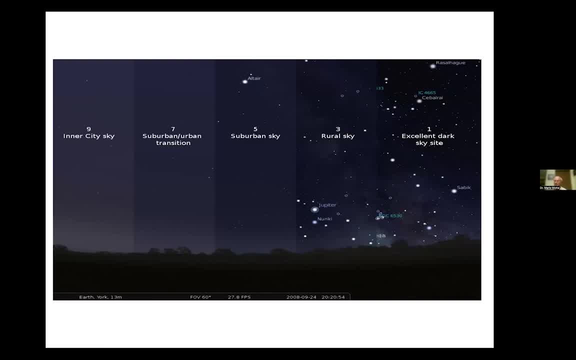 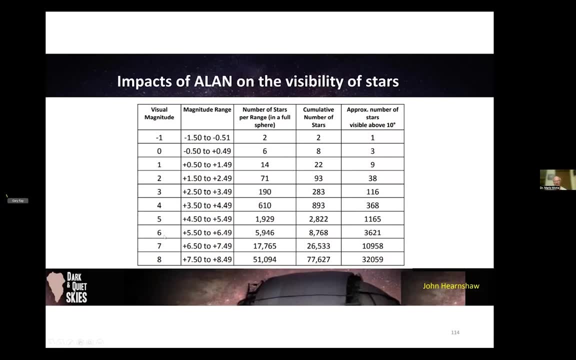 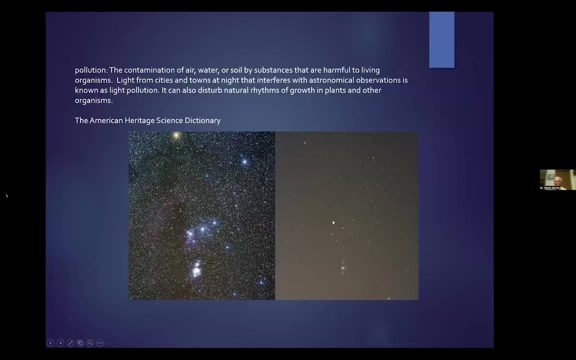 unfortunately now do. We've lost the beauty of the night sky And if you're in a true suburban environment- not suburban but rural- you see 6000 stars in the sky. Most cities are down to 14 to 70 stars. I would rather see this than this, personally, And many people have never seen the Milky Way. I think that's what we're doing. you're down to 14 to 70 stars. I would rather see this than this. personally, And many people have never seen the Milky Way. I think that's the biggest thing to add to that. That's it. So can you help me? 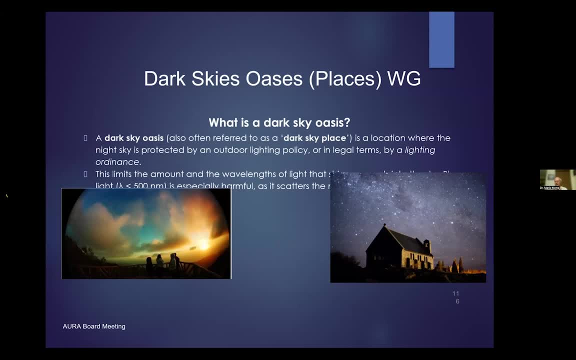 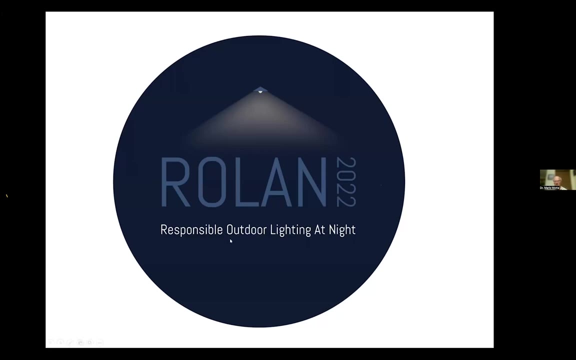 I don't know Any other questions. Absolutely Yeah, that's an abuse. One of the UN results was that we should save dark sky oases for the beauty of it and to allow people to see the night sky. I agree with that. This is a yearly meeting. 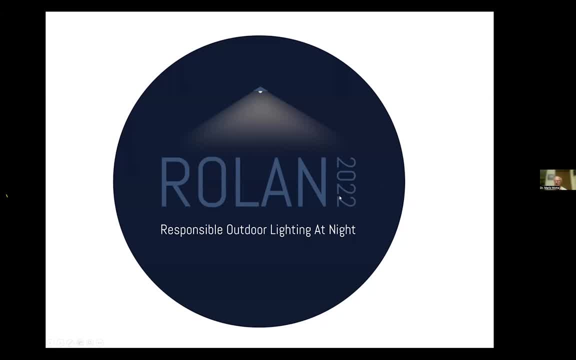 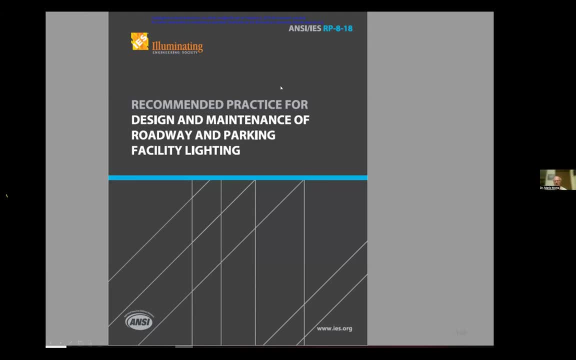 rolling from Europe responsible outdoor lighting at night. I contribute to that, and again the Europeans are ahead of us. The IES was fighting me for years. They finally- their last one that came out, their booklet finally agrees that blue light's not good. So here's the problem, though. 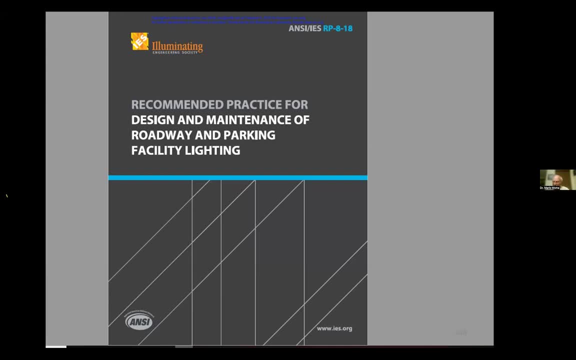 Most lighting engineers have no lighting degree. This is a sorry fact. There are only five universities in the country that give a lighting degree, So many people who have other degrees that have never taken a class in lighting will take a job as a lighting engineer. 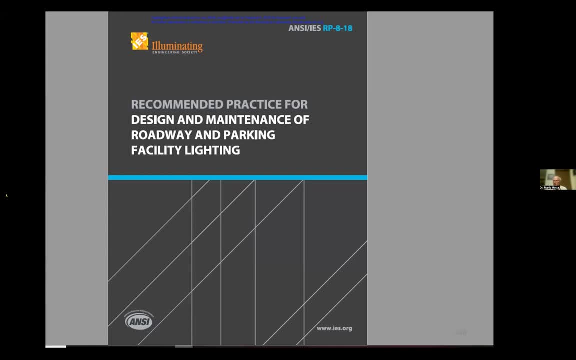 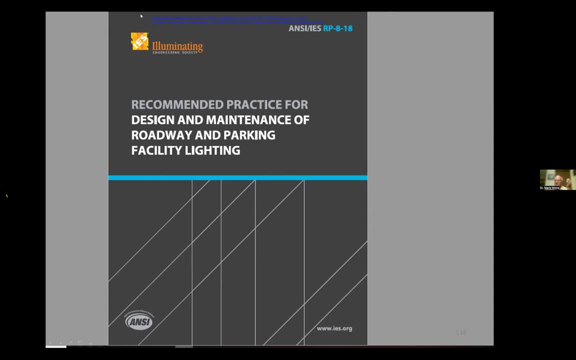 you and I did. But the IES gives them a handbook. and the second problem is, if they say, well, I'm using the IES handbook, ask: what year, what volume are you using, If you're not using the latest and many of them, because this costs 250 bucks or something and, like most of us, you're using. something that's 20 years out of date, If you're not using the latest and many of them, because this costs 250 bucks or something, and and, like most of us, you're using something that's 20 years out of date If you're not using the latest and many of them, because this costs 250 bucks or something and and, like most of us, you're using something that's 20 years out of date. 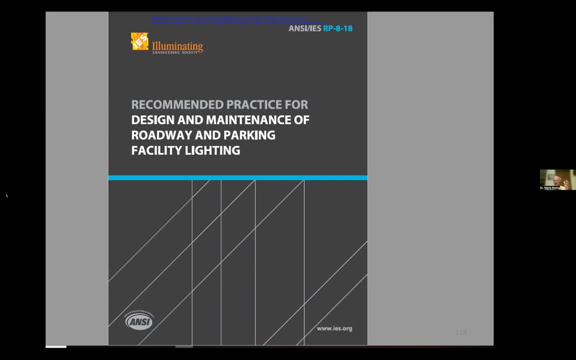 I've embarrassed some engineers at town councils. I simply ask which volume you use and they said 20, 20, 20, 2003, something like that. I says: well, why don't you buy the latest? and you'll find out that everything you just said is completely wrong. 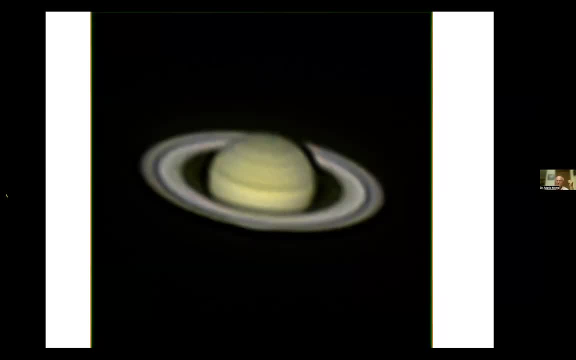 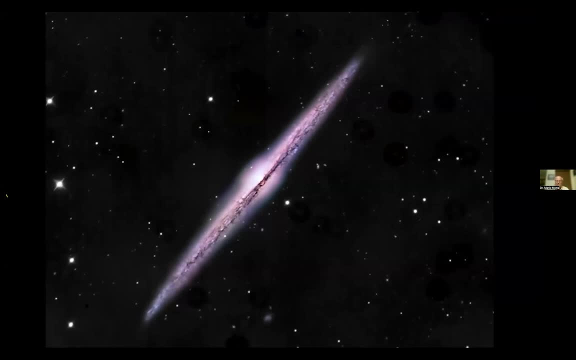 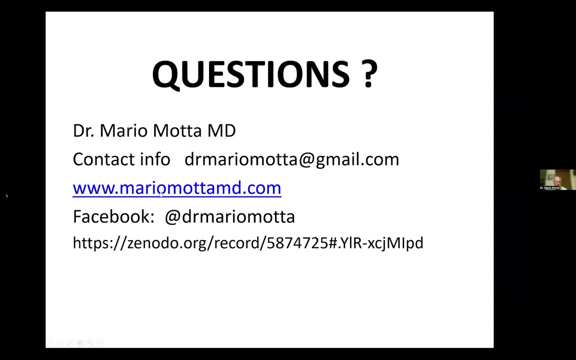 So use that in some town meetings- This picture of Saturn I took- and NGC 4565, which is one of my favorite galaxies, And I'll stop there and ask any questions. If you go to my website, wwwmyramadamdcom, you have many studies that you can download, but 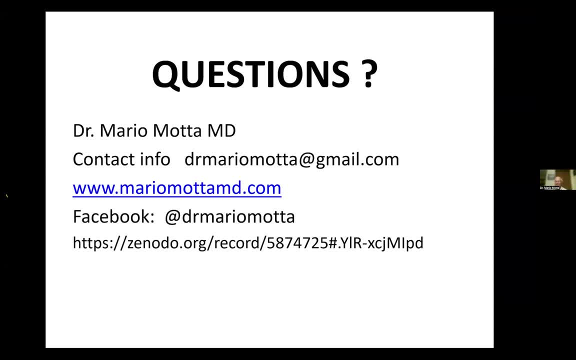 these are very available these days, so any questions I can answer. Dr Mata, thank you so much for that wonderful presentation. It's quite sobering to see just how wide-ranging the effects- of you know, something as simple as lighting could be on on so many different ecosystems. 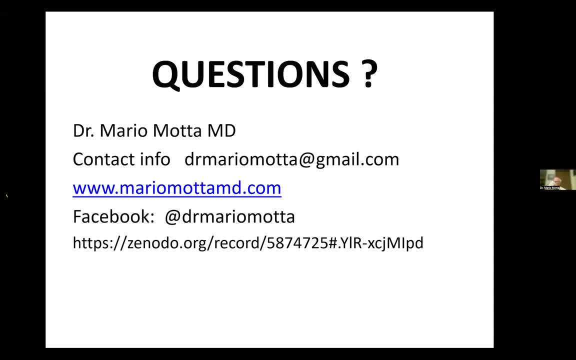 Not just limited to to. you know our own hobby here in astronomy, So thank you for sharing that. We did have a number of questions in the chat here. I'd like to get to those in order that they were presented. Do you have a few minutes for those, Dr Mata? 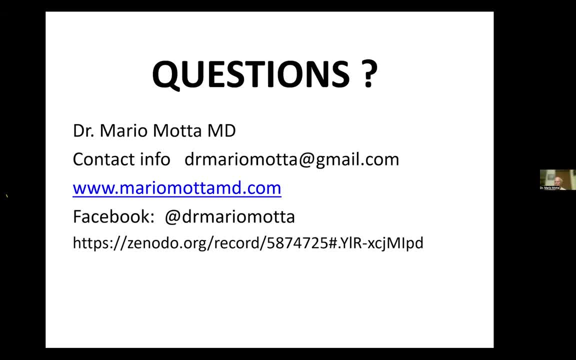 Okay, Debbie Moran had the first question in the chat. Debbie, do you want to come off of mute and ask your question? Sure, if I can remember which question that was, I think that was about that. I do remember. Okay, so Steve Goldberg and I've been 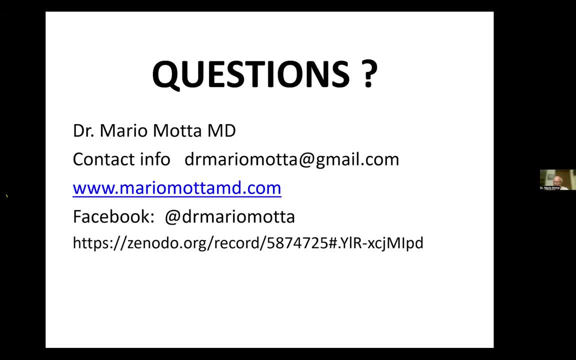 wondering. I've been looking for reading for years now The increases of cancers, mostly colorectal, in young adults, and I thought, well, if it has anything to do with blue light, there should be other cancers that are also coming up. And then just very recently there was a 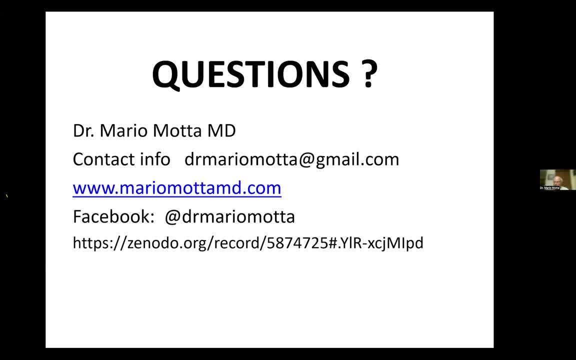 report on a study that said: yes, there were also increases in other cancers. I looked up some of them- uterine and pancreatic, by the way- And there's one- I have no idea why- it says cancer of the appendix and I couldn't find anything about that. but 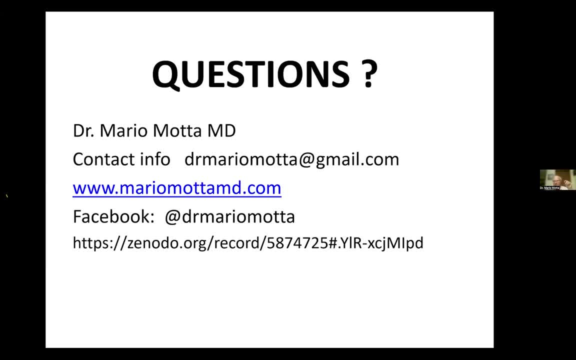 several of the cancer Is has endocrine cells in them. because it makes hormones and basically any hormone related organ seems to be affected. But go ahead, Yeah. so the question is, is every all the articles I read say there may be some unknown environmental factor and not one of them mentions blue light is even 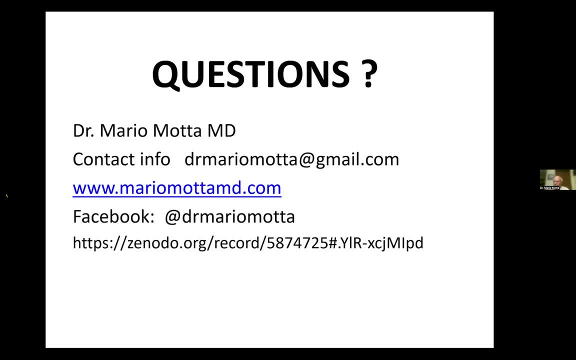 being looked at? Is any? is that even a possibility, and is anyone looking into that? This has been five or six years, they say. now they're looking at the gut biome, but nobody mentions light. The evidence for colorectal cancer is not as strong. There are several papers. 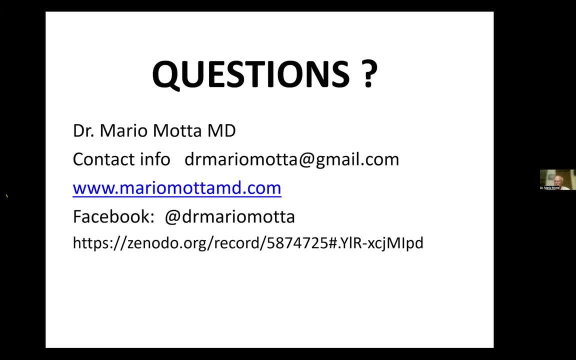 that are very suggestive, but the it's not as robust as the evidence for breast cancer and prostate cancer especially Those two have literally hundreds and hundreds of papers, so there's really no question about those. Thyroid and pancreatic cancer is now getting more firmly established, I believe. 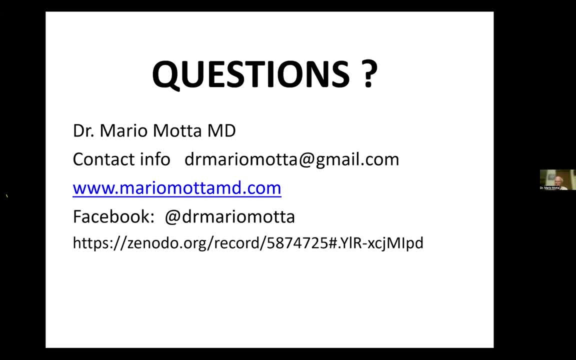 colorectal cancer, and it makes sense because it has endocrine cells, but it's just not as robust. People are now researching that. There will be papers coming out over the next five to eight years. Thank you All right. thank you so much for that. 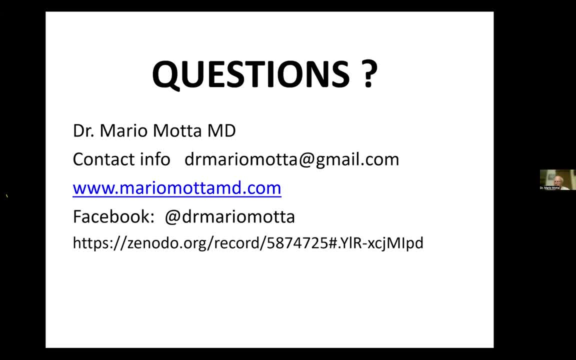 question. By the way, I want to give a shout out to Debra. She is a tireless advocate and I appreciate all your advocacy. No doubt we are certainly lucky to have her in our community. It just it may seem like there's not a lot of progress being made in Houston, but 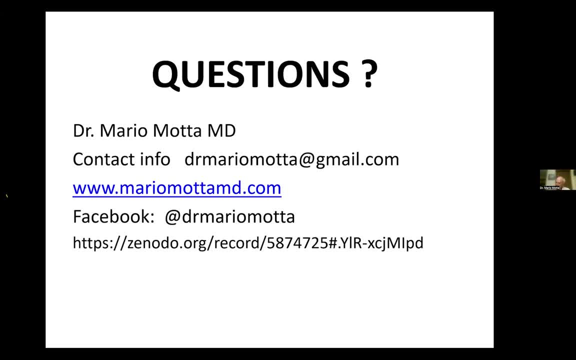 whatever progress is being made. Debbie's had a hand at a lot of that, so we do thank her for that. It's right. The best thing is we can use Houston as a cautionary tale, like we did in Sydney. It's very helpful that way. The canary in the coal mine right. 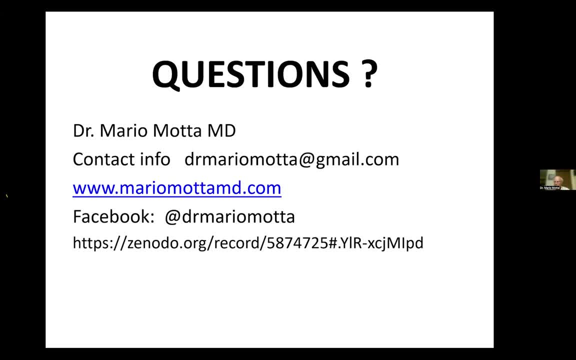 All right, Don Selle had the next question. Don, do you want to come off of mute and ask your question? Sure, thank you very much, Dr Mata. The way things typically work is cost savings, etc. We see cost savings due to the lower. 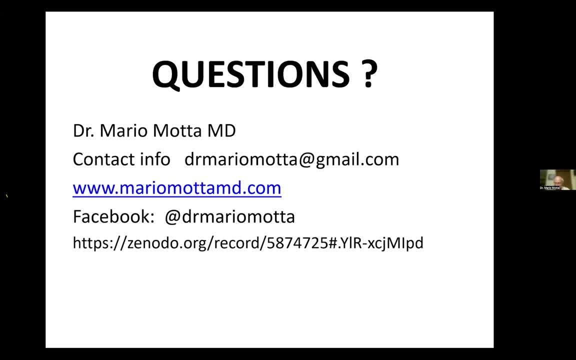 energy use. However, we're seeing more lights. I want to talk about real, really quickly, the glare impairment. Have we seen any lawsuits over that? Because savings from lawsuits is usually a big driver on getting things to change. There are some attorneys that specialize in lawsuits. 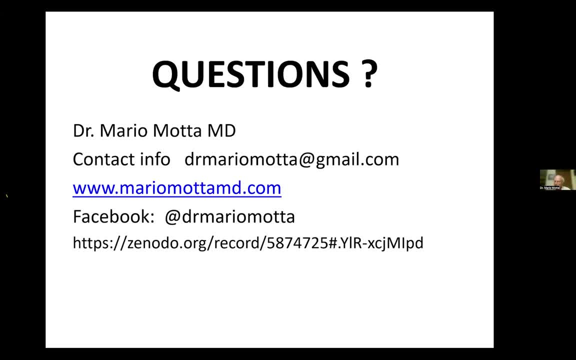 I don't like dealing with attorneys, so I don't want to get them all with that. but yes, and there are attorneys that will claim it both ways. Well, there was no light at this intersection, so that's the reason there was an accident, and others that will say, well, there was. 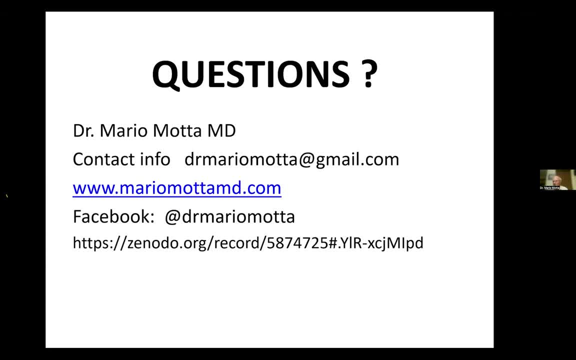 too much glare because there was a light. That's why there was an accident. They'll play it both sides, as most lawyers will, but the the net result is unshielded lights cause glare, Glare causes accidents. That's unquestionable based on multiple studies. 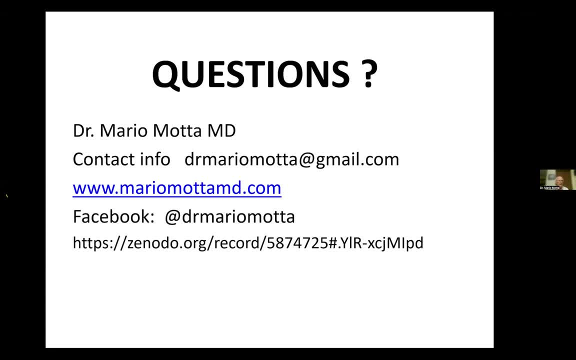 And so- and here's this, and you mentioned the economics- It doesn't cost any more to make a well-designed light as opposed to a poorly designed light. The shielding is pennies to add to material added to the light, So you might as well get the light. 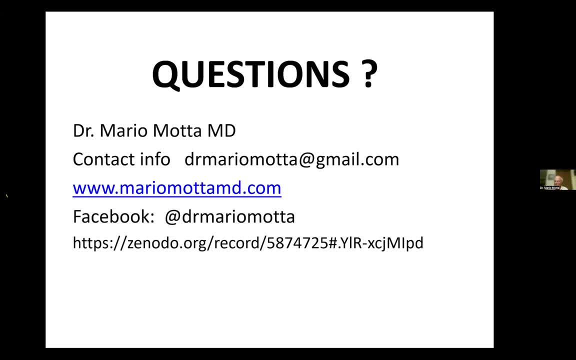 that doesn't cause accidents and doesn't ruin our environment. And the cost of a blue rich LED is no different nowadays than a 2,400 or 2,700 LED, So cost is completely irrelevant these days. okay, That should not be a factor. 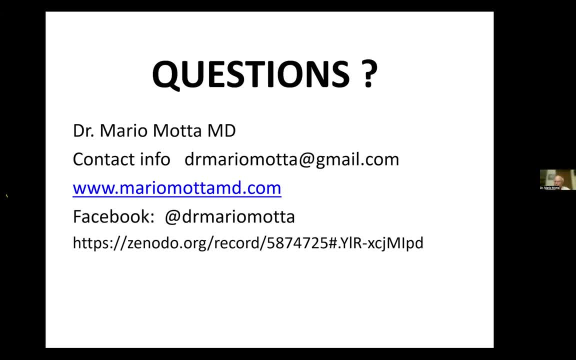 Thank you very much, Dr Mata. Thanks for the question, Don. All right, the next one was Hannah Power. I hope I'm pronouncing your last name correctly, Power. Hannah, you had a question about advocacy and what we can do to work towards correcting this problem. 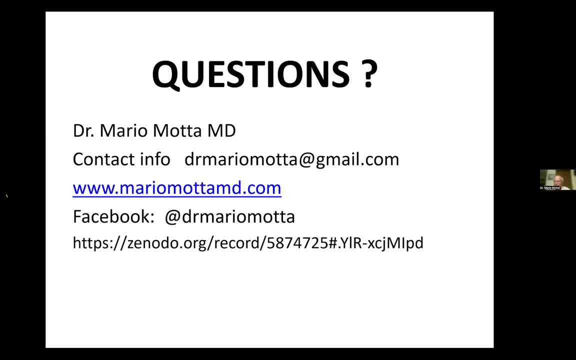 If you wanna come off of mute and ask your question of Dr Mata, please feel free to do so. Hannah, I don't know if you're there, but if you're not gonna come off of mute, I can ask the question for you. 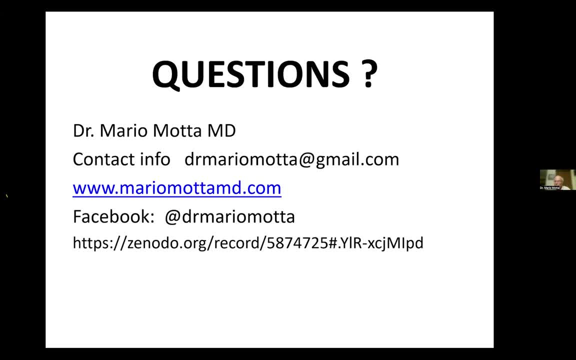 She'd asked: what work can individuals do to work towards limiting light pollution. Are there any activist organizations you recommend for someone interested in becoming involved? Do you believe meaningful change is even possible in America? Well, if you live near Houston, call Deborah. 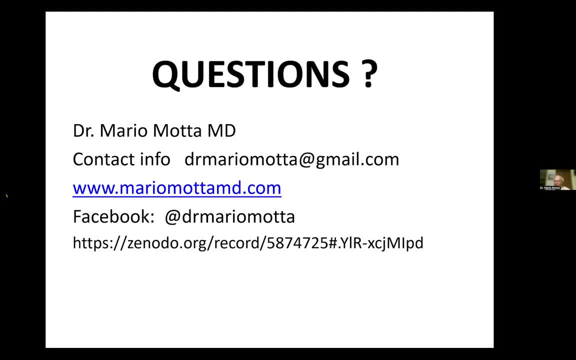 but you can join the IDA And that's a worldwide organization. I'm a past board member of the IDA and currently member of the IDA in Massachusetts And they do fabulous work. It's volunteer. they asked for $35,. 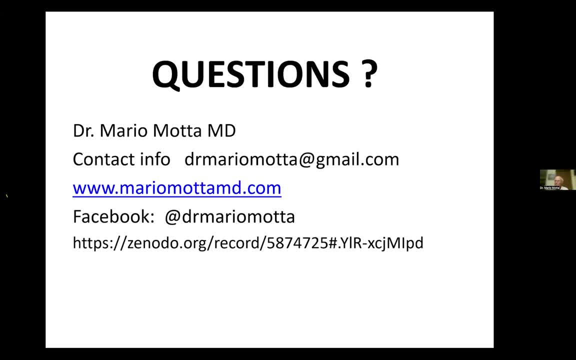 but it's basically a donation. but that'll give you plenty of information that you need to go to a local city council. And the second thing is basically my wishlist is that every city or town has at least one activist that will go to city council meetings. 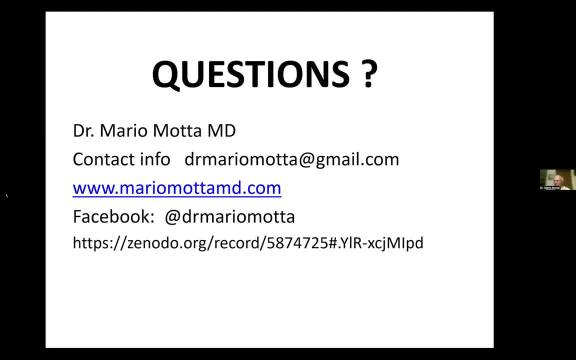 If we did that, this problem could be solved easily, because most city council members don't know anything about lighting. So they basically ask the lighting company. and the lighting company- surprise, surprise- best interest is to increase their profits, not to give you the best lighting. 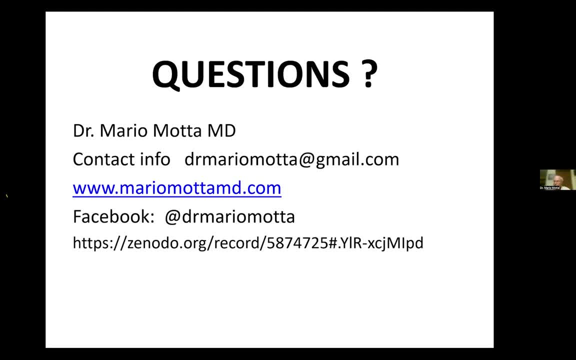 Okay, thank you for that. Dr Hsiao wanted to mention something before she had to drop. Dr Hsiao, the floor is yours. Please feel free to make the comments that you wish to make. Sure, just very quickly. 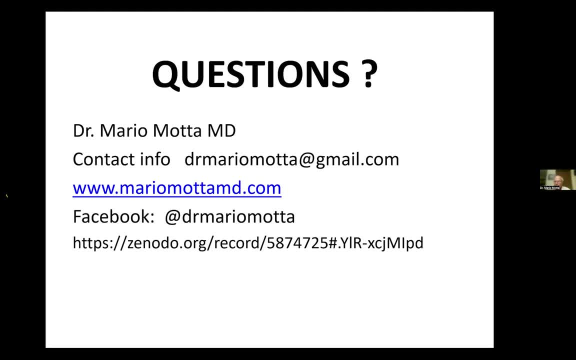 Thank you so much for this very comprehensive talk. It's beautiful. I just want to mention one thing: that, as I said in the comment, I believe light pollution is not just the public health hazard but also an environmental justice issue. So there have been some papers. 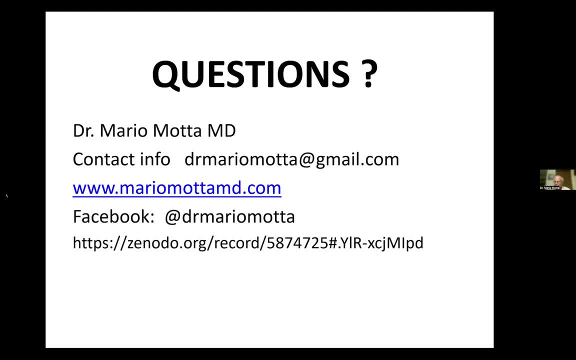 including one paper that we published that showed it's really the more disadvantaged communities and racial and ethnic minority populations that show their higher levels of light pollution. So you know, I just want to make that comment- And also those happen to be the people. 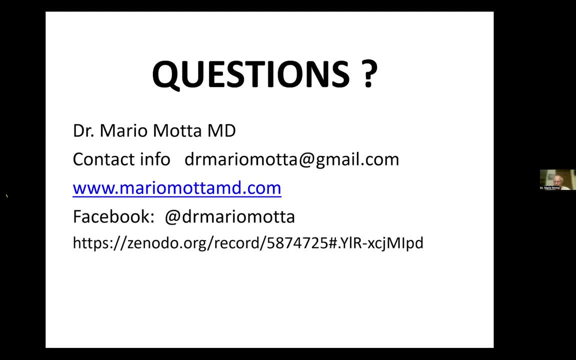 that has the least means to buffer the adverse effects. They don't have blackout curtains, they have to work night shift work and therefore they're more exposed to light as well. So just thank you again up to around now, but just want to make that comment. 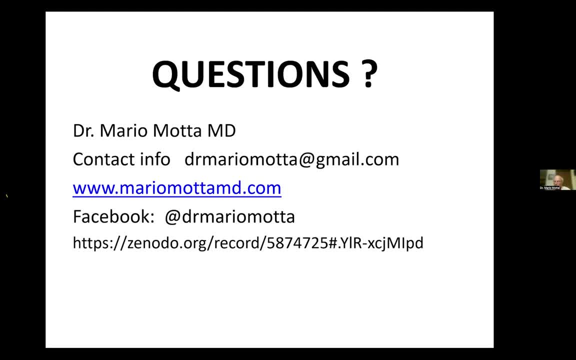 Thank you, I appreciate your papers. Thank you, Dr Hsiao. Thank you for sharing those links. For those of you who are still on, those are in the meeting chat. If you'd like, you can go ahead and click on those URLs directly. 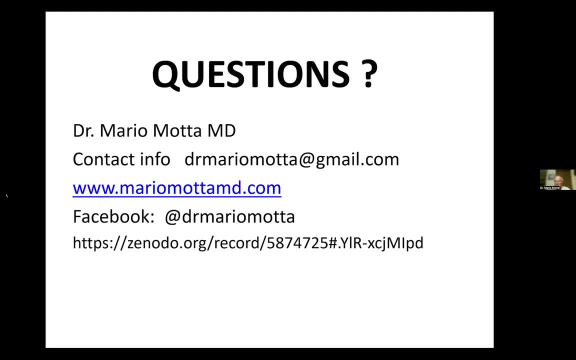 That'll take you to those, those links that Dr Hsiao had mentioned. Okay, we had a question from Vanita Fuller. Vanita, do you want to come off of mute and ask your question? Yes, I think you answered part of this. 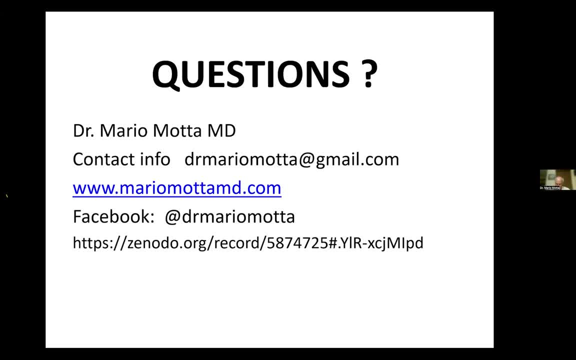 after I made the input. the question: I think you answered it with your studies on the rats, But could you explain the difference between dark and those gradations as the cancer risk went up? I mean, it's not like if you fall asleep with television on at night, is that a risk? 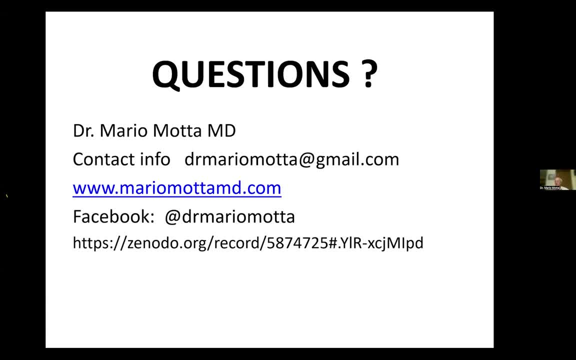 Yes, it is, unfortunately, but there is no dimming of blue on TVs at night. So basically, when you're looking at your screen up until sleep, normally your melatonin starts to rise when it's dark. So if you keep your lights on, 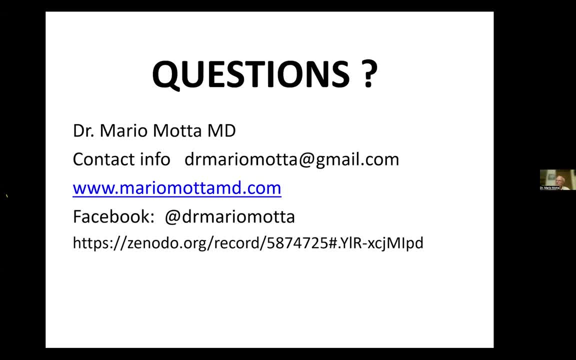 your melatonin is suppressed until you start turning off the lights. But the TV especially has high intensity blue light, especially LED, The LED TVs. So consequently that's especially harmful. And if you, instead of taking a sleeping pill, basically turn off the TV, 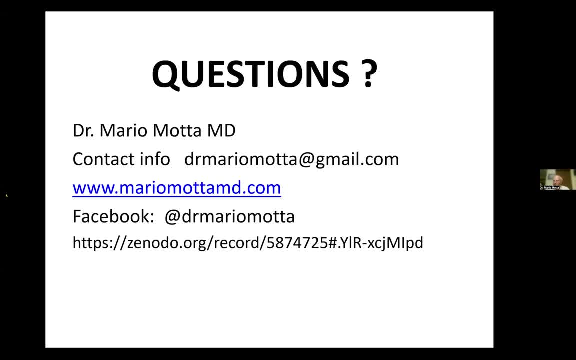 read a book under a yellow light for a half hour 45 minutes, go to bed And by the time you're ready to go to bed, your melatonin is starting to rise and you'll fall asleep much easier. People think it's that they're falling asleep. 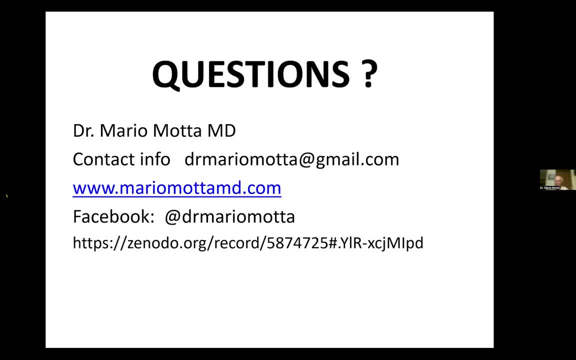 because they're reading a book and maybe they're getting bored, But it's not. It's because you're no longer suppressing your melatonin. Once the melatonin starts to rise, you get sleepy, So let nature put you to sleep instead of pills. 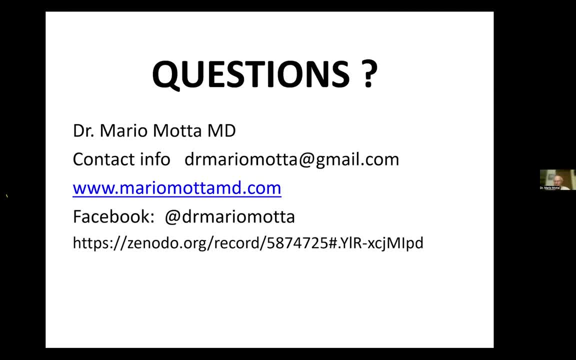 I tell that to my patients all the time. Thank you for that question, Vanita. And speaking of pills, Bob Gillespie had the next question. Bob, do you want to come off of mute and ask your question? The discussion has talked about melatonin. 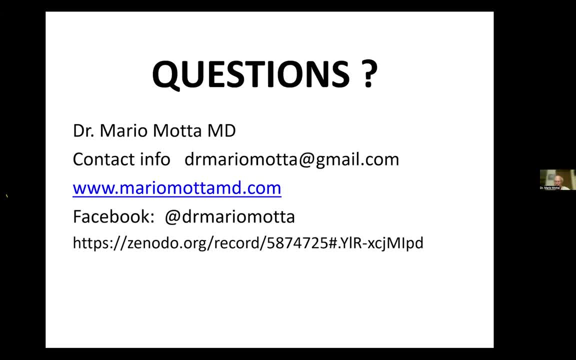 Melatonin quite a bit, And so an obvious question would be over-the-counter melatonin pills, things like that? I would assume they do nothing to help. Yeah, So melatonin certainly helps you if you're suffering from jet lag and changing zones. 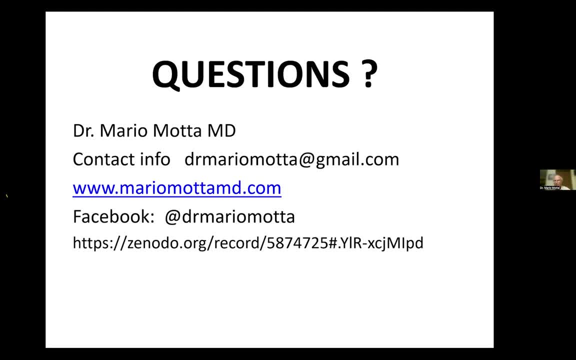 We all know that and it'll help you fall asleep. There was one study- in fact I included it in this talk- that showed that it improves the ability to, when you're getting chemotherapy, to fight. it improves the effectiveness of the chemotherapy. 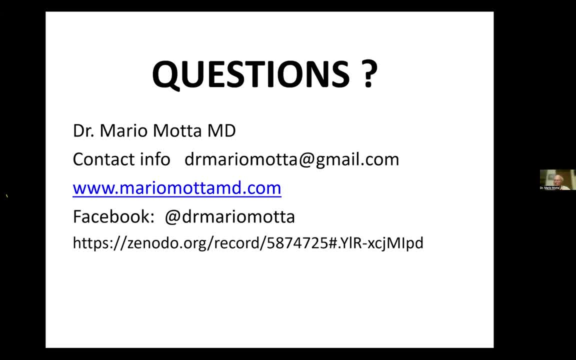 that take in melatonin. But there aren't many studies on this yet so it's not very much well-known. And there are other studies where people have taken extra melatonin and it doesn't seem to cut the risk of uh of cancers. uh, at least these were early studies 10 years ago. they haven't been. 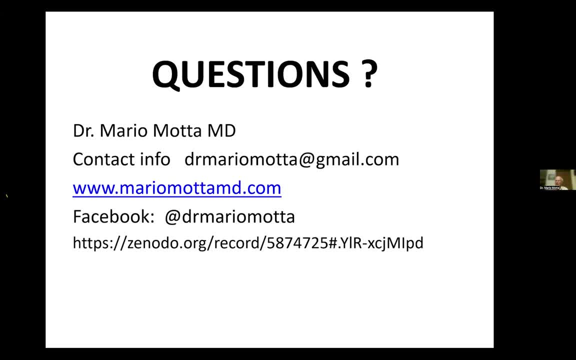 repeated uh. so it's kind of a mixed bag. i can't say if you take melatonin you're better protected. but what's incontrovertible is if you allow your natural melatonin to to flower at night, you are better protected. whether taking pills protects you or not is not robust enough studies to say that. 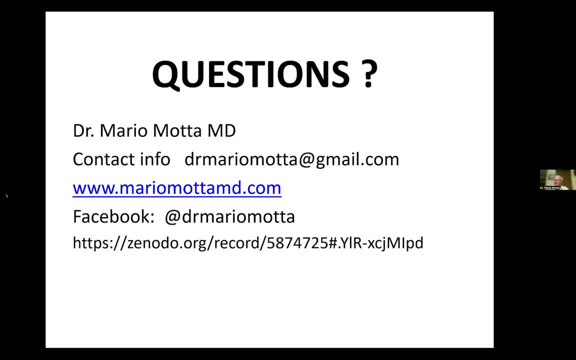 but i did show one study where it does improve the effectiveness of chemotherapy. all right, thanks for the question, bob dr mata, two more questions, is that okay? is that? uh, as long as you want, i'm fine, thank you, uh. the next question was from bill spaziri. uh, our good friend bill. 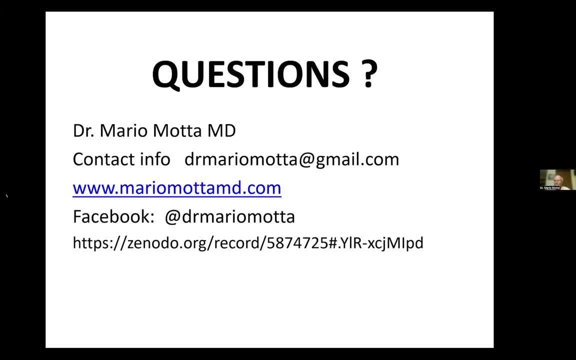 uh, bill, do you want to come off of you and ask your question? well, um, i think that was a long time ago, i i think i didn't have a question. i had a comment, um, which was extremely significant to me. it was in the form of a question, though. 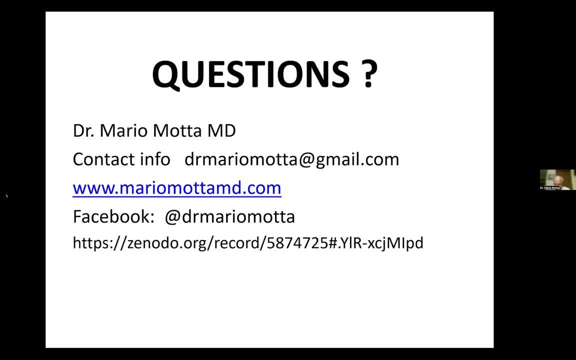 well, so, uh, okay, perhaps i hope we're talking about the same thing. uh, many years ago, many years ago, i was a believer in helping dark skies, but i thought that the i was listening to the advocates and they seemed like fanatics to me. please don't take this in any way. that's what it seems like to me. and uh, then one of those people- 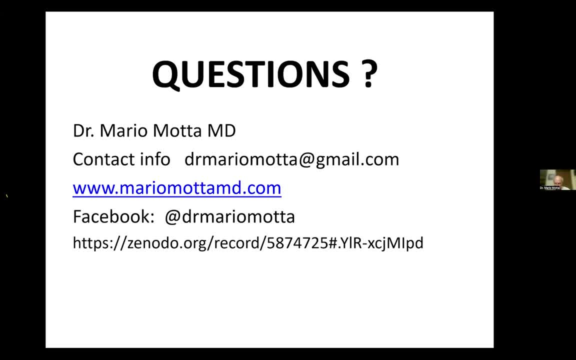 took me outside and i was like: oh, my god, i'm going to die, i'm going to die, i'm going to die, and showed me the proper temperature lights right next to the, the bright blue and white lights right next to each other, and i just hallelujah, i became a believer instantaneously when you see them right. 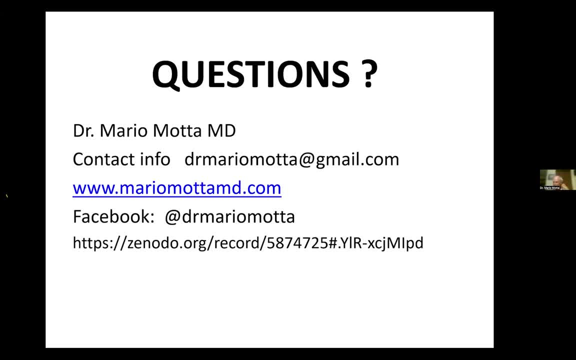 next to each other. the difference is striking. the problem is obvious. i even went to the houston city council and tried to tell them that, but you know what? are they going to listen to me? but when you see them right next to each other, you can make a believer out of somebody is what? 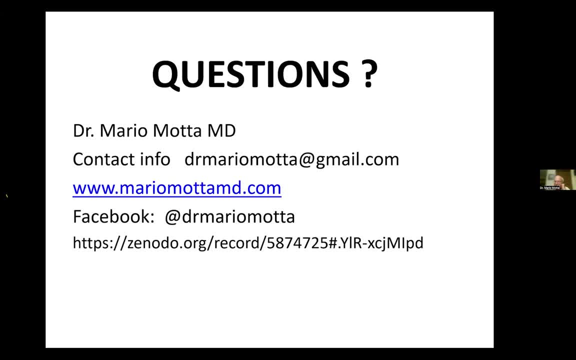 i'm trying to say: and uh, that's so obviously. you know, i understand what you're saying, i agree with you completely. but that was, i thought, a good way to make people understand. that's it. so i absolutely agree with you and the um. two things that. two quick comments on what you've said. first of all, in gloucester, 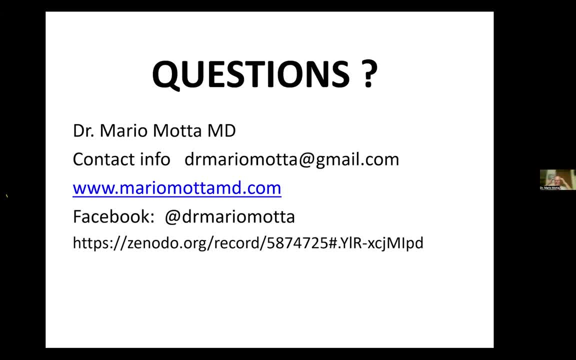 it was hard to convince the city council because people just intuitively know, even though they have no studies to back this up, that the brighter the light, the better. it is right. that's what people think. that's why people light up their houses like crazy. so what they finally? 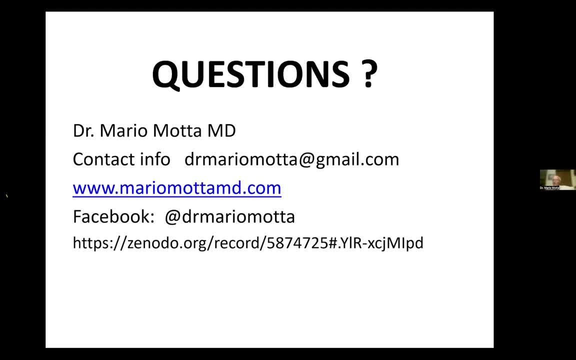 agreed to. okay, we'll do a study, we'll put up four lights- uh of uh, what did they? 4 000 k and four lights of 3 000 k, and they did that along the street near the center of town and they they published it and said: please vote, uh, for when we replace our lights, which one you like they got. 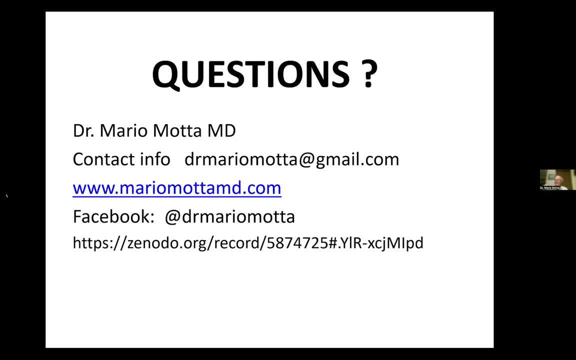 something like 230 votes. everyone voted for the the 3 000 k. no one wanted the 4 000 k and the reason is, once you're exposed to- i mean, it's a number- 4 000 k, 3 000 k- what's the difference? once you see it, you realize how. 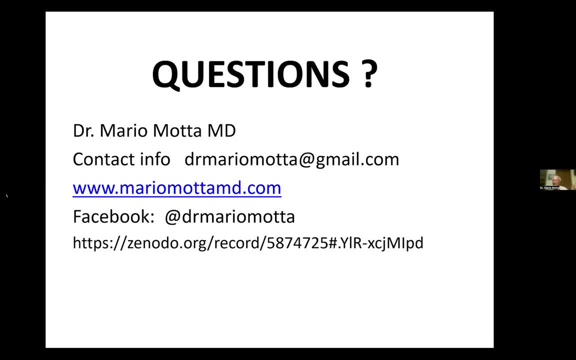 bad, it is okay, and that's why seattle is taking down, you know, all of their lights right now, as we speak. it's a five-year project and the reason they're doing it is because the city people hate it. so, consequently, the city people hate it and they're not going to vote for the 3 000 k. 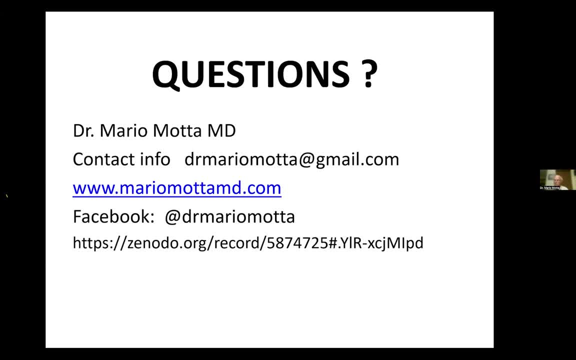 the thing to do if you have a reluctant city council is say: do this experiment, why don't you put up a few three 2 700 lights, a few 4 000 k lights and let the townspeople vote? that's what convinced people in town here where i live and, uh, it was unanimous at the city council once the 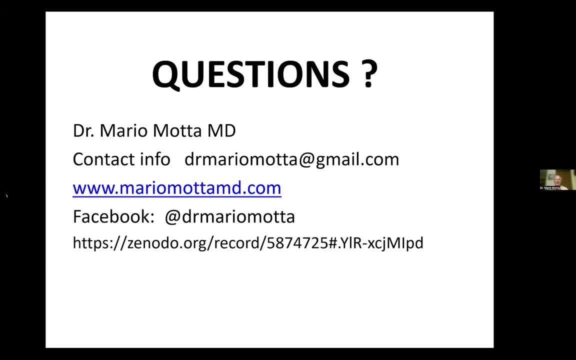 votes came in. and the second thing you said about fanatics. yes, sometimes people can be fanatics. i never tell people you have to shut off all your lights because immediately you'll get a turn on. what i say is: use light appropriately, don't place it where you don't need it. don't interfere in your. 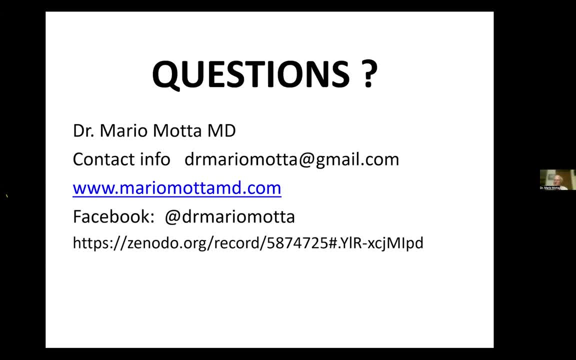 neighbor's lights and shield lights, so it doesn't cause environmental harm. that i think everyone can agree to, and once you put it in those terms, you don't come across as a fanatic and you win people over. all right, joe, i think i found what you might be referring to as my question. my question was: 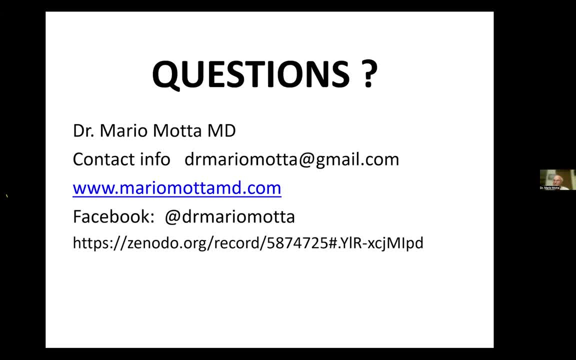 do the cell phone and computer companies have any comments on all this? that was the question. okay, the um cell phones- the iphone i have dims automatically at 9 pm, gets rid of all the blue, and that was bait. and apple specifically stated because of the 2012 ama paper. so that's, you can. 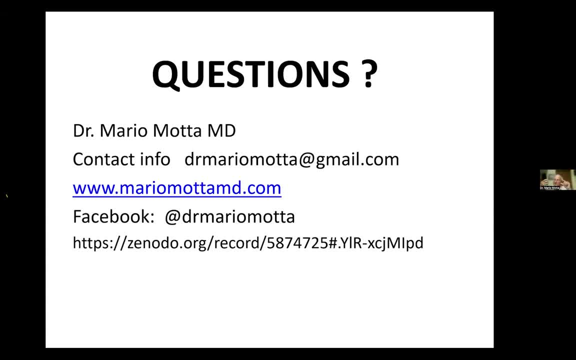 override it if you want, but it the uh. basically it shuts down all the blue and you can use it all night long, but without blue. all the other most of the phones now do that. most computers do that, not all. but there are things you can download to dim your computer and get rid of. 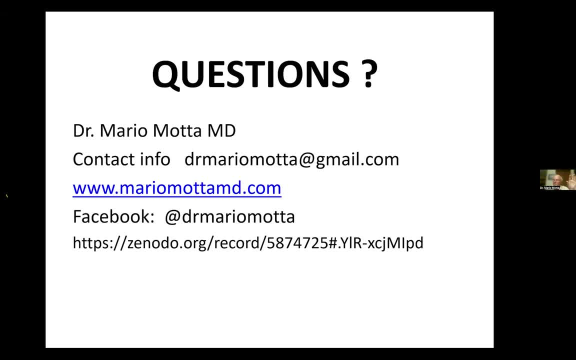 blue tvs are a whole nother matter. they have intense blue and that's why you should shut them off an hour before you want to go to bed. all right, thanks, bill. um, all right, last question from predict: predict. do you want to come off of mute and ask your question? 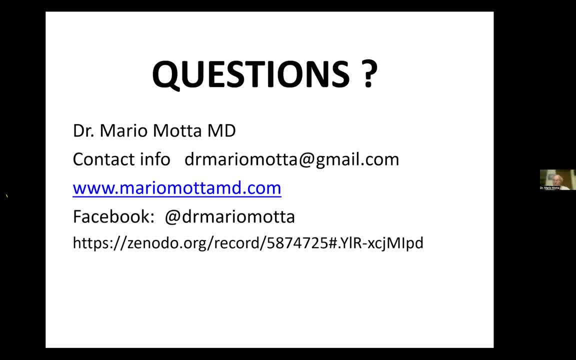 okay, no mike, that's right. all right, i asked one quick question, just very quick. well, let's get to predict's question first. and i don't. is that joe? yeah, that was joe donald. well, he popped up and said: no mike. so i thought: okay, yeah, no worries, we'll get to his question because he did ask it, and then we'll give the. 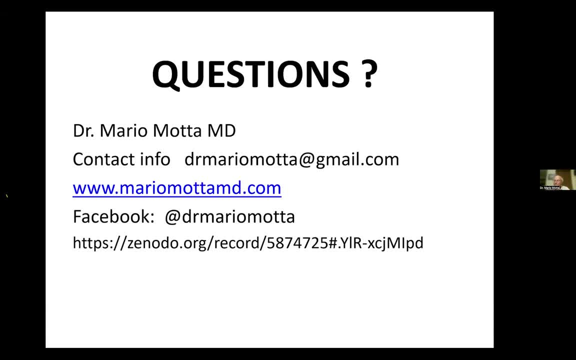 last question to you, if that's okay. so predict's question was: do blue light blockers work and are they recommended? the initial section of your presentation seems to provide a solid argument in favor of their utility. said, i've previously been skeptical of them as merely a marketing. 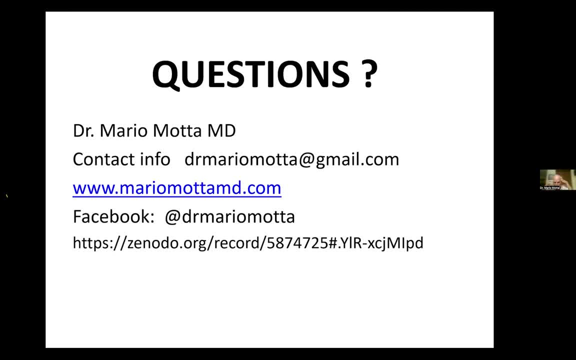 spiel or gimmick. you're talking about the blue light blocker. the blue light blocker, the blue light, i imagine the high glasses that are blue blockers, i believe. so, yeah, and the answer is yes, they work, uh. so you, um, in fact, i've got a pair. a company sent them to me after i gave a talk, uh, and they 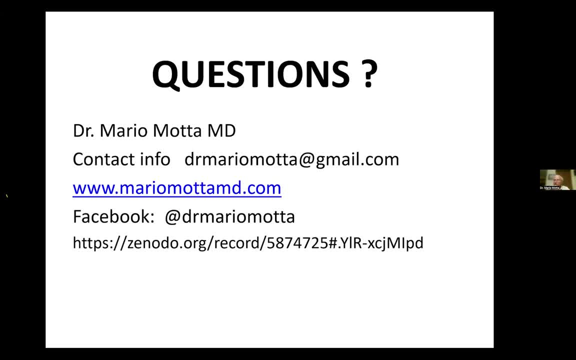 seem to to work. it helps me dark adapt a little faster. it's not the uh be all, end all, but it does block blue. and if you want to wear them at night to block your tv, that that might work, although i see no study on that. but it's not the uh be all, end all, but it does block blue. and if you want to. 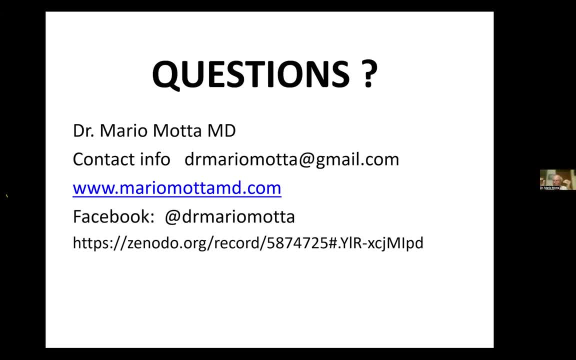 that, so i can't recommend it. the only thing i will ever recommend is something that's proven with a study. but it makes sense that if you block the blue from a tv light, a tv screen, you have less of an effect later at night. so that's the only way i can answer it, based on some common sense. 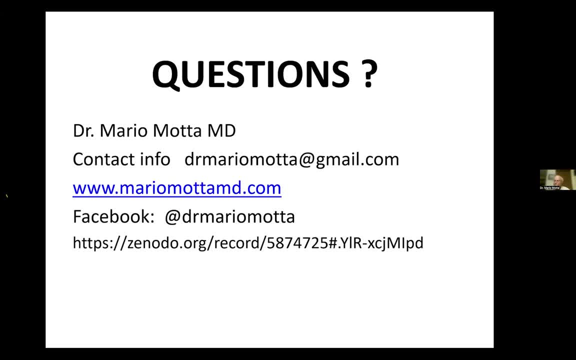 great, thank you for that. and then, uh, joe, we'll go ahead and get your question as the last one. okay, i was just going to say if you had any other good ideas for how to convince people, because i was going to make one comment. we we tried to get a lot of people to answer that question, but i 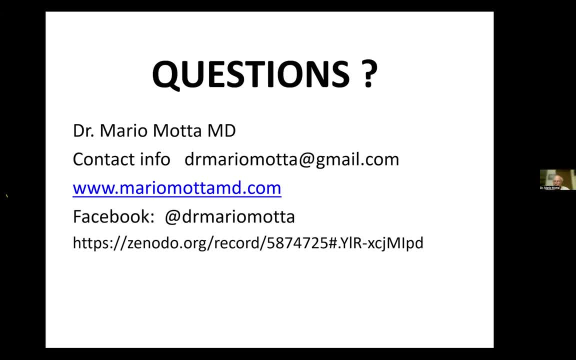 was going to make one comment. we we tried to get a lot of people to answer that question, but i pollution ordinance around the george observatory and we succeeded for about 15 years and then the state legislature canceled it again, so we eventually lost. but uh, we've talked a lot to. 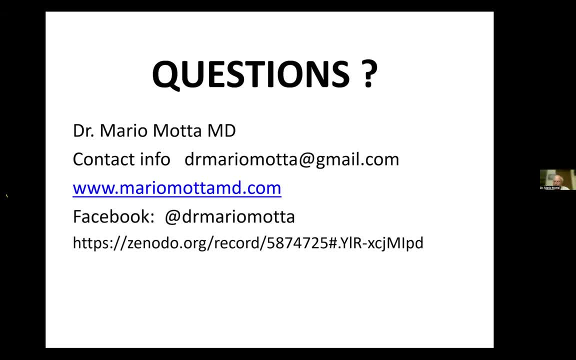 city councils and such, and what we found was: uh, the winning argument was to switch the argument to be about light trespass. uh, that, what we found is people in rural areas. if you you tried to say we want a light pollution ordinance out in the countryside, they got mad. i want to be able to. 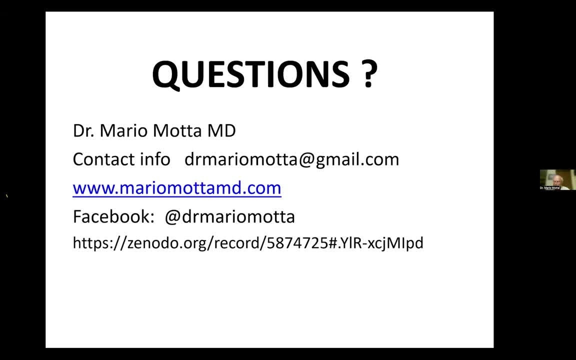 do whatever i want, but if the conversation flipped to we want an ordinance against light trespass, then everybody loved it. so i don't know, is there like a collection anywhere of like all the good strategies for how to give good arguments? well, there are political realities, i mean in 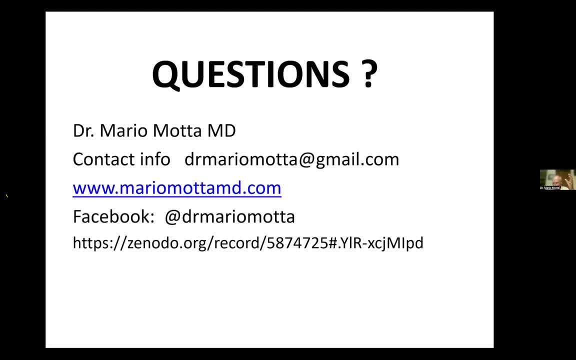 gloucester, um, and i've worked on many others. some some are stricter than others. connecticut has some of the strictness, like pollution laws, uh, and that's due to a uh, several people who i know down there, but, um, it's, you're not. it's hard to get a lot passed. 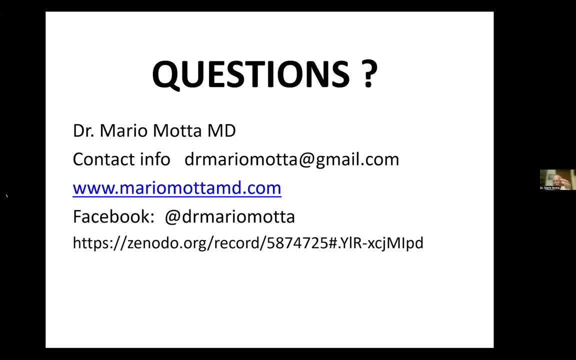 for private homes. it's very, very difficult to do that. so in gloucester, uh, the ordinance we have. this covers all streetlights, businesses and multi-family homes. so if you have two or more families, you're covered because you're renting out and you're basically listed as a business. 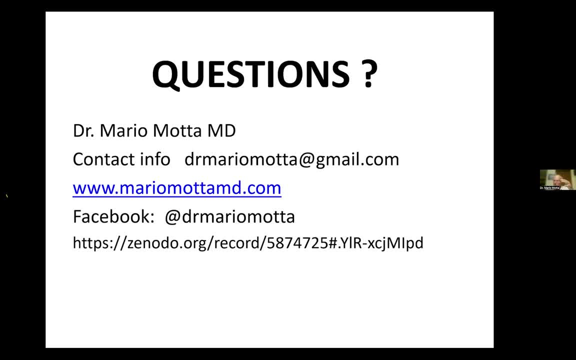 uh and it's been helpful because all developments since then tends to uh follow the bylaw. it's it's enforced at the uh when you have to put in your building plan and then your lighting plan, uh. so because it's really hard to fix things after the fact. so but in other places it's weaker or stronger. connecticut does cover. 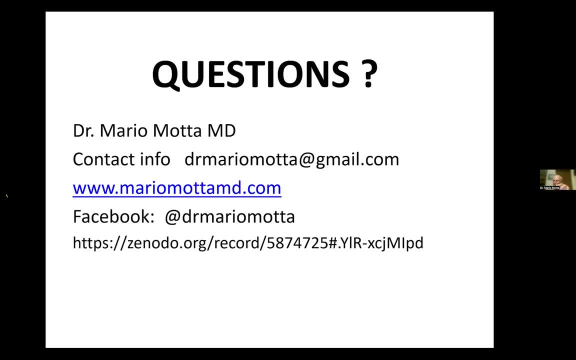 it's the only state that i know of covers private homes. but you are absolutely correct. nuisance, uh, issues such as someone shining a spot on a building and then you have to put in your building plan spotlight directly into your bedroom window. you can complain about that, uh. and if there isn't an 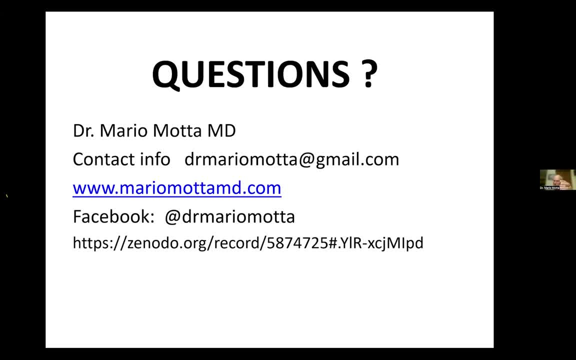 ordinance and just by nuisance laws you may get that addressed. generally the best way is to speak to that neighbor. if they don't want to listen then unfortunately you've got to complain elsewhere. but most people are reasonable. some people are not. the problem in many locales is people just. 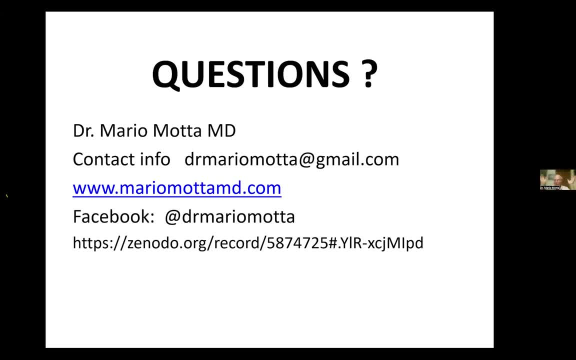 quote: know that, uh, that if they put up lights, that, uh, this will help them prevent crime. we won't get broken into. yet, study after study after study- the best one i found i should have included that one- is: you go to study people to ask people in jail for burglaries: why did you pick these houses? and invariably, the answer is: 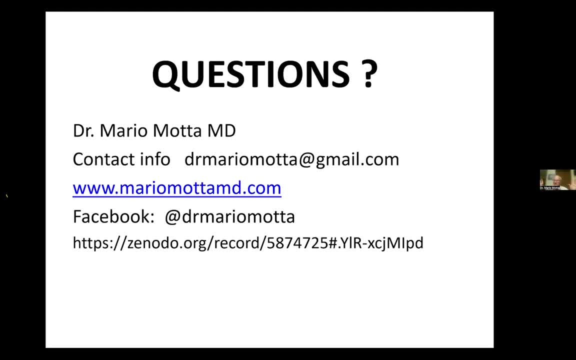 it was brightly lit and they're basically saying- i'm paraphrasing here- they're basically saying: i'm afraid of you and i get a lot of expensive things in my house and i'm trying to scare you away. okay, so they pick the houses that look like they're rich and all lit up, because those are exactly the houses that they want to. 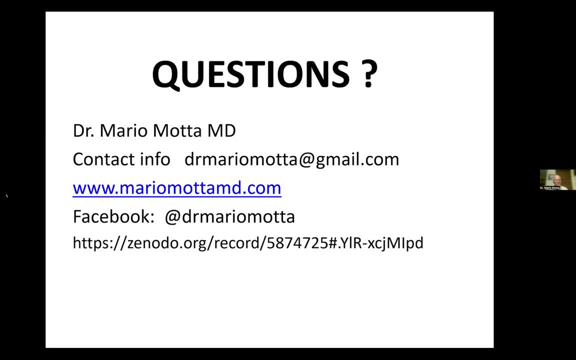 hit and the houses that tend not to be lit up don't get hit as hard or as much or as often, and that's a well-known fact. that's a new one, thank you. okay, that's a good one. i love it. appreciate that. yeah, and just uh, anecdotally, the the night that, uh, they put the of the day that. 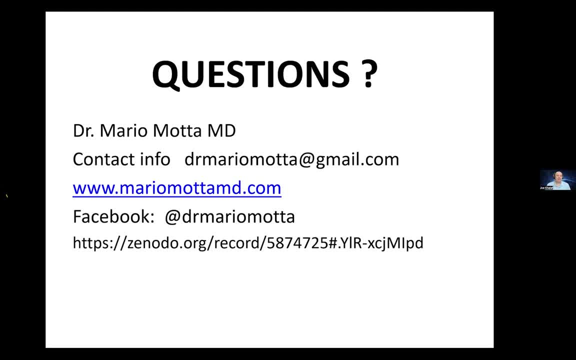 they put new leds on the house. they put new leds on the house. they put new leds on the house lights on my street. uh, my neighbor had parked his jeep right under that bright new led light and, uh, his, his jeep was broken into that very night. well, i just gave you a study on that from england. 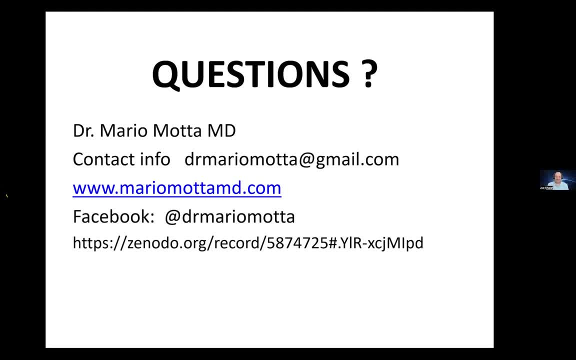 that showed that, yeah, basically, uh increased, uh, break-ins in into cars absolutely. comment: i know we have a little time, but but um, i'll come, i have that slide. and then, conversely, and woodside, where we have shielded light, we have a video of someone breaking off a. 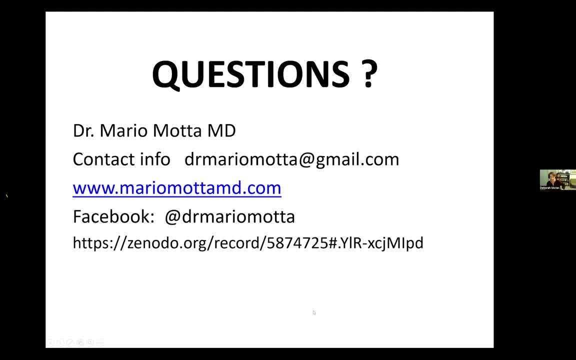 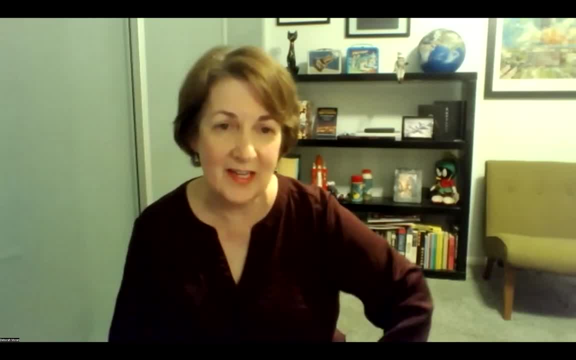 car burglary when a when a light came on, we had some dude light there, but um, i just want to let the membership know that i really think the root cause of light pollution is uneducated police forces and having only environmentalists do this measure, this message, instead of the police talking. 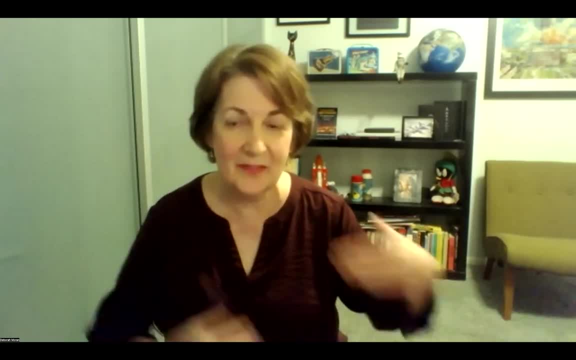 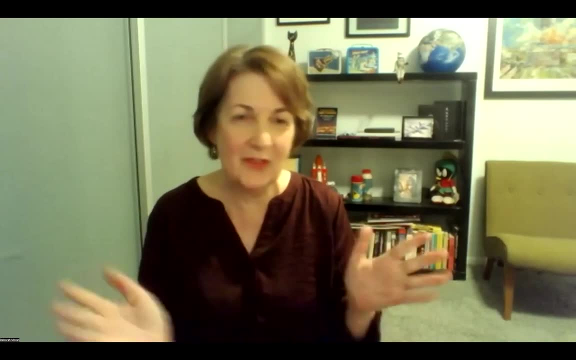